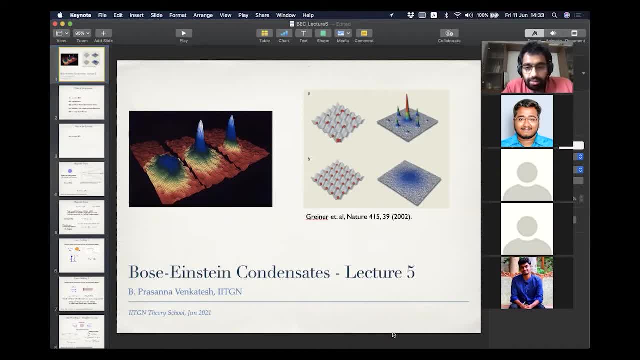 OK, so let me get my annotator. Why can't I see my annotations? OK, so let me get my annotator. Why can't I see my annotations? Wait, Can you all see my pointer? Can someone confirm that you can see my pointer? 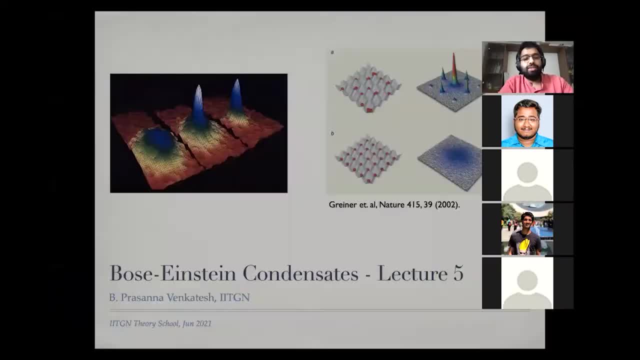 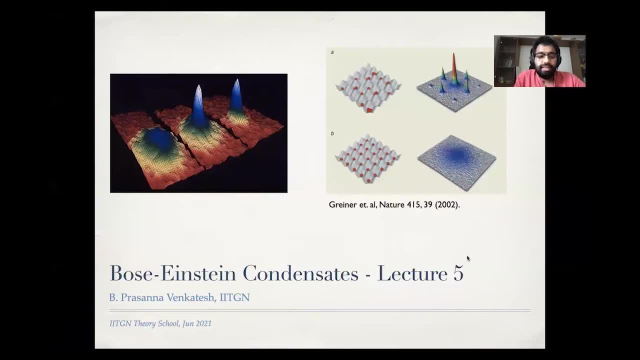 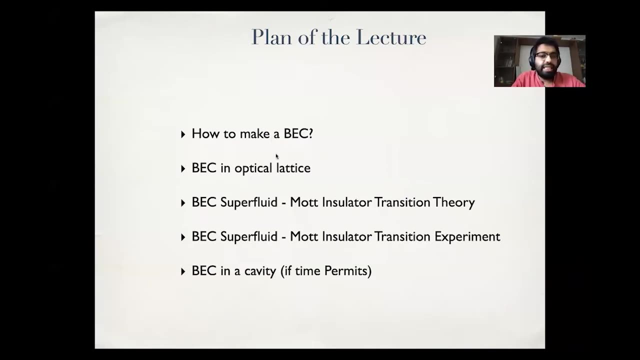 Yes, sir, OK, fantastic, All right, So here we go. So let me make this smaller. Welcome to the fifth lecture of this series. And so what are we going to talk about today? OK, so one thing I realized is, basically, I never told you in detail how one goes about making a Bose-Einstein condensate. 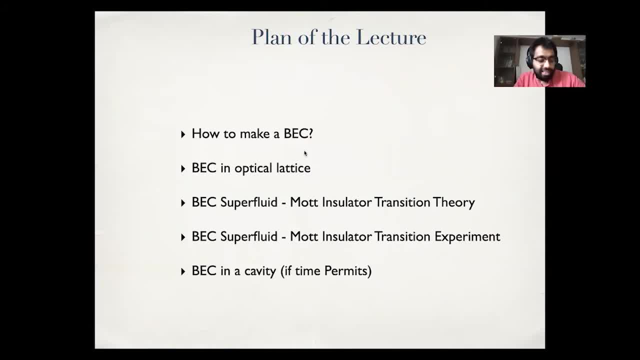 We've been talking a lot about the theoretical description of how to you know, how to understand what a Bose-Einstein condensate is, and so on, But I've not really talked about how to make it. So I will begin with a brief overview of how, which is 20,, 30 years of research. 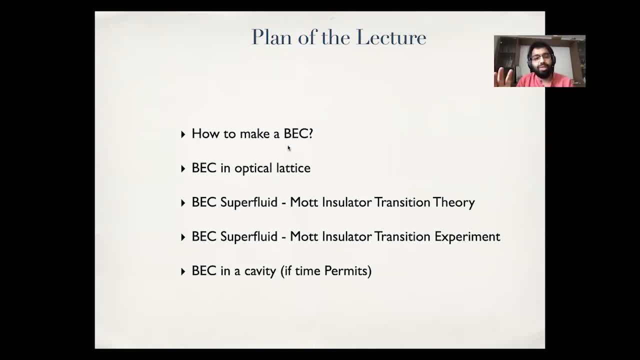 But I will make a very brief overview of how to make a Bose-Einstein condensate: trapping, cooling and so on. Then I will really talk about Bose-Einstein condensates in optical lattices, which are periodic potentials of light in which atoms are placed. 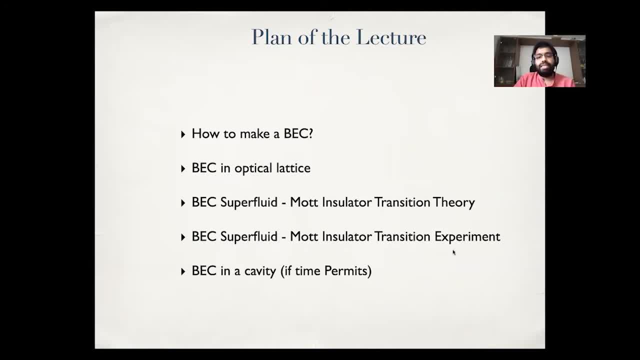 And in this context I'll describe this very famous experiment, a landmark experiment that actually in some sense showed the community the power, the full power of what this Bose-Einstein condensates in optical lattices, or cold atoms in optical lattices. 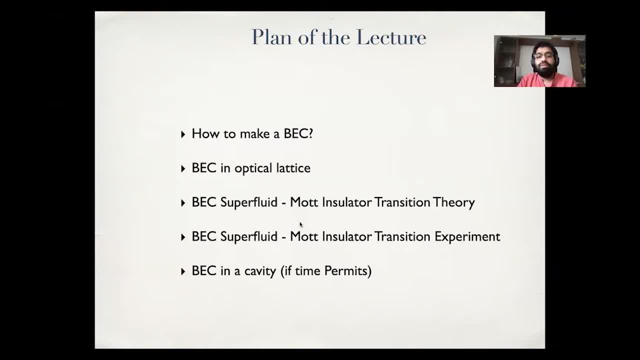 What sort of physics can we address with this very interesting experimental and theoretical? So that's going to be the meat of the talk And then, if time permits, I'll come to the study of Bose-Einstein condensates in a cavity which is, in some sense it's like an optical lattice, but it is alive, in the sense that an optical lattice is an applied static potential of light. 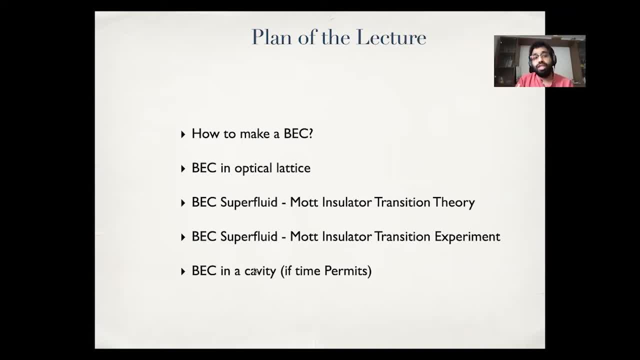 But a cavity is essentially an applied potential that is dynamic, which changes as the atomic state changes. That's the zeroth order description. That's the function of cavity I'm interested in And that is very close again to the sort of things I work on and the things that I am interested in. 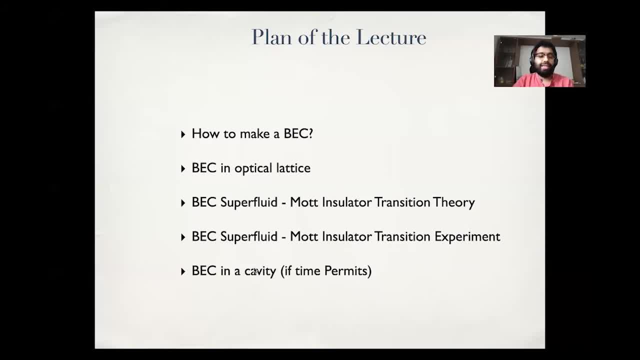 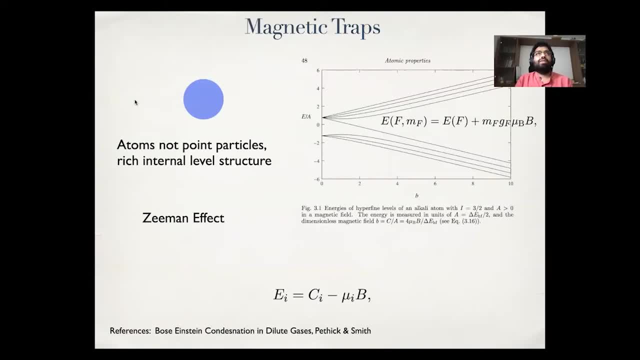 So it might be. from a personal point of view. if I can get there, it would be great, But otherwise it's all right. All right, So let's begin with how to make a Bose-Einstein condensate. Basically, if, from what we learned in the first part of the lecture, in order to make a Bose-Einstein condensate, you want to essentially trap atoms, because that's when the density of the atoms becomes significant- 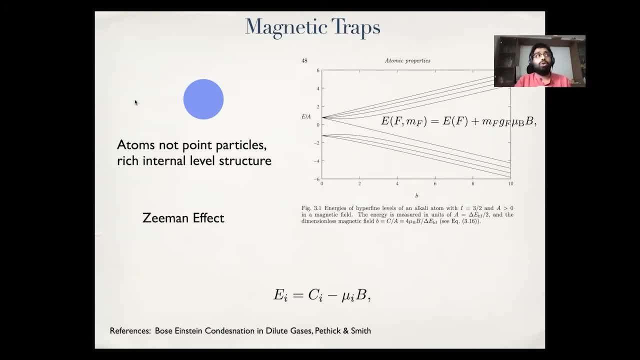 So that the Transition temperature comes lower. at the same time, even when the transition temperature is low, you have to trap and then you have to cool them below the transition temperature. So if you wanted to make a Bose-Einstein condensate with neutral atoms, so to speak, you have to learn how to trap them as well as how to cool them. 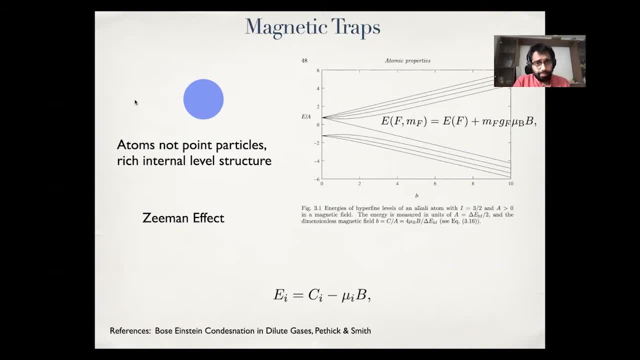 OK, so the zeroth order way to trap atoms is by using magnetic fields, And the fundamental Principle that lies behind it is the fact that atoms are not point particles, right? So the, for example, if you think, the electron in the outermost shell of a sodium atom, an alkali atom or rubidium atom, these, this electron has a rich internal level structure with different, different orbitals and so on. 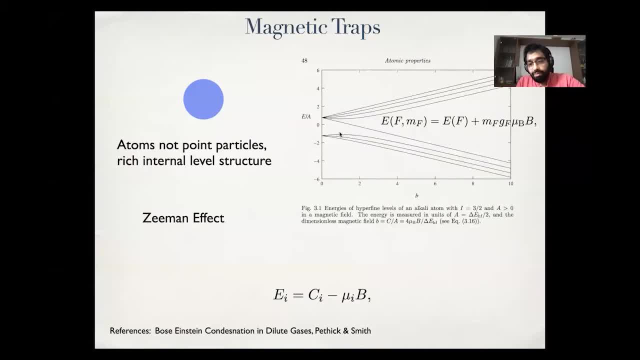 Moreover, very interestingly, once you apply a magnetic field, these energy levels split right And these energy levels can. energies can increase. Some cases, energies can decrease in upright field, and this effect is what is called a Zeeman effect, right, 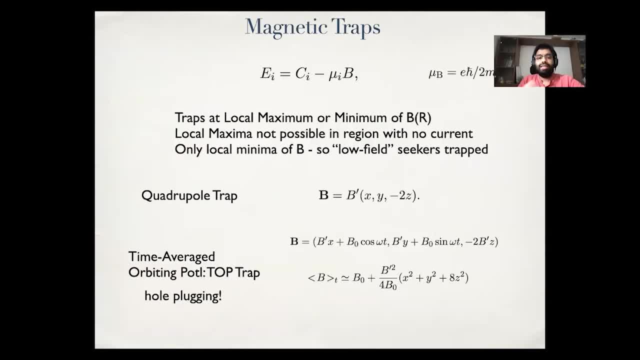 So one can take advantage of the Zeeman effect to make a magnetic trap. The idea is very simple, Basically the changing internal energy of the atoms. once you make the B field position dependent, this essentially becomes like the potential energy for the center of mass of the atom itself. 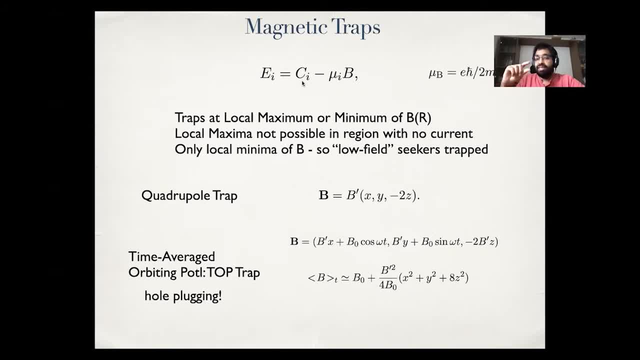 So the electrons Internal energy Level is going to depend on position. As a result of the entire atoms, atoms, potential energies now becomes B of R. OK, so now how do you trap? Of course one can trap at the, at a local maximum or a local minimum of such a magnetic, static, magnetic field. 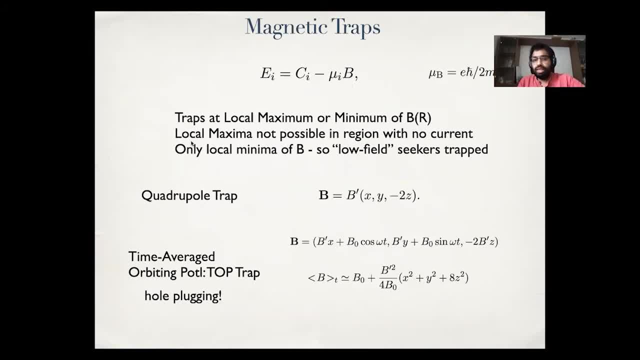 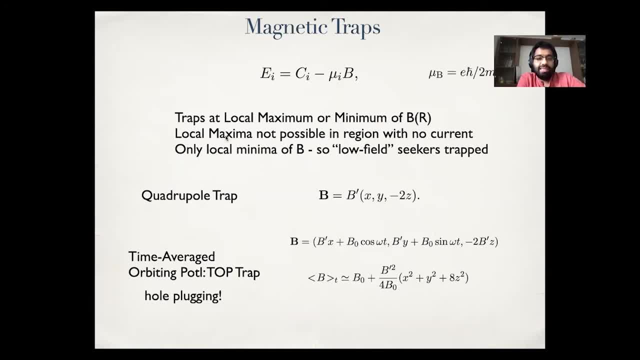 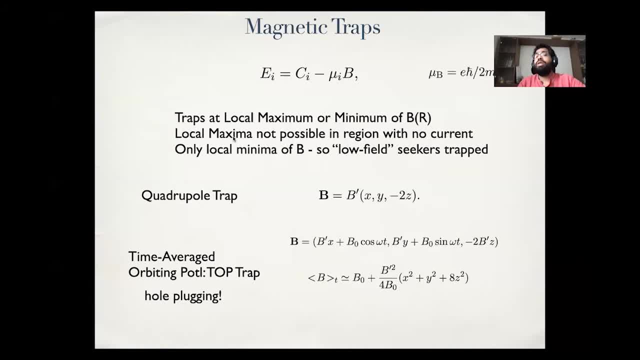 for electric fields that it cannot have maxima. there is actually no extreme, for electric fields is not possible. Similarly, you can show that mac is not possible from magnetic fields, But you can actually make a local minimum, in which case you should only choose items which 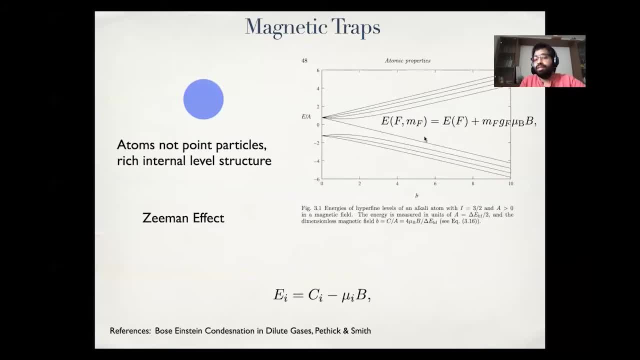 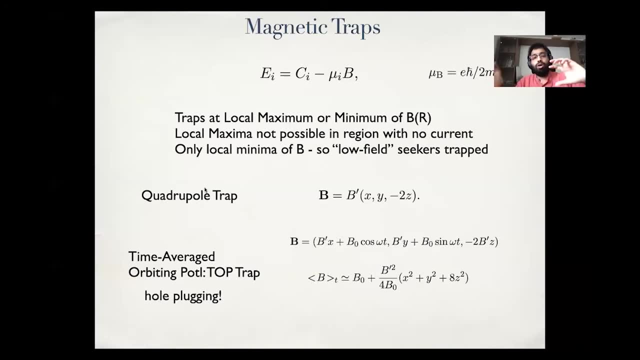 have a low field seeking. so you want to put your items in an internal state such that it seeks lower and lower fields. So this branch, not this branch. You have to then find ways to make configurations of electric currents such that you can realize. 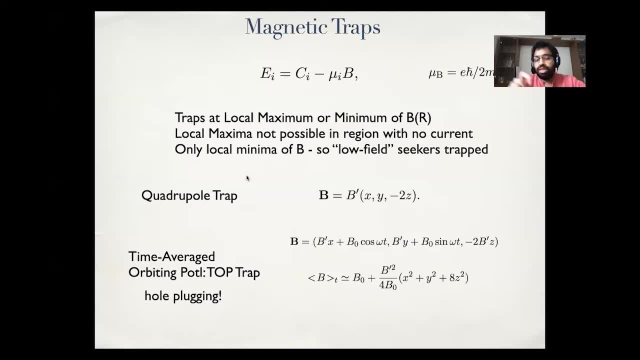 magnetic field configurations with absolute minima or local minima at some point in space, and then you can collect atoms there. There are different known choices here. Of course I forgot to mention this mu. the magnetic moment is coming from the magnetic moment of the electron. 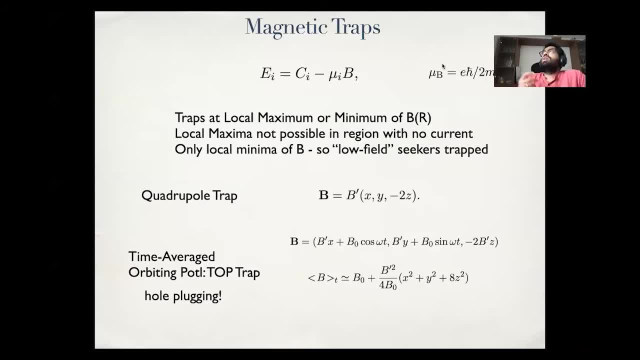 which is Bohr magneton. Of course the nuclear and the protons neutrons, all of them have some magnetic moments as well, but those are tiny compared to the electrons moment. So you can actually trap with such configurations, The most popular configuration. 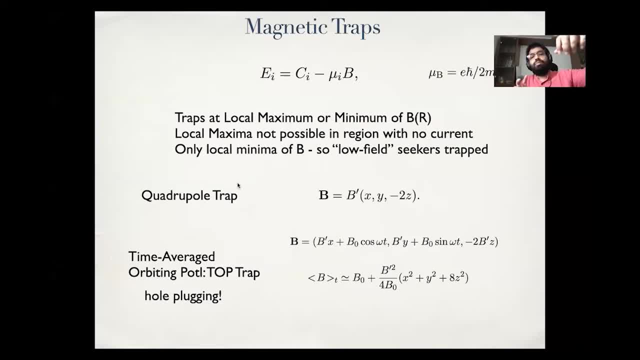 simplest configuration is called a quadrupole trap. You can actually design it by. you might have seen this in your basic magnetostatics calculations in undergrad, where you put two coils, two circular coils, with oppositely directed current. you get a minima in. 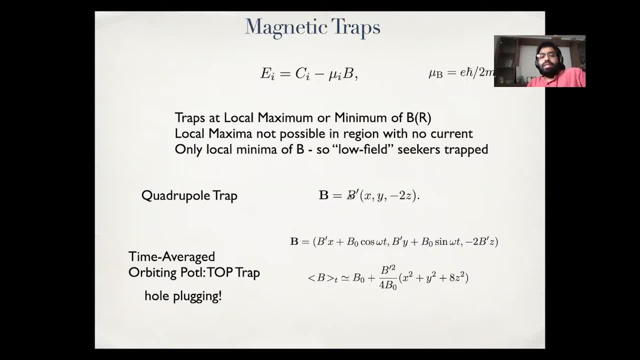 the middle. So such a trap is called a quadrupole trap. and this quadrupole trap has this form: the magnetic field depends on x, y, z. So when you basically look at mu dot b, then it gives you basically a very nice dependence where you have a minima at the point x equal to y equal to z, equal. 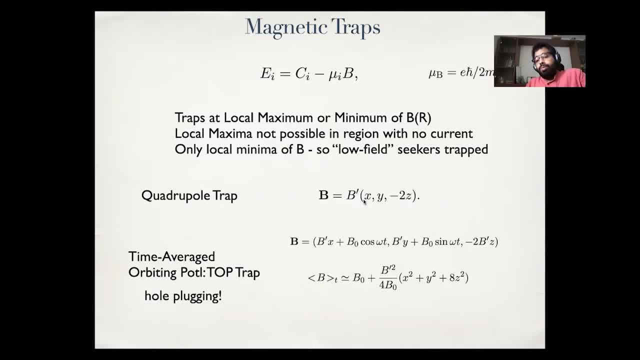 to zero, right? So then, there is one small problem with this. The problem is that there is a zero. you are trapping your atoms at a zero magnetic field. This is not very advantageous. This has a problem. The problem is, what are you doing when you're assuming that, basically, as I move in, as I apply a position? 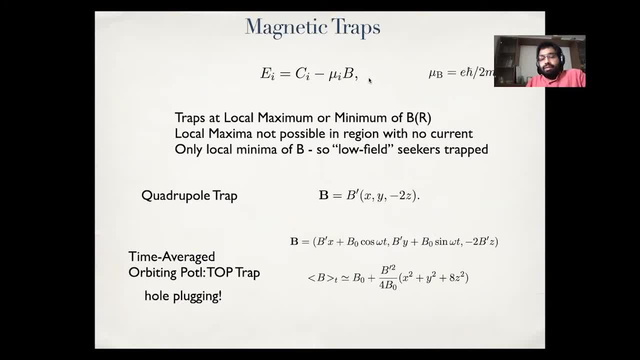 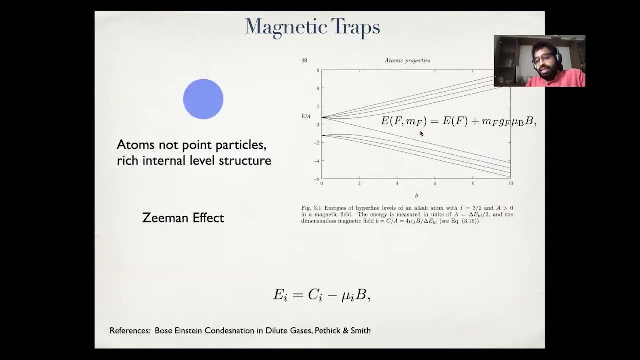 dependent magnetic field and my atoms move in such a potential landscape created by this. I'm assuming that the internal level of my atom is always on the same branch right, So it doesn't move to any other internal level states. As position varies, I'm going to move somewhere. 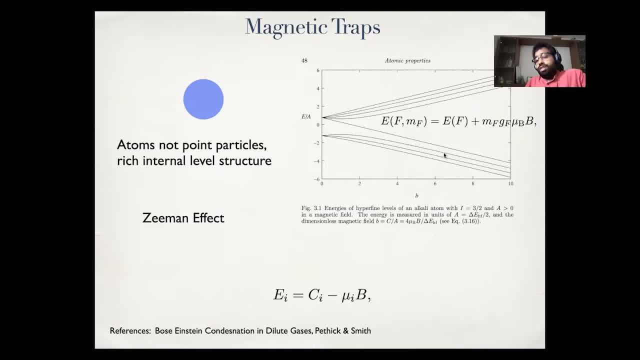 on this line, But the problem is this motion is not very slow for a hot atom. Sometimes you can also have processes where I jump into one of these higher levels right, And since the energy gaps between the higher level and the lower level are smaller, at smaller b field, very close to zero field. 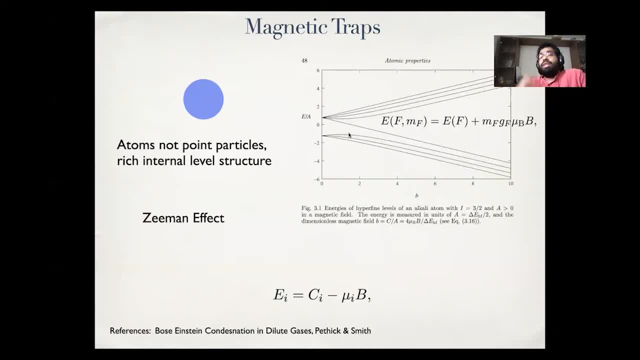 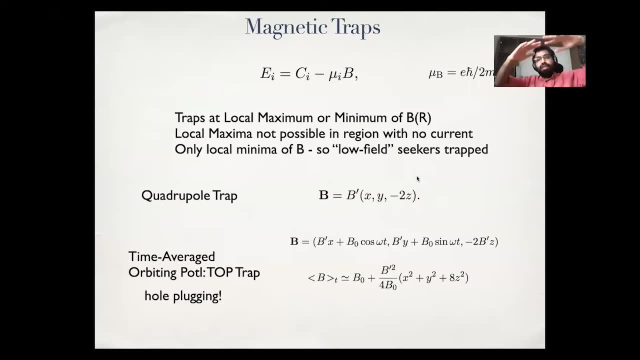 what happens is you can, actually the internal state of the atom can flip from the one that you can trap. Then what happens is you have a quadrupole trap and all the atoms like really go close to the, to the point where you want to trap, and then they just escape. There is a spin flip and they escape. 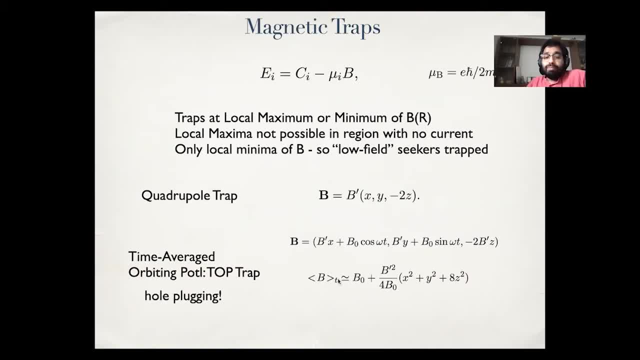 And this is a problem, So it's sometimes called as a hole in the trap, And you can plug that hole by other configurations. This is called a top trap, where you add an oscillating component And this oscillating component, when you time average it, you end up with a trap of this form. 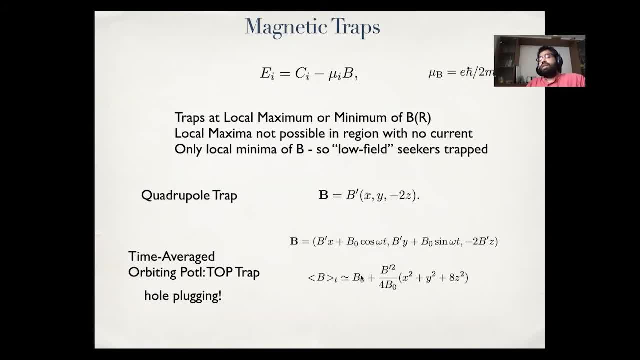 right. So this is a very nice harmonic trap And it also has a non-zero b field value at the, at the x equal to one. So this is a very nice harmonic trap And it also has a non-zero b field value at the x, equal to one. 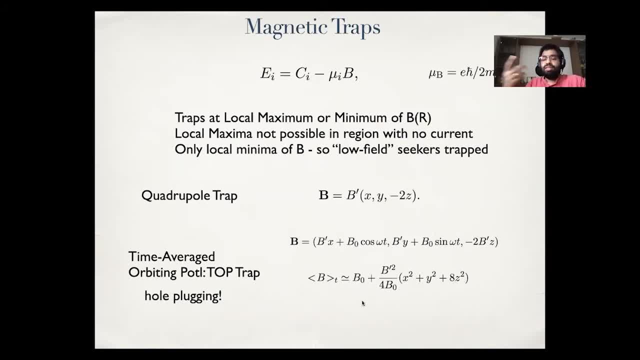 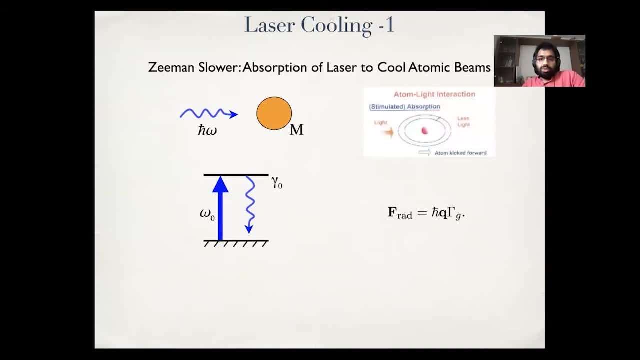 So this is like a hole. so this is how magnetic traps work. So that's one aspect. So you have a trap, but now you want to cool the atoms, So point. So this is like a hole. So this is how magnetic traps work. so that's one aspect. So you have a trap, but now you want to cool the atoms. so the fundamental idea of how to cool 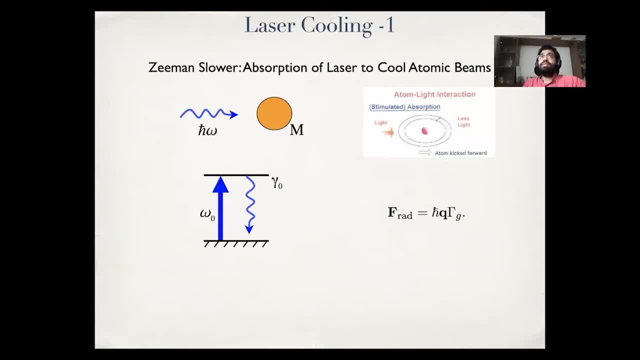 atoms again involves the fact that atoms have internal levers, but the main candidate for cooling is lasers. So the idea is that the atoms can interact with laser light. So in this case, it's basically the fact that the laser light has an electric field which is much larger than its 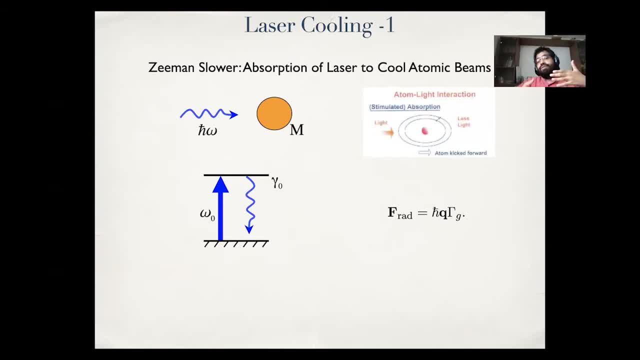 magnetic field, so it's an electric field- and the fact that the atoms have dipole moments. this is what causes this is sort of the fundamental physics. you need to have laser cooling. but let's look at how laser cooling works in a couple of scenarios. so the first scenario is basically a 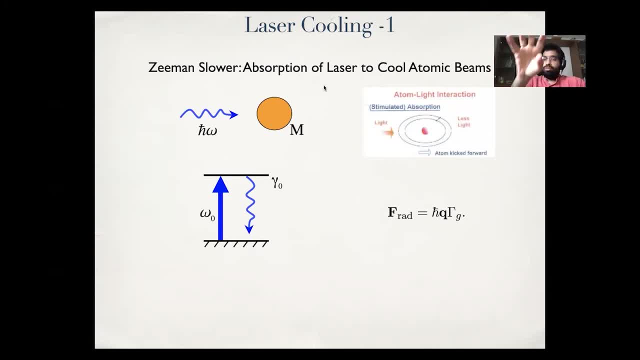 situation where i have an atom beam that comes out of a, comes out of some oven, and then i'm going to shine laser- repeated, i'm going to shine a very bright laser at it and from popular science fiction or just some thought, you know that there is some kind of radiation pressure that actually 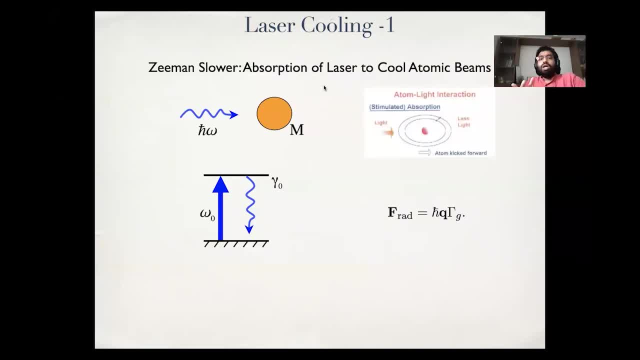 can stop my atoms right or slow down my atoms. so how does that happen? fundamentally, the quantum thing that is happening there is that the atoms absorb a photon that is coming at them. when you absorb a photon, your momentum. so when you absorb a photon, you get a momentum recoil in the opposite. 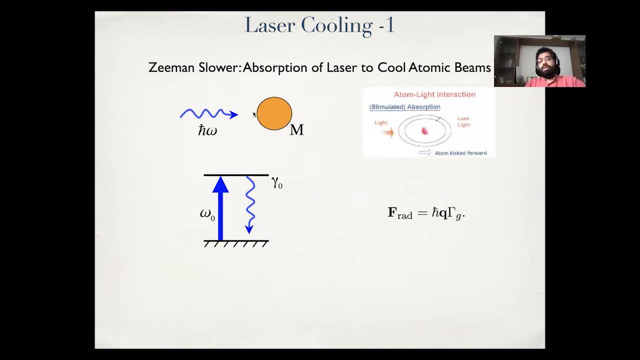 direction to the photon. so if this is coming like this, i lose momentum in the forward direction and i slow down. but of course, if this were the only issue, then i can basically, you know, make all sorts of cool devices with my lasers. but there is another additional. 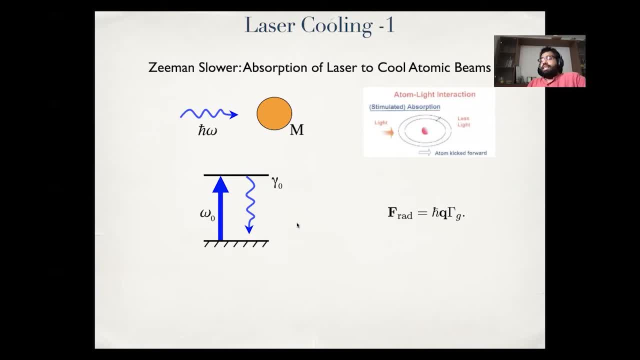 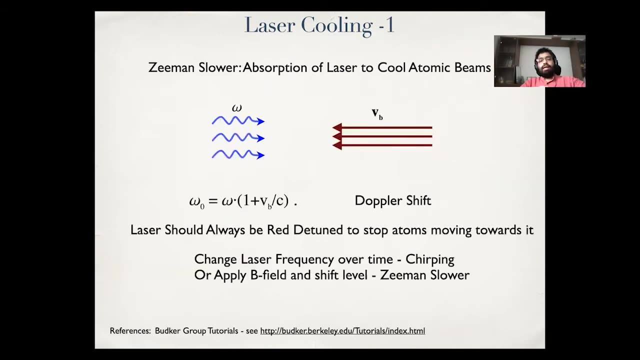 feature. just as i can absorb a photon, eventually an atom can actually spontaneously emit a photon. but the our luck and what helps us to actually use lasers to slow down atoms, is that this spontaneous emission is essentially- i don't have a picture for that- the spontaneous emission is essentially. 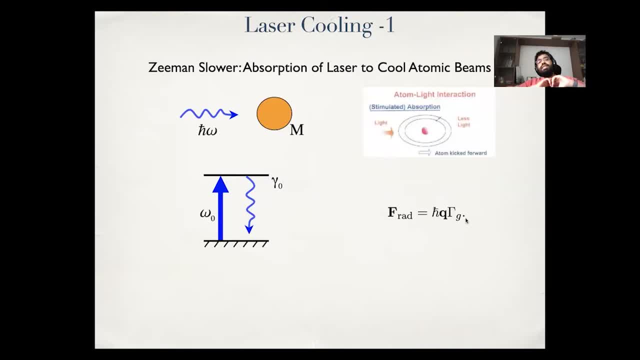 which is read by this gamma zero or this gamma g. this spontaneous emission is essentially. it can happen in any direction. so the spontaneously emitted photon, by the light, by the atom, can go anywhere with some distribution in space. but it can go anywhere, it is not always emitted in the 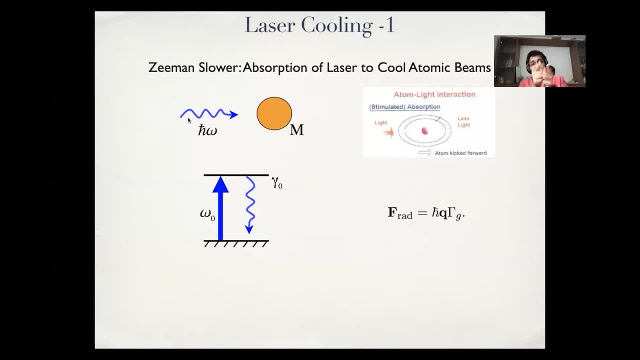 same direction as the original photon, because if it were preferentially emitted in that direction, then of course you have no momentum loss. but because it can be emitted in this in space in different directions and it's very randomly emitted on an average, the recoil that you get 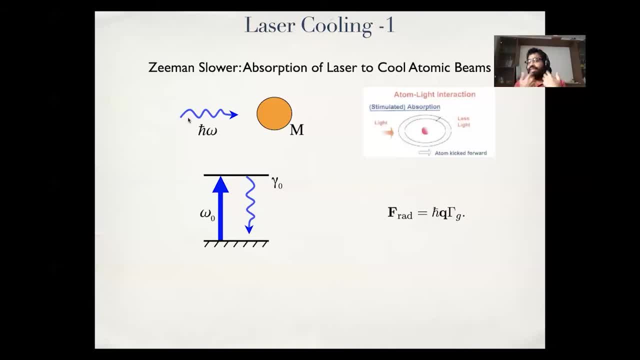 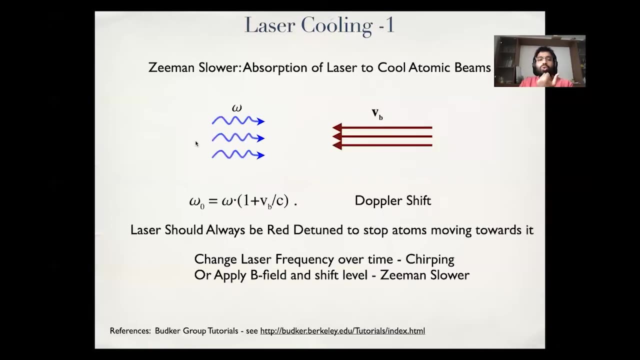 due to spontaneous emission doesn't slow you down, it doesn't change your average momentum. as a result, i can basically shine lasers on the on, on an atom, on the blue, on a sort of a beam of atom, and i can cool them down somewhat. uh, so this is regularly used. but uh, how do you do it? you can do it by 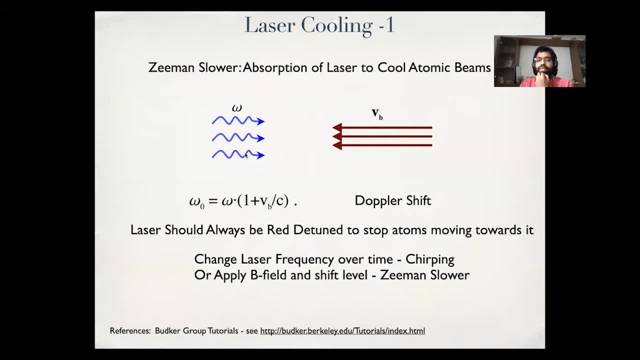 doing it with atoms. there is a small catch when you try to do it with an atomic beam, and this is got to do with doppler shift, which can be again exploited to make a better cooling mechanism. but let's first understand what happens when i have like a hot cloud of atoms that is released from. 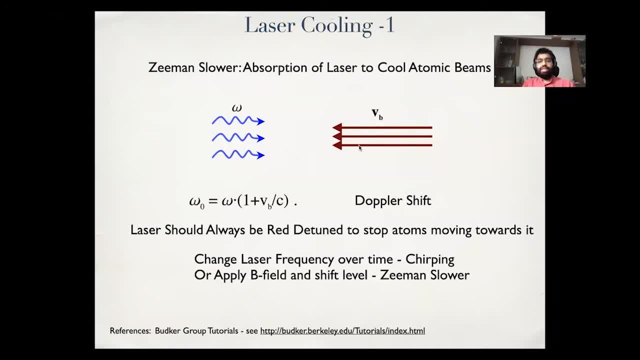 an oven and i'm shooting lasers at it and i'm trying to slow it down. so now the problem is: it is true that i can use the process that i said and i can sort of cool down my- uh, my atoms, but as my atomic velocity slows down, 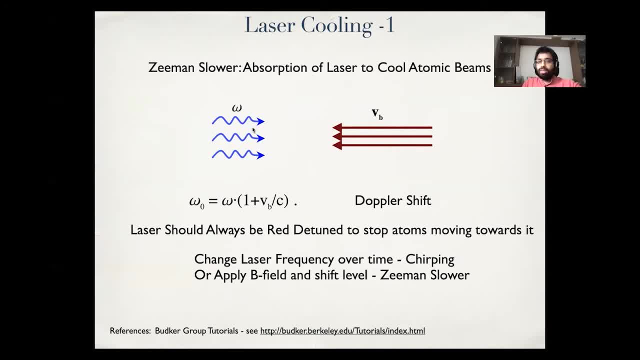 because of the doppler effect, atoms that are moving towards my beam will actually see a frequency that is larger than the applied lasers frequency. right, so if the laser photons in their frame of reference, the laser photons are going to be, uh, blue shifted, or basically they're going to 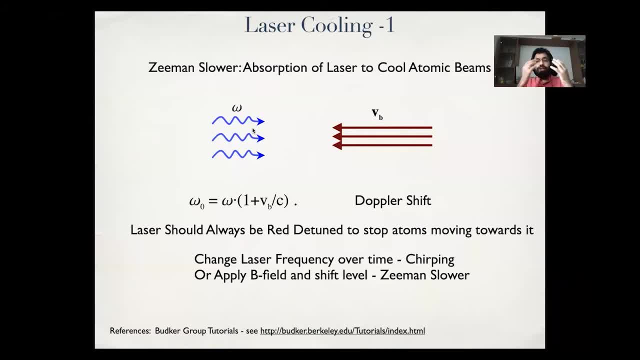 be. if you're moving towards the laser beam you will see a larger frequency photon and that is a problem because my energy levels that i have for my atoms, they have a particular resonance frequency. if the frequency of the photons is larger then i'm not going to be able to cool down my atoms. 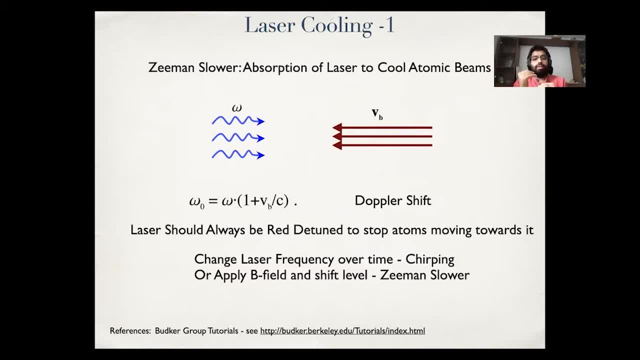 not able to efficiently absorb these photons. right, so i'm in trouble. so what, how do you? what do you do? so what do you do is very cool, which is you always send in light that is of slightly lower frequency. but now there is the additional problem as you keep, uh, slowing down the atoms, the frequency you. 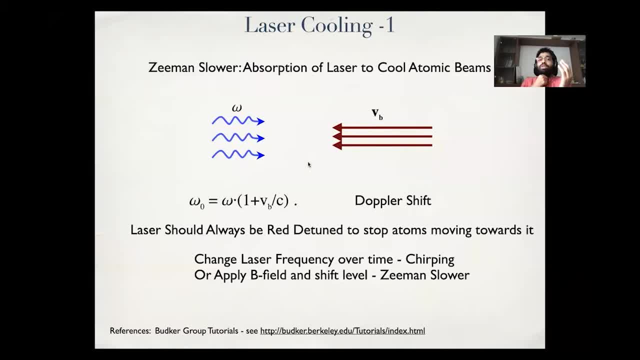 have to drive with. you have to make it also different. right, because the red shift is going to be the doppler shift, which is to this leading order. like this, that is going to be very different. the laser light that I should apply, omega, should also be changed right so now, which means as the 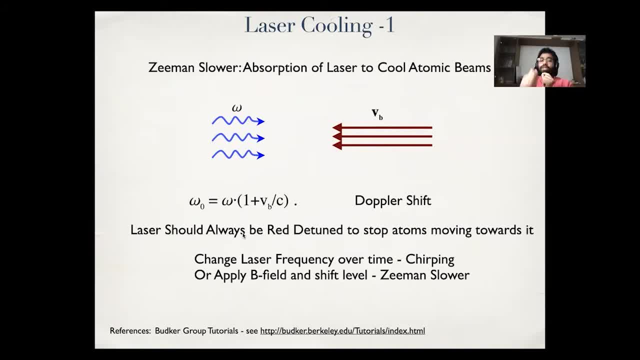 as I slow an atomic beam, I have to slowly change the frequency of my laser over time, which is one technique one can use, which is called chirping. or you can do again this beautiful thing with magnetic fields, where I apply a non-uniform magnetic field along the position direction. 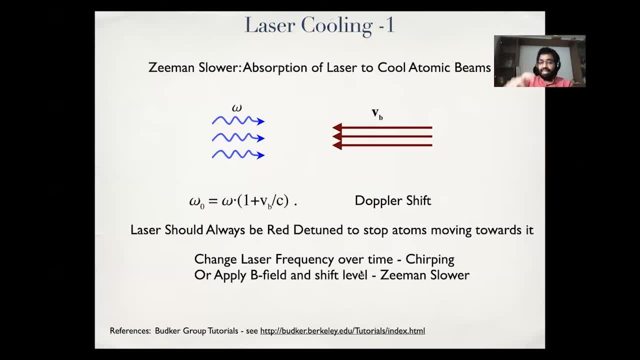 and, as a result of this magnetic field, it shifts exactly my atomic resonance by the same amount, such that, such that I'm basically changing omega 0. so I can either change omega or omega 0. omega 0 I can change by applying the magnetic field. omega I can change by chirping the laser frequency. 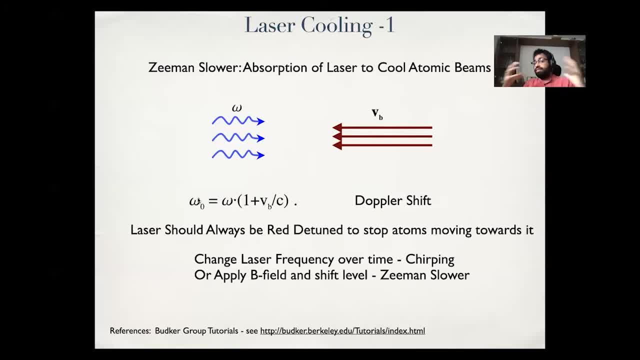 either if I change omega 0 by applying magnetic field. this is actually a very beautiful piece of equipment called a Zeeman slower, and so you can use that to cool atoms. so that's what is the first stage of any kind of laser field. So once you do that, you get slightly colder atoms than just thermal room temperature or even hotter. 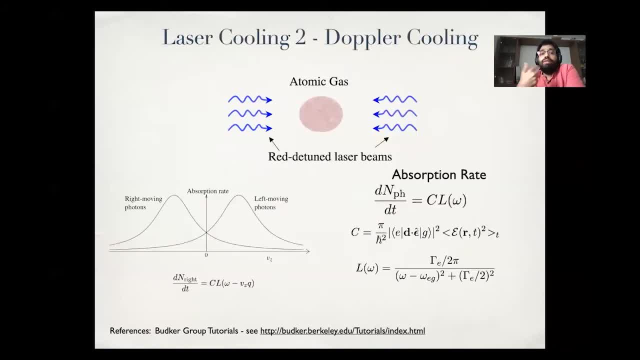 atoms. but that's not enough, so we have to cool even further down. the second kind of cooling that is employed in these Bose-Einstein condensate systems is called optical molasses or laser cooling. in this form, where I have an trapped atomic gas somehow trapped, let's say, in a magnetic, 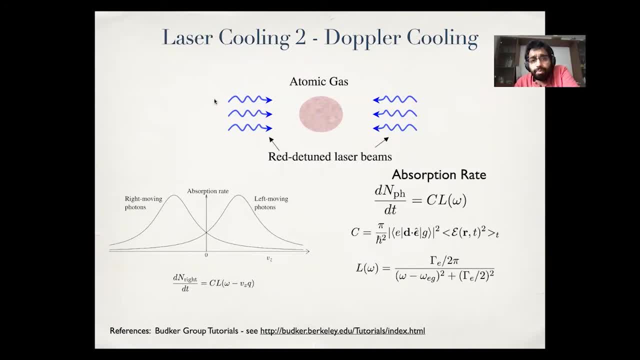 trap. and then I have. I apply from all, actually in three directions. I apply red detuned laser beams, so there will be six laser beams that are applied on. let's look at one direction alone and understand how applying these red detuned laser beams allows us to cool. so the cooling mechanism is exactly as before. I basically get photon. 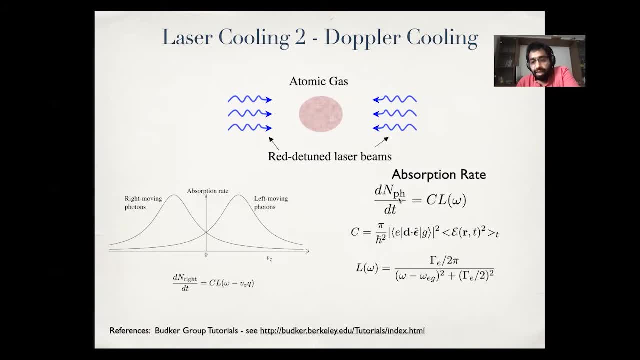 photons are absorbed by the atoms and that absorption is what is causing the cooling. the rate at which my atoms absorb the photons is. the rate at which my atoms absorb the photons depends, of course, on the dipole moment of the atom squared. the strength of my applied 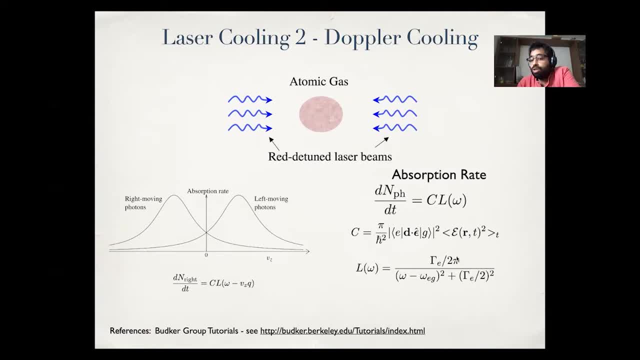 field. but it also depends on this response function, which is basically a Lorentzian function that tells us that the atoms are like an oscillator that can actually just pick up energy precisely at this omega EG or omega zero, but with some error that is given by their spontaneous lifetime. 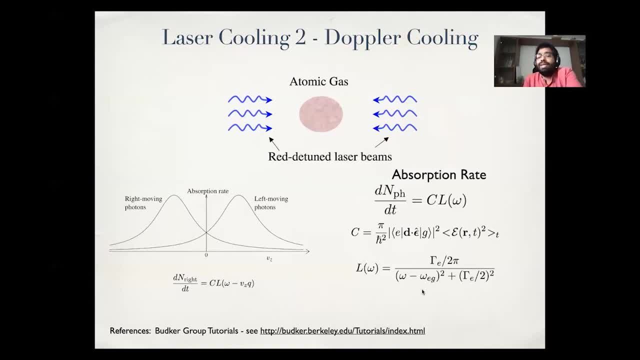 or the width, right? So I'm just thinking of a very simple model of an atom with just two levels, okay, and in this picture, what happens here? so what happens is physically something very nice happens, which is if I have an atom that is basically at the middle, at exactly at z, equal to zero. 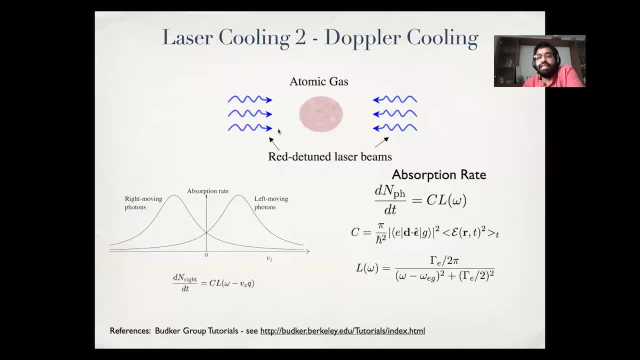 it will equally absorb left and right movement. That's not going to have a lot of effect. It will have a lot of effect If I do not absorb the energy. it will not absorb the light, which what happens is I can actually see a little bit of object, which is the current that is in front of the atom. 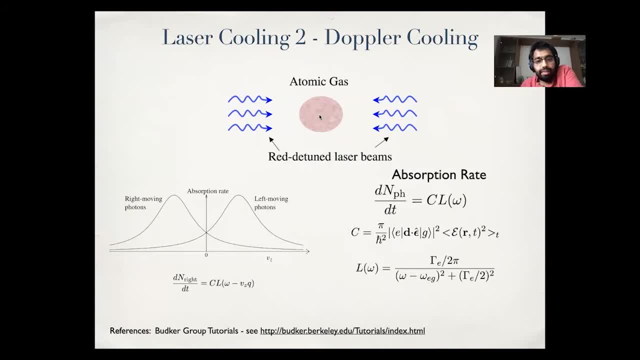 and I can also see that the current is beating more and more and more and therefore I can see that the current is at the right momentum and therefore I can see that the current is moving at the right velocity. So that's another technique which is showing that the current is really moving, even when 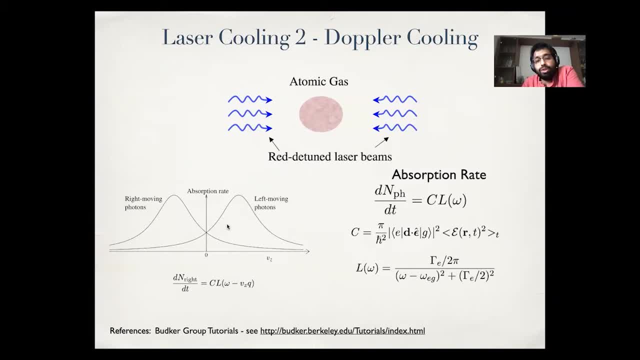 there is no interference in the pattern, which basically means that the current is not moving. All right, So this is the plate. so what I mean is that I will see this and this is actually charged, is I'm going to. the atoms are going to see the right moving photons with frequency that is actually lower than original frequency. 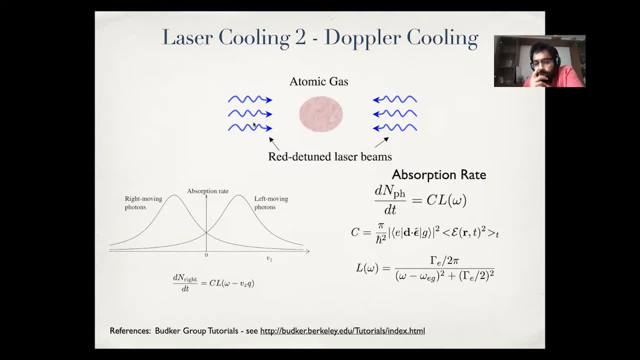 Both these frequencies are tuned to be below the atomic frequency, but this will become even lower Right. So then it will, But on the other hand, the left moving photon will actually be. its frequency will be increased, and it will be because of the Doppler effect. 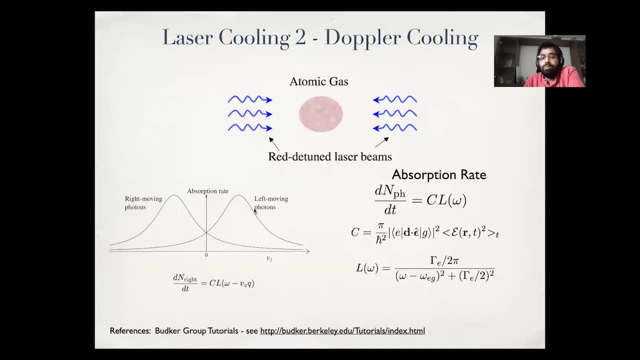 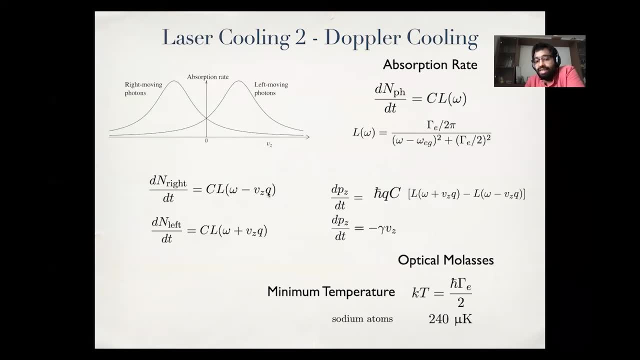 It's more likely to be absorbed Right. So let's put this into math. So if I look at my right moving absorption of right moving photons, I have to take omega minus my velocity times Q, And I evaluate this at omega minus velocity, my BZ times Q. 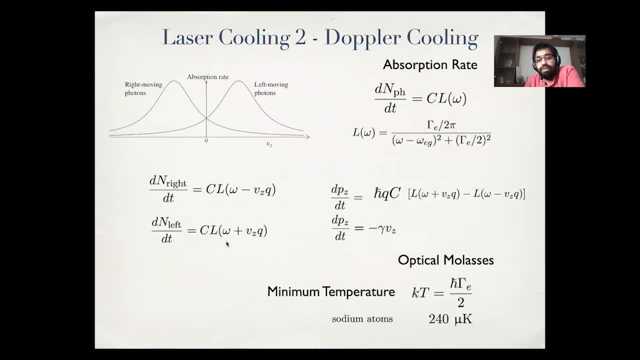 On the other hand, the left one, which is these photons, they will be absorbed at omega plus BZQ due to the Doppler effect. Now, basically, my change in momentum Right. So my, my change in momentum, My change in my average momentum is basically H bar Q times the absorption. 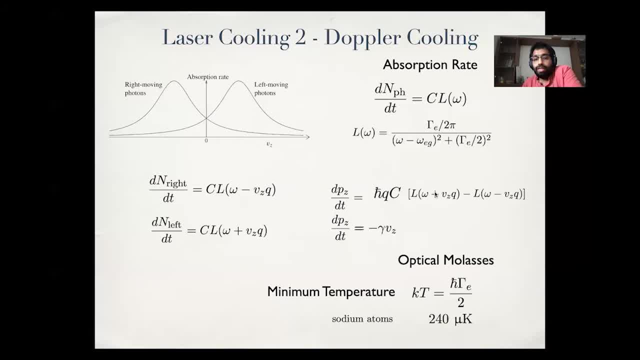 Right. So this is H bar Q times. the absorption of the left moving photon will give me a H bar Q kick, Whereas the right moving photon will give me a minus H bar Q kick. So that will be my total absorption rate. This part and that times H bar Q is my momentum change. 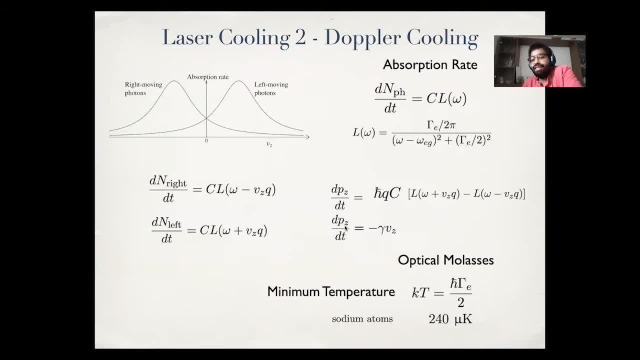 And when you actually write this down and calculate it, you get a very nice answer which is DPZ By DP, the momentum change has a minus gamma times BZ, which means- and this gamma is a positive number which depends on this whole thing- Not important. 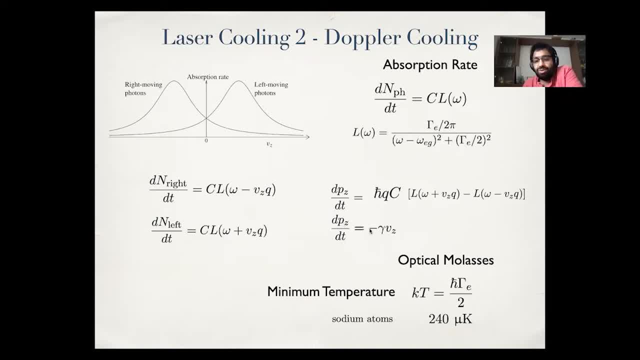 But the basic idea is that P is V, So this you can write it as basically damping of my velocity. So what I get is actually a frictional force due to this configuration of two lasers, And this is what is called an optical molasses. 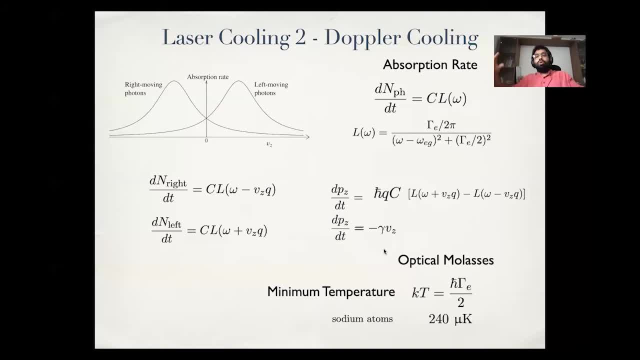 And, as a result, I am sort of my my momentum slows down further and further. How small can I make my momentum? So if I take a momentum distribution which is basically P squared averages of the order of KT, So my width of my momentum distribution is KT. 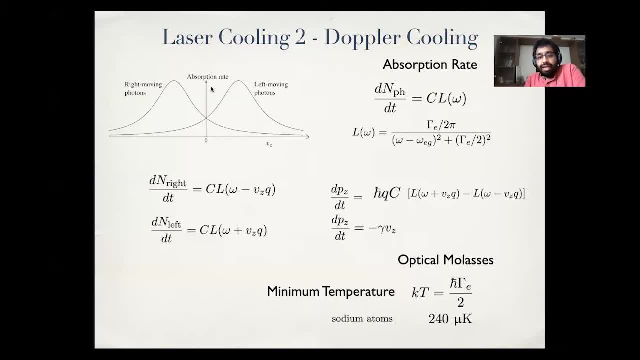 I want to be able to distinguish between the right and the left moving photons. That is when I can get this cooling effect, which means if my momentum distribution- once basically the momentum distribution- becomes small enough that I cannot do this distinguishing, I basically cannot cool any further down. 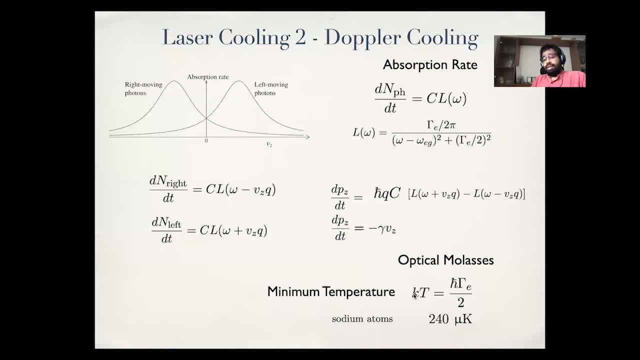 Basically, once I add temperatures for four temperatures lower than this, basically I cannot use the Doppler cooling optical molasses idea And this is the lowest temperature I can get to, And this is about order of 100 micro Kelvin. OK, so this is what happens at the second, typically the second stage. 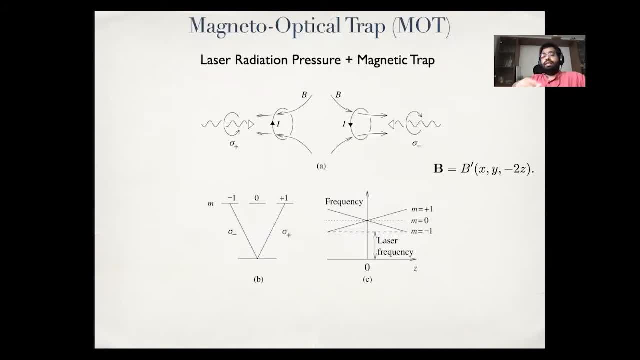 But there is a more efficient way of doing this: laser cooling, Using a combination of magnetic trapping and laser cooling, which is called the magneto optical trap. So this is the workhorse of ultra cold atoms and Bose Einstein condensates, And this works in a very clever way. 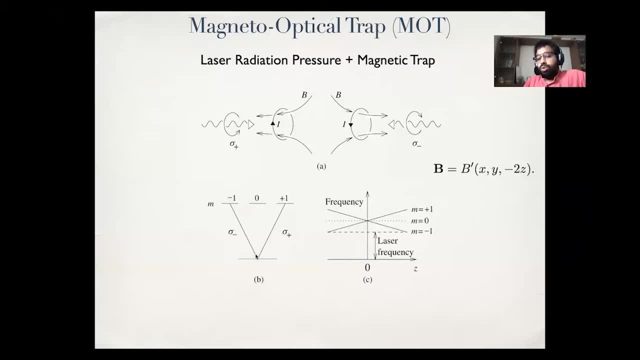 So the idea now is to have a, instead of a two level atom which was absorbing photons with some linear polarization. Now I'm interested in an atom with excited states of different magnetic, With different angular momentum. For example, my ground state has no angular momentum, but my excited states can either have minus one, zero or plus one. 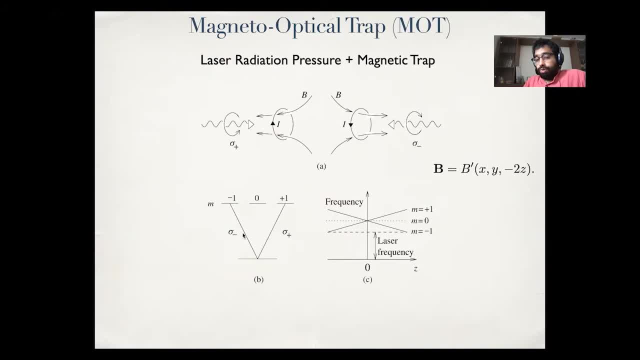 So now, if I want to go and absorb, if I want to make a transition to a atomic state with a different angular momentum, of course I have to absorb basically a photon that has some spin. That is which means I have to be in one of these circular polarized states. 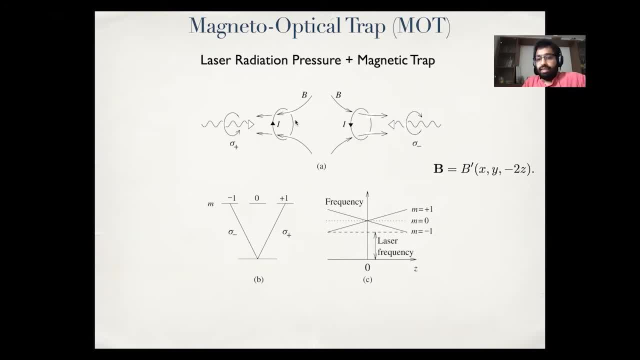 OK, so then the idea is to basically consider A regular magnetic trap, like our quadrupole trap, and trap atoms in the center of this trap, And then, from the left and the right, you apply basically a plus polarized light, which couples zero to plus one state, and a minus polarized state from the right, which couples from zero to minus one. 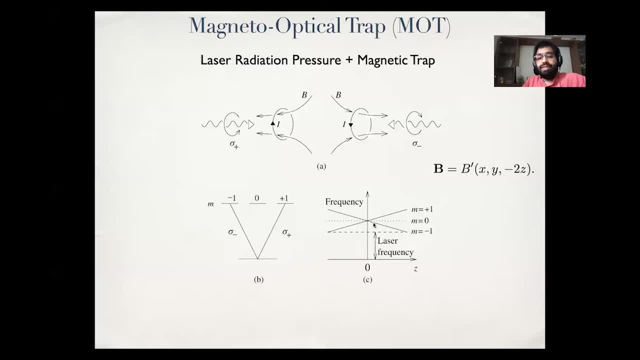 Now the interesting thing is the energy level, and you put the laser at some red detuned value. OK, so the laser frequency is here. These are the atomic levels. Now the idea is basically the gap between the minus one and the zero and the ground state. 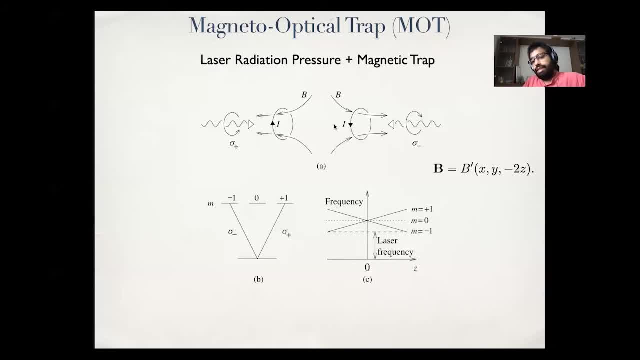 Basically, if you take an atom that is at the center and let's say it moves a little bit to the right, So Z becomes positive, So let's call this Z and Z becomes positive. Now what happens is basically the M equal to minus one state. 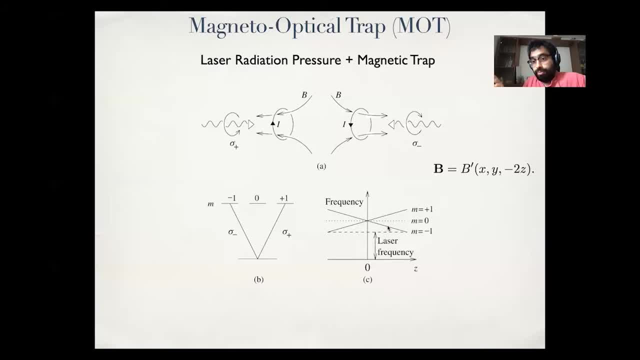 Its energy decreases because of the Zeeman effect, because of the magnetic field configuration Right Now. as a result, my laser frequency becomes closer to my atomic frequency and hence I absorb more of the light sigma minus light that couples zero, the ground state, to the minus one state, which means I'll absorb more of the laser light that is coming at me. 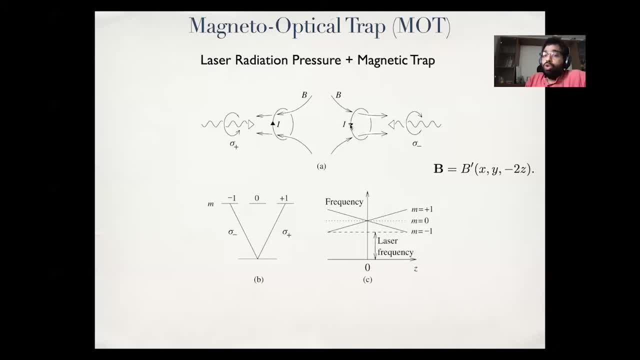 which means I'm going to get kicks towards the Z equal to zero. And you can see from this configuration that the exact opposite happens. when I move to the left Right, I absorb more of the sigma plus. So with this clever scheme you can really cool atoms down a lot. 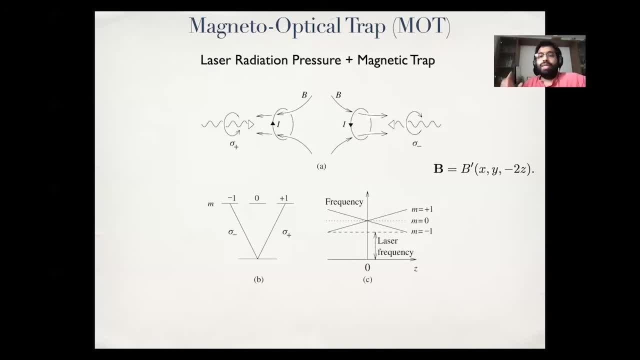 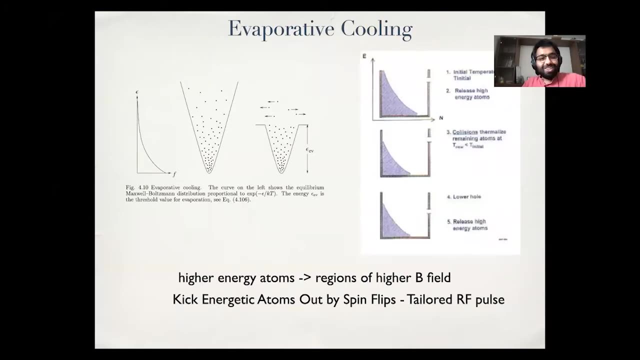 OK. so you can get them down to typically, if you make a very good mod- to even lower than this 240 mu k. But once you have done that, that is still not enough to make a Bose Einstein condensate. The final step in cooling is actually in a sort of a cruel twist of fate in some sense. 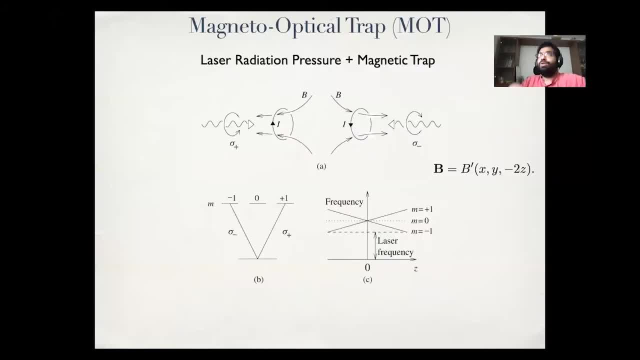 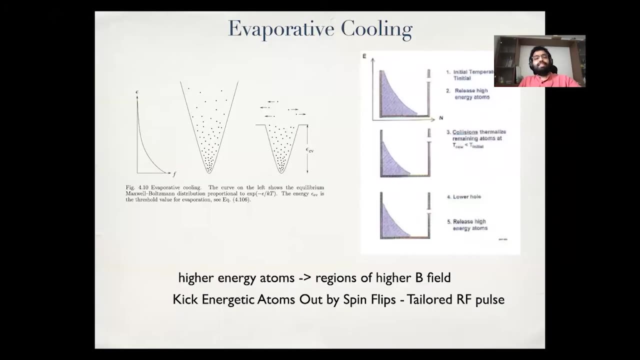 People found out all these clever schemes to make, You know, cool down atoms And there are Nobel Prizes for, for you know, for for these kind of laser cooling that was awarded. But the final step that one had to do to really get to the Bose Einstein condensate was literally something that happens every day. 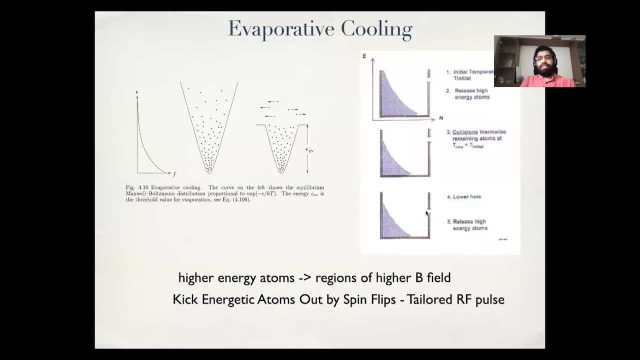 So I'm drinking a cup of coffee and I took the coffee when the lecture began and it's super cold now. So what has happened? Basically, there is like a hot vapor, So some part of the water in the coffee was vapor state and those hot vapors have evaporated. 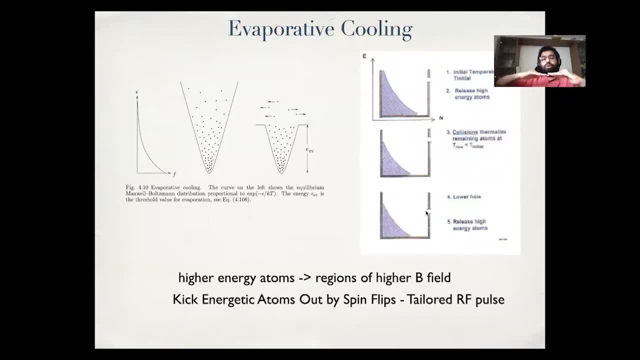 So the you basically make a way to take a gas of atoms that is at some temperature and you cleverly find a way to kick out the most energetic atoms. OK, when you do that immediately you get a state that is non equilibrium. It's not a thermostat anymore, but then the atoms have interactions. 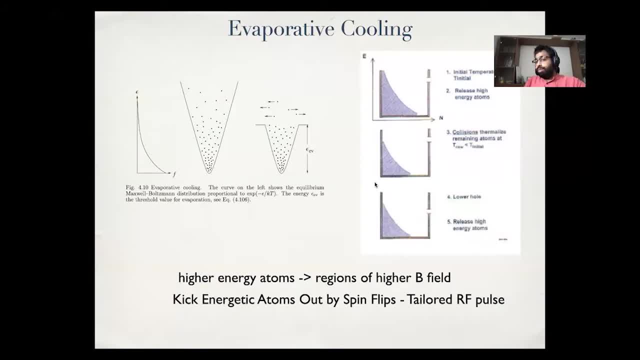 They collide and they settle down to a thermostat. But now the thermostat will be off Much lower temperature. OK, the way you do that in an ultra cold atoms experiment is after you've made the temperature to a certain value with the Mott. 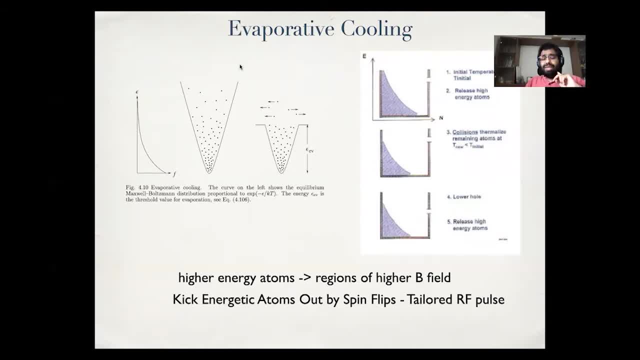 You transfer to a purely magnetic trap, like this quadrupole trap, And then you apply, basically, RF pulses which flip the atoms from a low field seeker, which is trapped, to a high field seeker that will leave the trap. Moreover, you choose the RF frequency such that 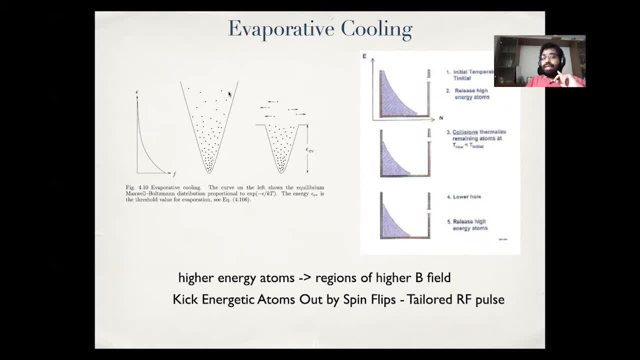 You basically only flip atoms that are far away from the center at higher energies. OK, so you can choose that frequency, So the atoms that are already at lower energy don't get kicked out, but the atoms at higher energy get kicked out, and that lowers the temperature a lot. 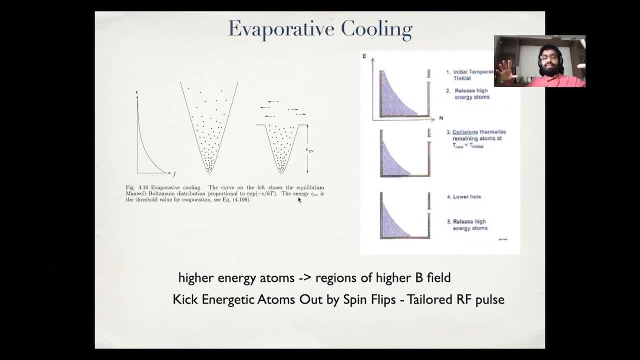 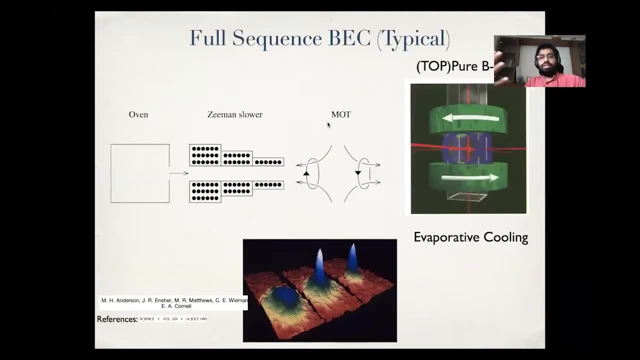 OK, this is the final step of Bose-Einstein condensation, And after that you actually get a Bose-Einstein condensate. So to summarize what is the typical full sequence of Bose-Einstein condensate to produce a Bose-Einstein condensate. 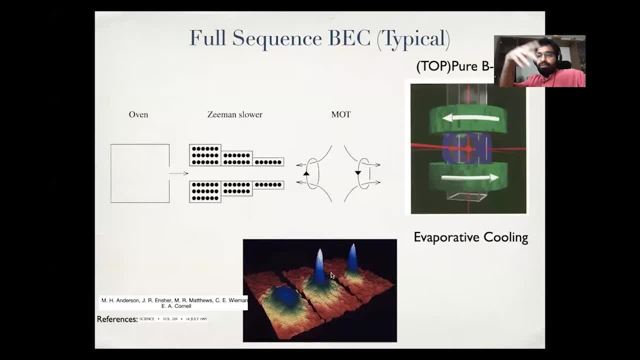 Well, you get a Bose-Einstein condensate. that is followed, for example, in this landmark paper that we have seen a few times now. Atoms come out really hot from an oven. You use this Zeeman slower and a laser that is applied from here and it cools down the atom further. 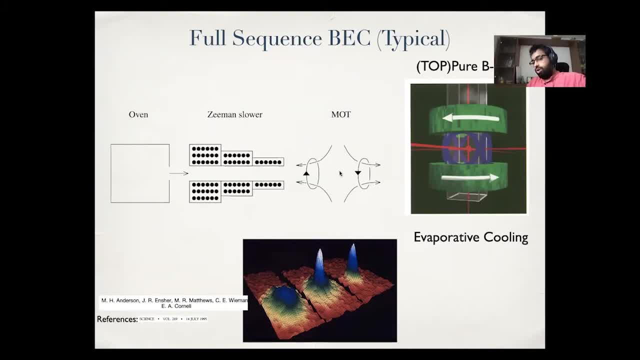 And then this allows a slightly hot- but still not so hot cloud to be loaded into a Mott And because of this Mott you trap a bunch of atoms in this Mott. Then you turn off this Mott and purely have one of these magnetic traps. 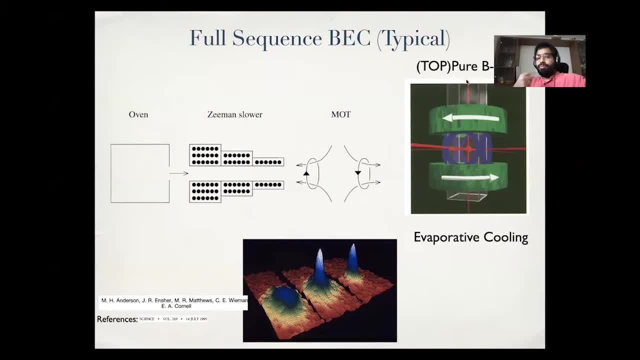 So in this experiment they did this top trap with this oscillating field, with the hole in the zero plugged, And once you have that, you basically apply RF flips and implement this evaporative cooling. Once you implement this evaporative cooling, voila, you have your Bose-Einstein condensate. 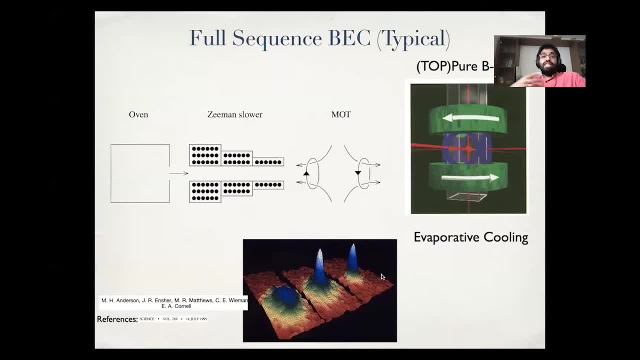 OK, so this is the magic that is done to actually get these objects we've been talking about for the last four days, And all of the considerations we made would be just meaningless, theoretical things if not for these beautiful experiments. So I thought I should definitely give some attention to them. 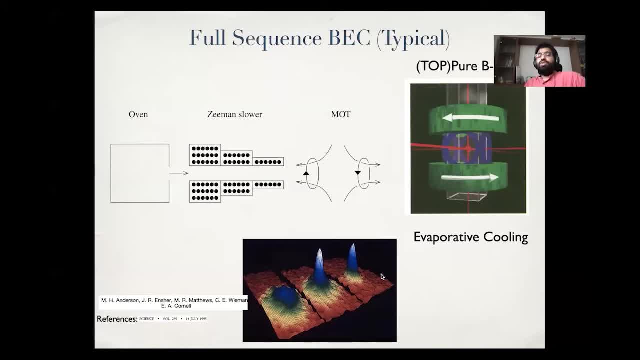 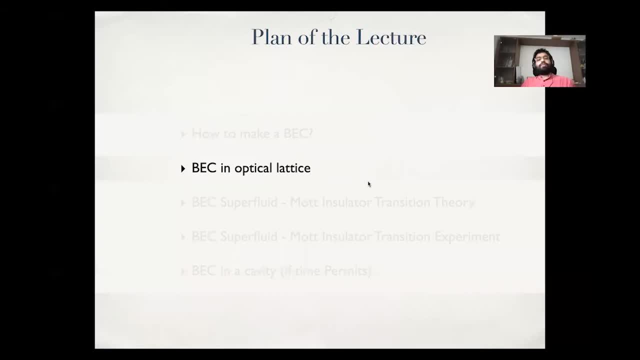 So I will stop it, And also because they have very beautiful quantum optics, So I will stop at this point before I move on. If there are any questions, I'm happy to take them now. The last method that you mentioned that finally came out. 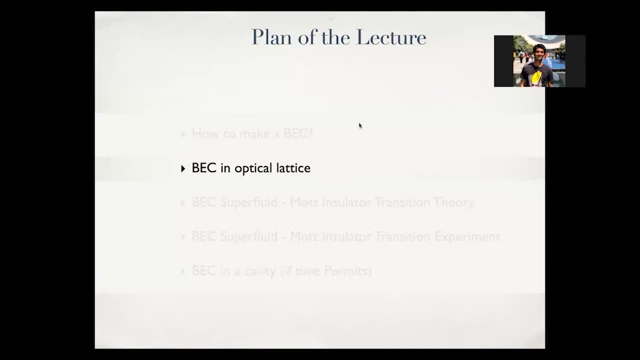 We have to do all the other things, like laser cooling and Doppler cooling and all those things, to get to the point where we can use this method, or can we do it from the beginning? No, So you really have to do all of the other things to do this method for a very, very cute reason. 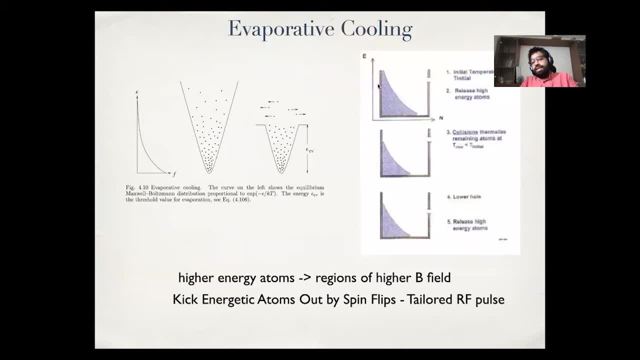 The cute reason is as follows. You see, the success of this scheme is not just allowing the fast moving atoms to leave. Whatever is left should be able to terminate. It should be able to terminate, which means you should have enough of this density, or, more more accurately, what is called this phase space density. 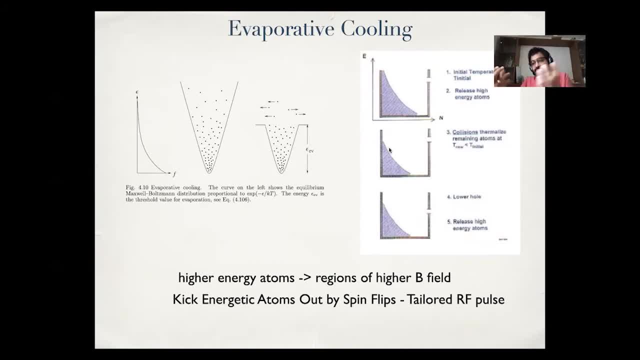 So this N lambda cube should be significant enough so that there are enough collisions for the gas to terminate to a lower temperature. Otherwise you get some non equilibrium state that is never going to be a Bose Einstein. That's why you use the first cooling process to get enough cold atoms with enough density. 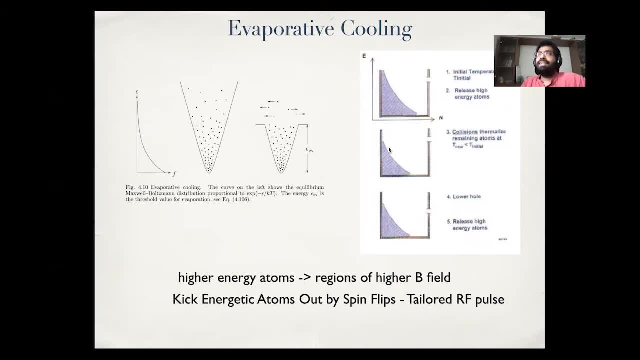 So that finally, you can do this evaporative cooling. And in fact, even though I framed evaporative cooling, as some you know, junk simple idea, The whole point was: how do you get? everyone knew you have to do evaporative cooling at some point. 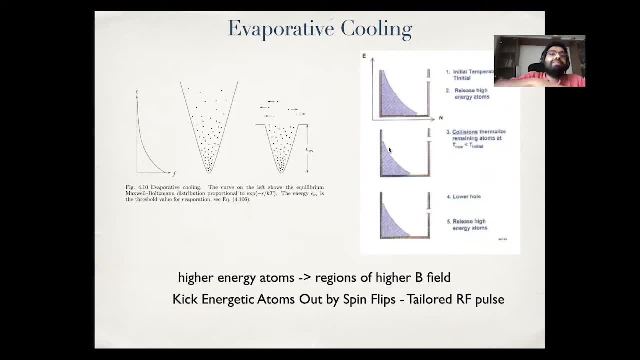 But how do you get to that stage and how do you combine it with this laser cooling? That is where the whole genius of Eric Cornell, Carl Weiman and Ketterle and all the other people, all the people that have worked on it- 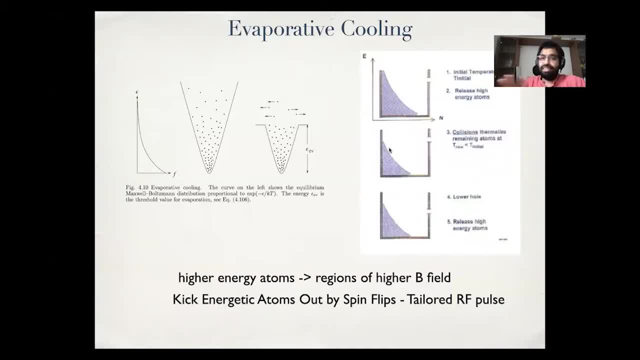 So that's really required a lot of technical stuff that I A- I can't say I can't cover it here. B- I don't know a lot about it myself as a theorist, but it wasn't easy. Let's say it didn't take 20 or 10,, 10, 15 years for these people. 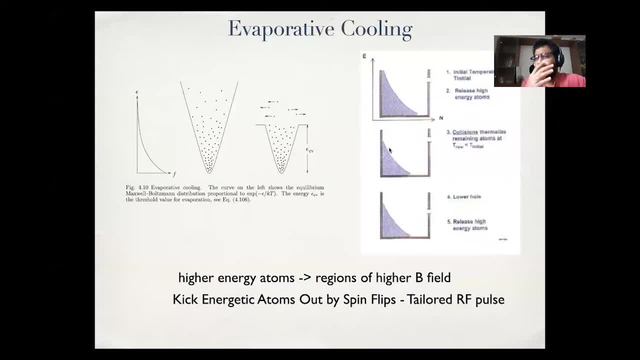 After laser cooling: 1990. laser cooling laser cooling was known in 80s and I took like 10, over 10 years to get to a BEC, So it is non-trivial how to get to it. Yeah, Did I answer your question? 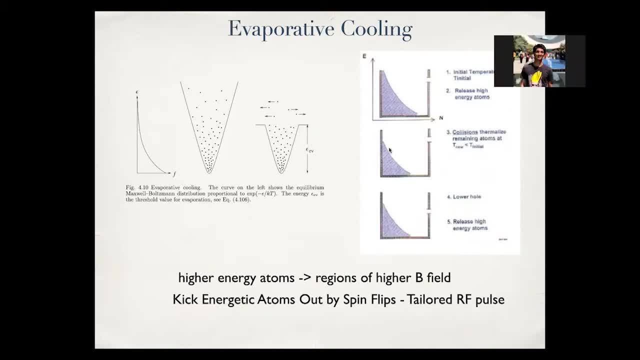 Yes, but I think I like to read up more. So basically, you have to do enough cooling so that the density you have to cool and collect enough atoms, without which you can't do evaporative cooling, That is the main idea. Yeah, I understand. 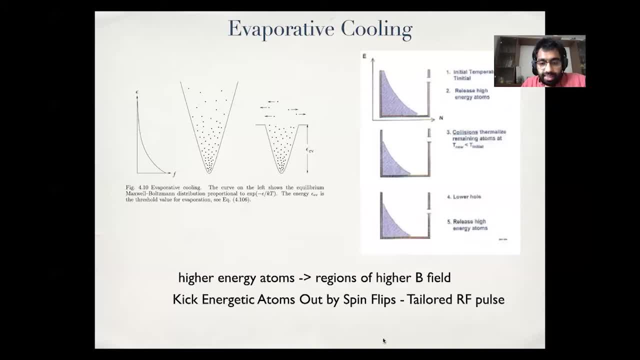 OK. Also, if you are putting something in the chat, somehow I can't see the chat so well. OK, now I can see. OK, In this case, the environment Is always hotter than the sample. How are we shielding the sample from environmental effects? 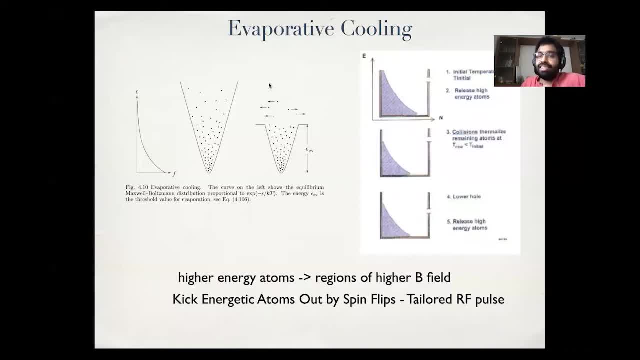 Very good question. One thing I never mentioned in this is everything is done at very high vacuum. If you don't have a vacuum chamber, you cannot do any low temperature or high or Bose-Einstein or quantum optics experiments. The good quantum optics experiments need high vacuum as well. 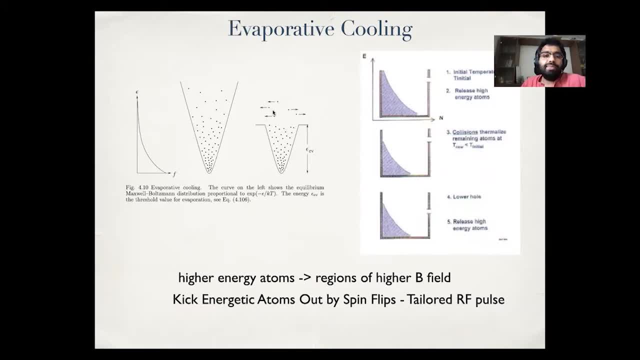 So that's how you remove all the environment atoms that are hotter. OK, Are there any further questions? You can unmute and ask as well if you want. OK, if not, let me move on. OK, good, All right, So. 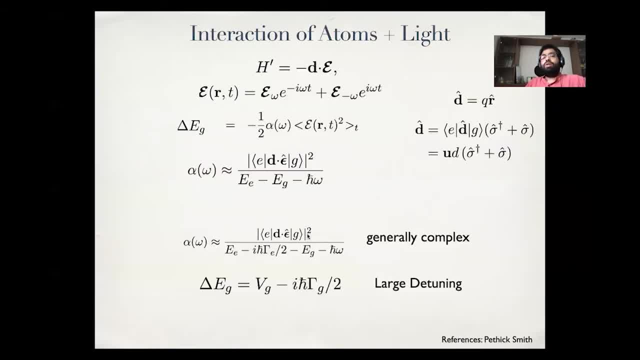 Let's move. Let me move on to the second part of the lecture, where I want to understand the theoretical and aspects of how, what, what happens what? what are these optical lattices? What? how do Bose-Einstein condensates in optical lattices work? 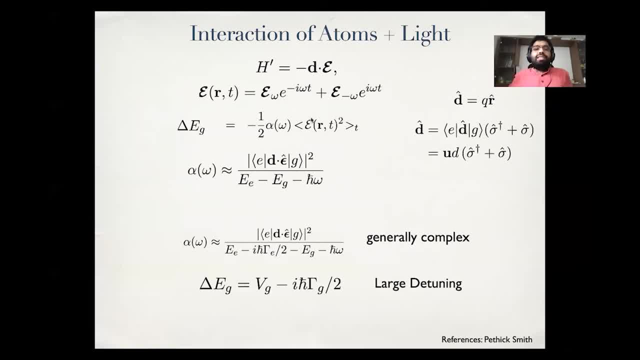 OK, so basically the idea in an optical lattice, as I mentioned, is to apply an electric field produced by a standing wave of light. OK, how does the electric field and the atom interact? It is basically a dipole, coupling with D, dot, E. 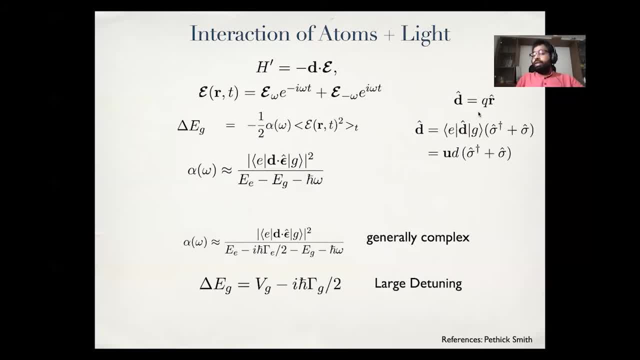 So the dipole moment, of course, is a quantum operator for an atom. In the simplest case, of course, a dipole moment is this Q times R, and you can expand it in the internal levels of the atom And it will basically have transitions between different levels. 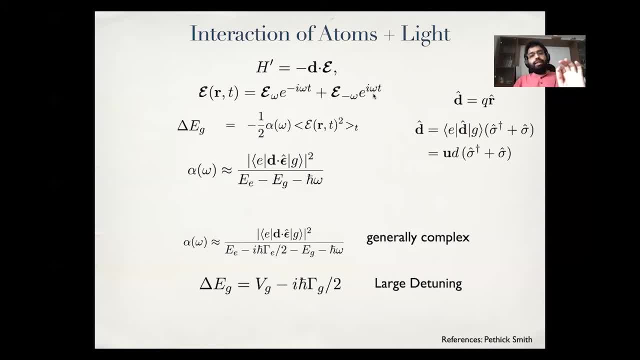 But if I'm going to attack with some periodic variation of light, so some some actual laser light with a fixed frequency, I can basically just worry about two atoms that are nearby resonance to this applied field And I can expand my dipole operator in this very simple two level form. 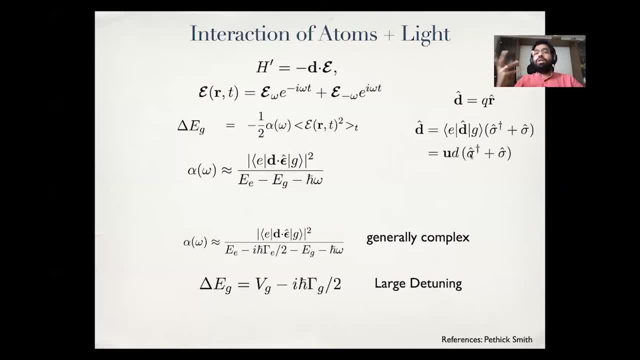 It's like a pseudo spin, half operator, if you want, quantum mechanically. With that, what can I do? My Original states basically is: my original Hamiltonian is EE minus GG, with the, with the resonance frequency E minus EG. And now I can treat this sigma plus sigma dagger, which is basically EG plus GE. 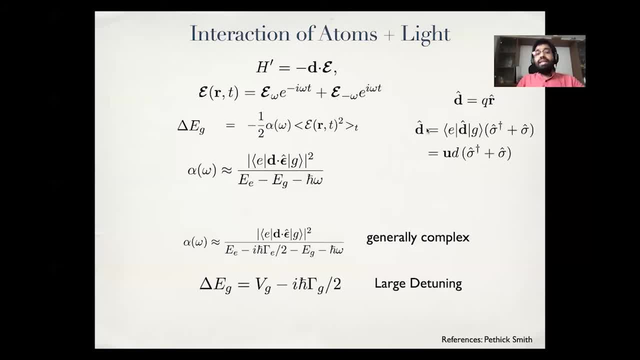 So it causes transitions between E and G as a perturbation, and do second order perturbation theory and write down how my ground state of my atom Is shifted due to the application of G, The application of this electric field. and I can write it in this manner, where this is an time average over the electric field applied: electric field square. 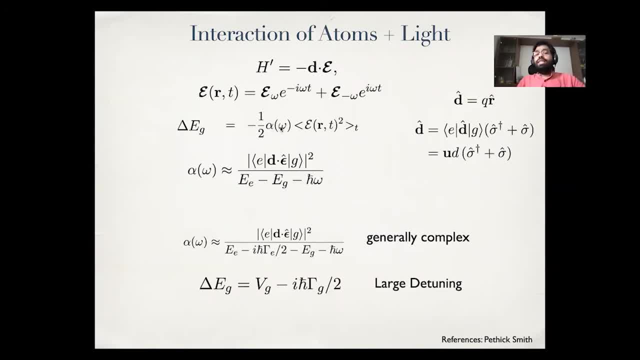 The intensity is time, average times and quantity. alpha of Omega, which depends on the atomic properties and which is called the polarizability single atom. polarizability of an atom, Of course it depends on the strength of my dipole moment, But it also depends on how close I am to resonance. 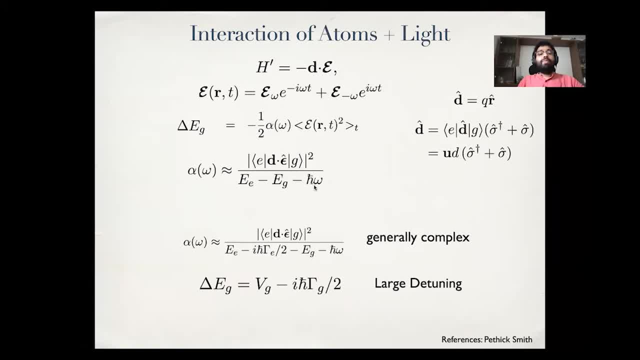 So what that means is that I can ultimately get an important result, which is the continuous emitting emission, with the spontaneous emitting EG minus H bar. Omega is the laser applied frequency. Now, of course, in general, my atoms do not have perfectly well defined resonance lines. 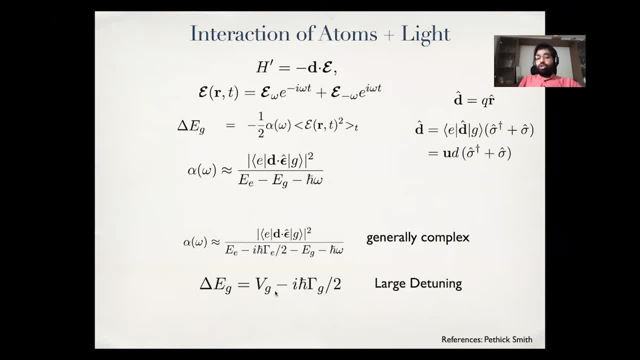 There is always some width, which is basically the spontaneous emission rate. One is a conservative, it's called a conservative form. I'll call this conservative potential in a moment, for a reason I'll come to, but it also can have a imaginary component. 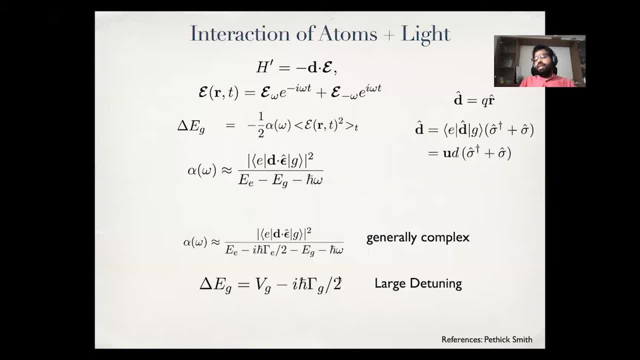 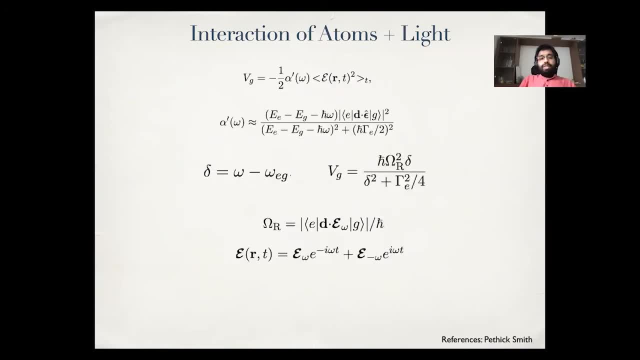 For these optical lattices and the kind of things I'm gonna describe. I'm typically going to ignore this spontaneous emission in this case, okay, So now what is happening? So all that I have is my. I can write my. basically, I can write my result of applying. 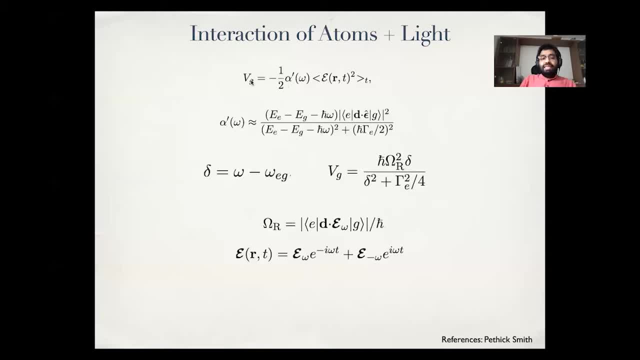 an electric field on my atom as basically providing an external potential VG of this form. okay, Now, this does a time average, but I can have some spatial dependence of the electric field, right. So that spatial dependence, all of it, goes into this so-called Rabi frequency. 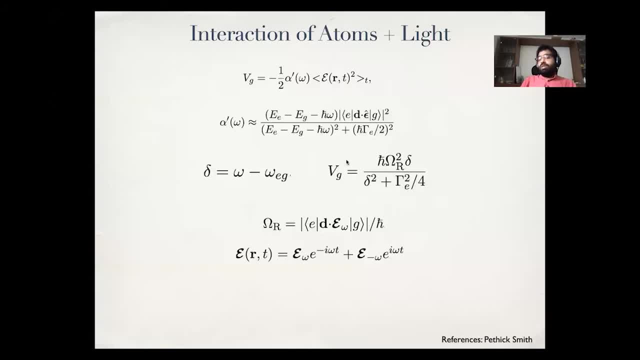 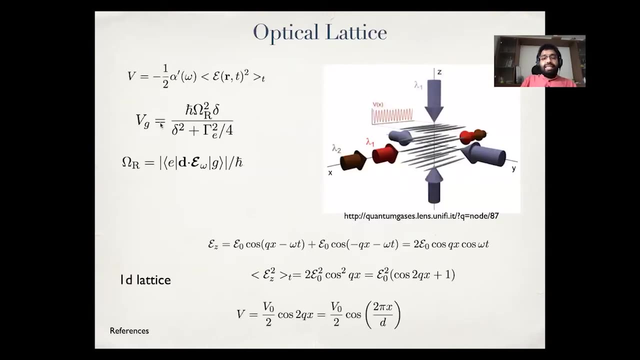 And basically, if I set gamma to zero, my potential just becomes h bar omega squared by delta, and omega squared has a magnitude of the applied electric field and also the position dependence of the applied electric field. okay, So the entire idea is: as soon as I apply an electric field, 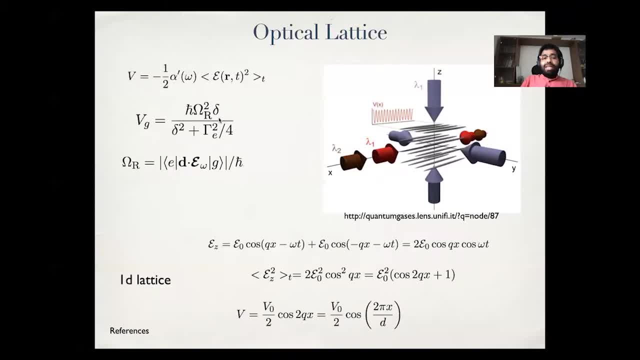 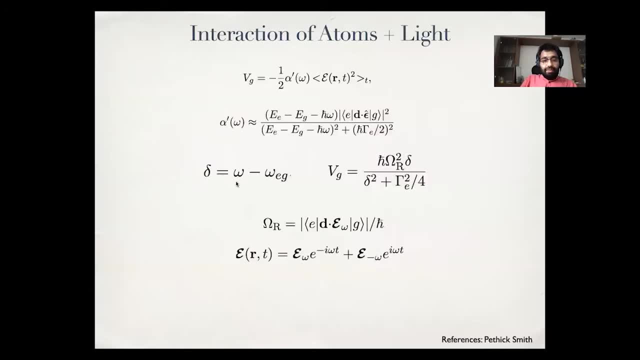 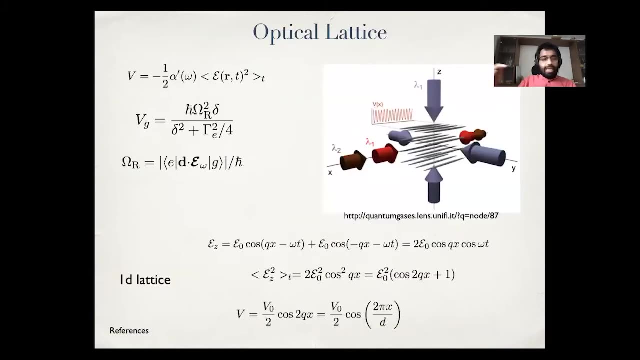 that is, if I have an electric field applied, it produces for me in this limit once my detuning delta, which I have defined here as the difference in frequency between the resonance frequency of the atom and my applied laser frequency. okay, So if I apply lasers of slightly different frequency, 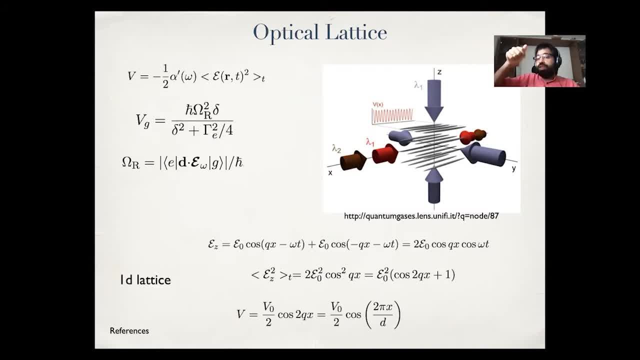 in fact significantly different frequency from the transition, so that absorption is not so important. the light fields, applied light fields effectively, give me a conservative potential whose shape is set by the position dependence of the applied electric field. That is the idea that one exploits. 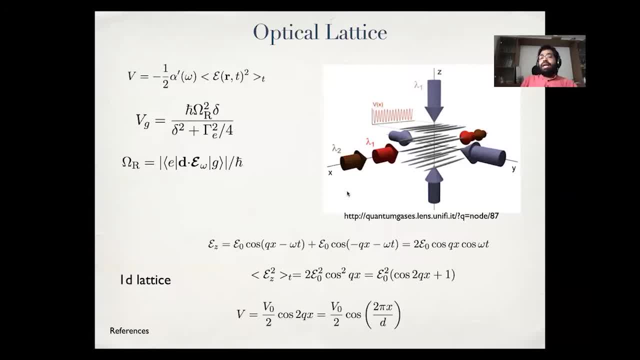 to make a so-called optical lattice, which is simply applying a standing wave of light and atoms, essentially because of the fact that this is a standing wave. let's just consider a standing wave in one dimension And it takes this form Once you do the time average. 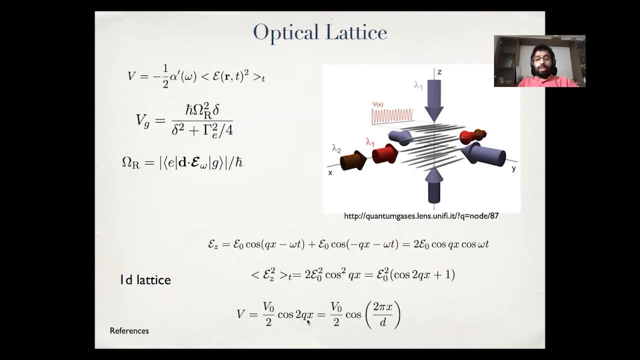 this standing wave basically gives you a position dependent potential, or a potential that has exactly this form. So it gives you a position dependent periodic potential with the periodicity precisely set, in this case by the half of the wavelength of the applied light. Okay, So that's 1D, but of course, 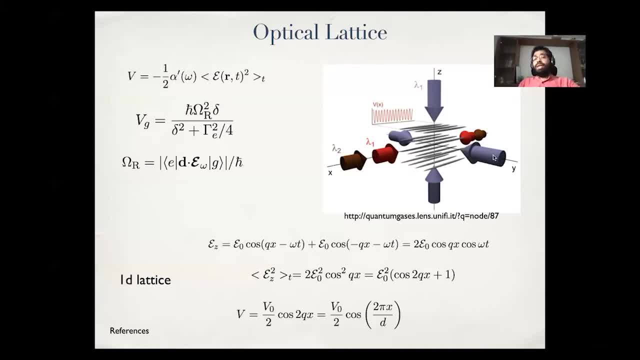 what stops me from going to multiple dimension? I can basically apply lasers in all three directions and I can make three-dimensional lattices, two-dimensional lattices, lattices with all sorts of crazy geometries if I want to simulate condensed matter systems, and so on. 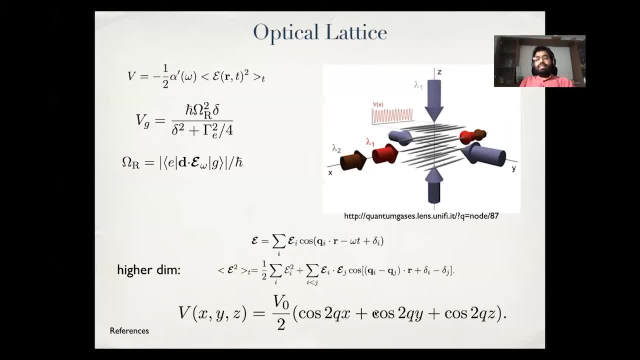 Okay. So this is an example of a three-dimensional lattice. For example, if I apply three lasers, I can- sorry, six lasers and make three standing waves or larger standing waves. okay, So that's 1D If I apply even three dimension. 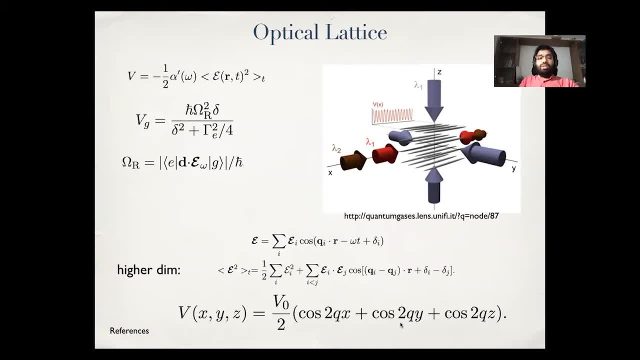 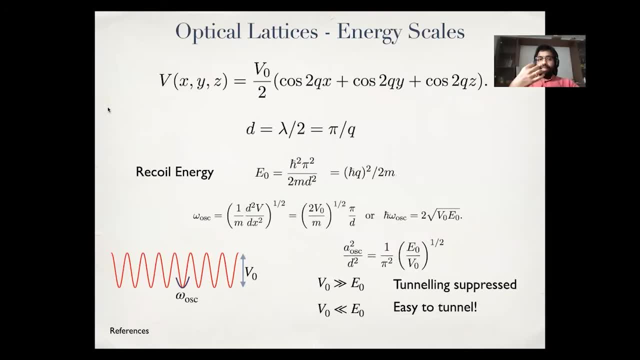 I can get a potential of this form, okay. So now the idea is, at the end of the day, once I have understood the quantum optics, of how to produce an optical lattice for my atoms in the ground states, which is the state in which I make. 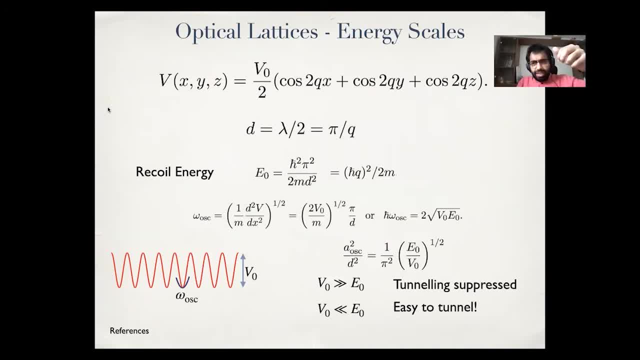 my Bose-Einstein condensate in in this ground state, meaning ground state of the two-level system. So in this ground state I make, all the atoms are in a Bose-Einstein condensate and this Bose-Einstein condensate. 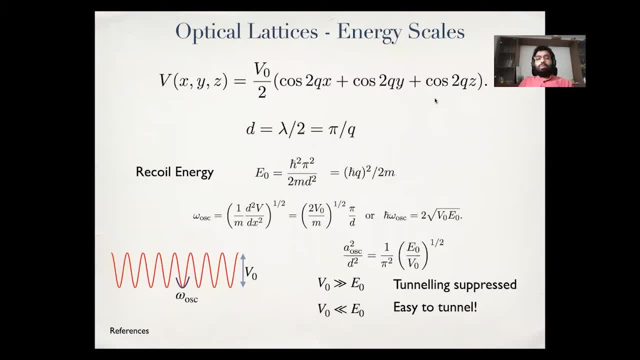 and this atoms basically see a periodic potential in space. So this optical lattice is just a light-induced periodic potential for quantum mechanical atoms. okay, That is the main thing to take care of. Now let's think a little bit about the energy. 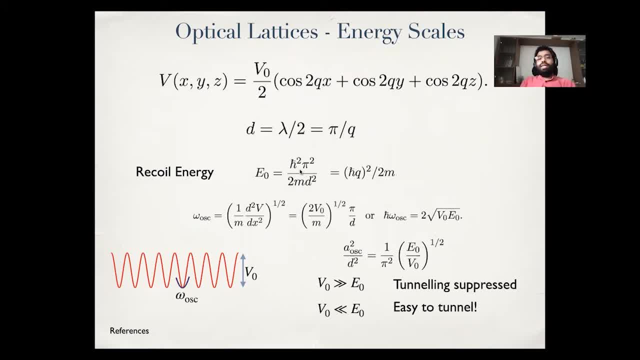 different energy scales that occur in the atomic case. So one energy scale is basically the one can think of it in two ways. One way is basically, if I have a laser that has photons of momentum Q, basically if I have a laser that has photons of momentum Q. 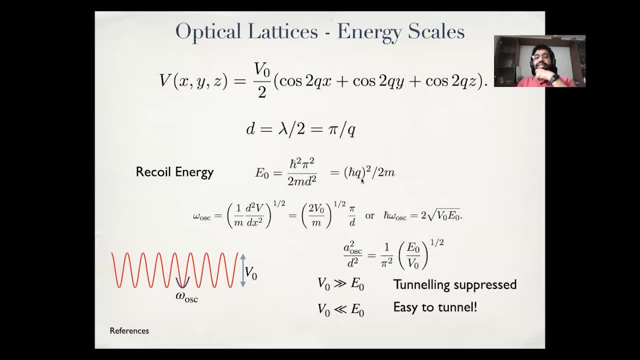 which is related to the periodicity of my lattice. this, basically, is the recoil energy. It is the. if I absorb a photon of H bar Q, my atom will feel an energy change of H bar Q whole squared by two M. So this is called the recoil energy. 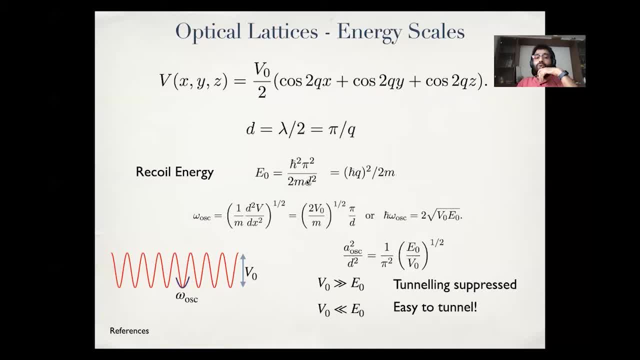 Also in another way. this is also telling you how localized, in some sense, is your lattice spacing, So as in how tight is your lattice. So this D it, it. it also gives you a sense of the lattice constant. okay, 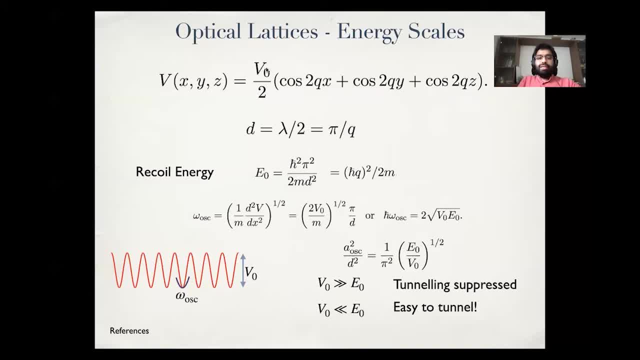 So now what one can do is to understand what is a big or a small lattice. The idea is that the ratio of the applied potential in units of this recoil energy really tells you if the potential you've applied is how big a potential barrier it is. 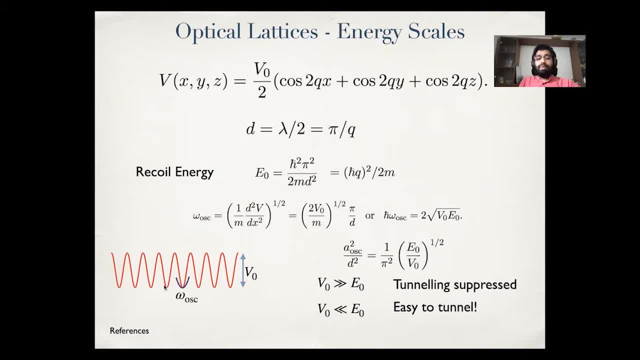 If you want to say that, if you think of quantum particles tunneling in this landscape, how well they can tunnel, that is in a sense set by the barriers And you can actually understand that by seeing the ratio between the applied potential strength to this recoil. 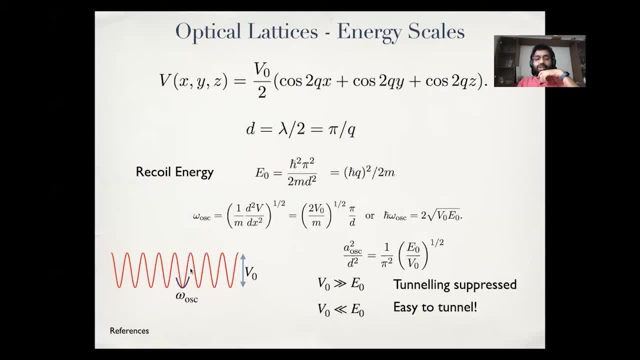 The way to see that is, I can, roughly speaking, I can think of at the bottom of my wells, I can think of as though I have an oscillator potential with the second derivative of the applied potential, which is actually nonlinear, and it has this cosine form. 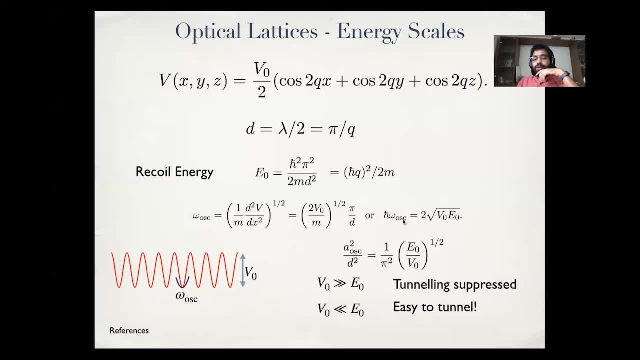 but at the bottom it's like an oscillator And it gives me some oscillators. It gives me some oscillator frequency. Now, if I take the ratio of this oscillator, the oscillator length implied by this oscillator frequency, which tells me the extent of the wave function, 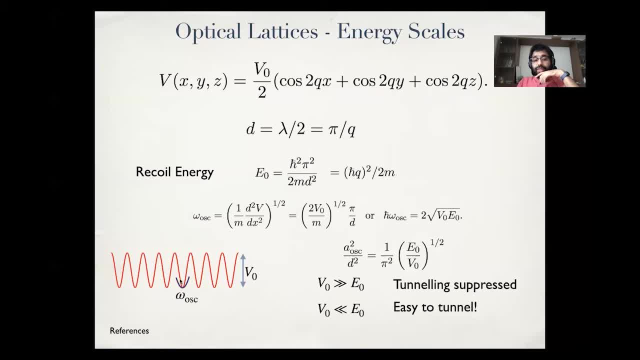 when I put an atom at the bottom of this well to, basically the separation to the next well, D, that is precisely given by E zero to V zero. So now, if V zero is much, much greater than E zero, the extent of these individual wave functions. 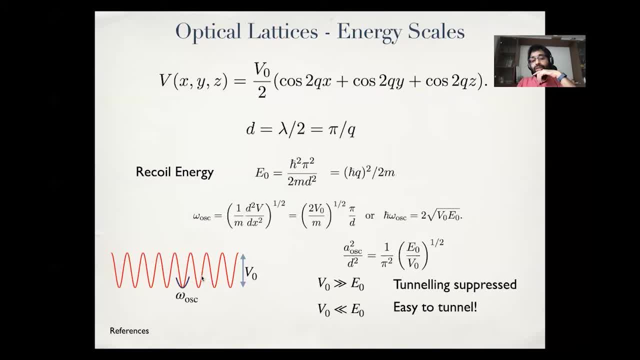 are going to be really tiny right And I cannot get enough. tunneling to the next. well, But on the other hand, if V zero is much less than E zero, opposite happens and my wave functions are delocalized and the atoms can basically move freely in the lattice. 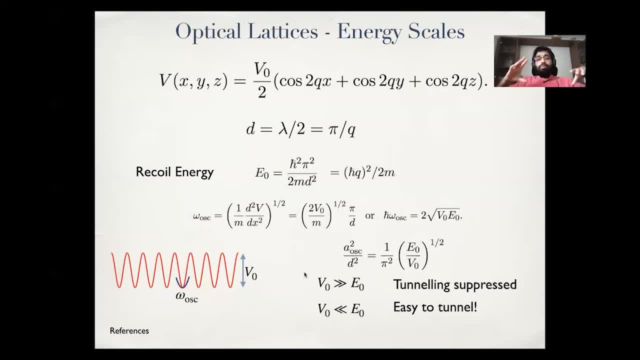 So a large lattice strength means the applied potential V zero is much larger than the recoil energy of the atoms, and so on and vice versa. okay, So that's just to give a sense of the energy scales in an optical lattice. okay, So now. 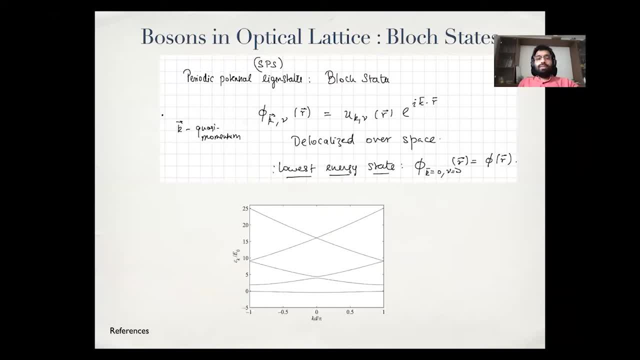 I'm slowly moving towards this description of this Mott-insulator superfluid transition for which we have to understand a little bit the quantum single particle states of quantum particles in periodic potentials. We've already understood it for free space, which is plane waves. 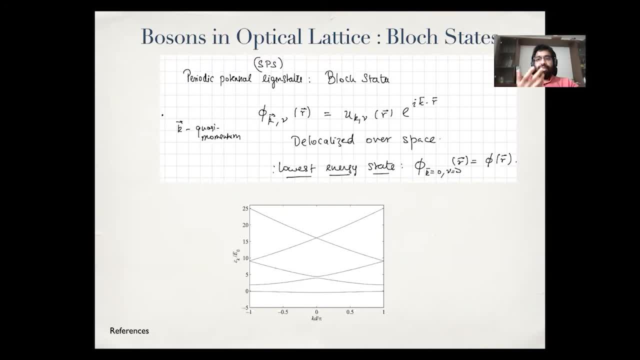 Let's just quickly revise. I think some of you might have already seen this in condensed matter courses. So the eigenstates, for example in an periodic potential- this is in 3D- are given by these block states. These have this very nice property. 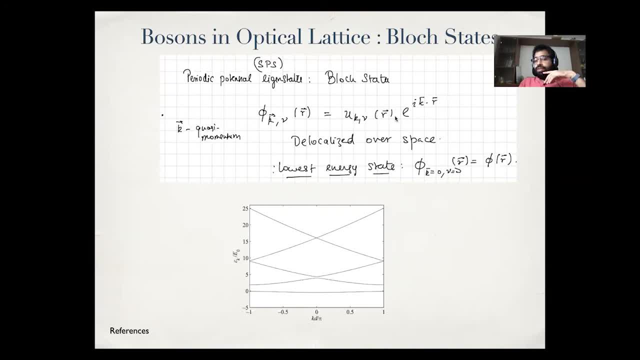 that they are a plane wave times, a periodic function. It is periodic in the lattice parameters, So if it's cubic lattice it is repeated over AAA, the size of my lattice constant, or D here as I'm using, And of course these are energy eigenstates of my system. 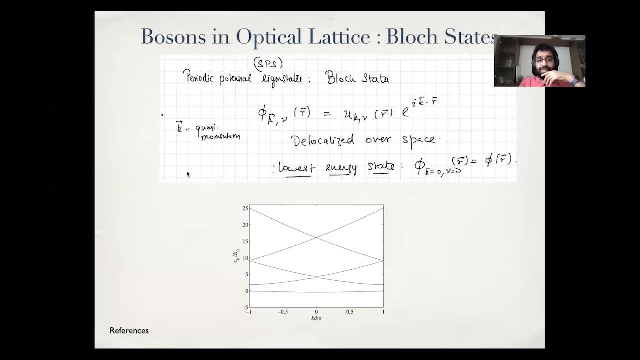 And so the lowest energy eigenstate has quasi. this K is called a quasi-momentum because this is not perfectly plane wave, It's not a momentum in that sense. So it's not a momentum in that sense. But so the lowest energy state has K equal to zero. 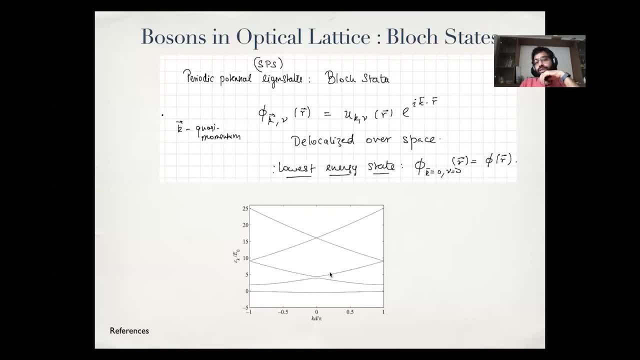 and there is another index, mu, which tells me what is the band And one can just specify. this quasi-momentum is a special kind of wave vector which is unique only in minus one to one, in the sense that it goes from minus pi over the periodicity. 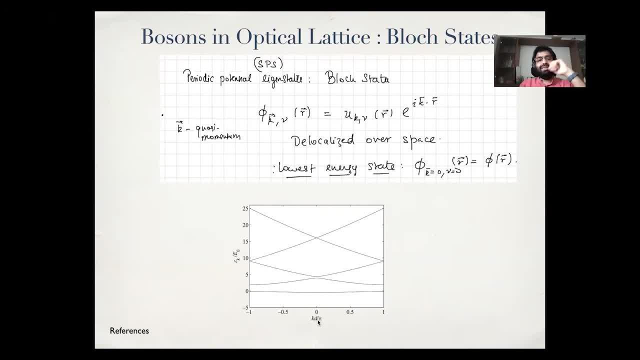 to pi over the periodicity for a 1D system, which is the reciprocal lattice Which is the size of your first Brillouin zone. So beyond that it is basically repeating. And this repeating things you can fold back and make a picture that's called a band structure, right? 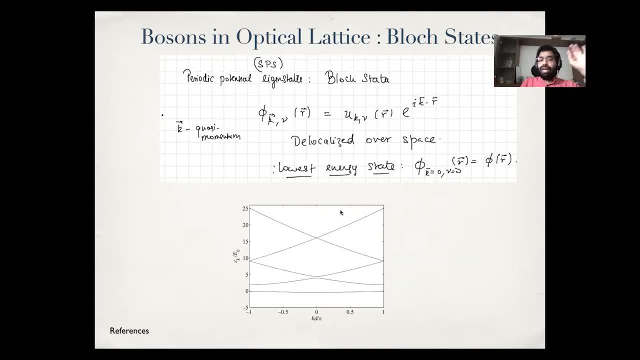 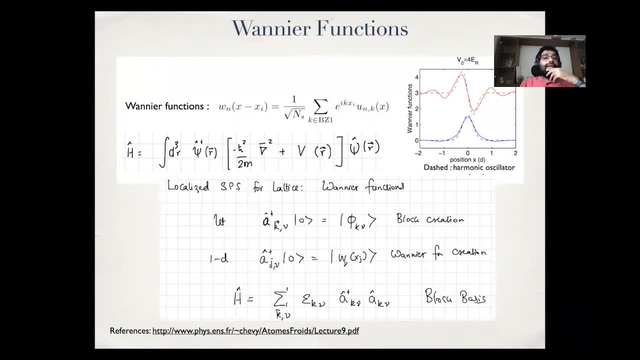 So this is just the one dimensional band structure. This is how the energy eigenvalues of a single quantum particle in one of these optical lattices is going to be okay. Now, this is one kind of basis functions into which our many particle system can occupy. 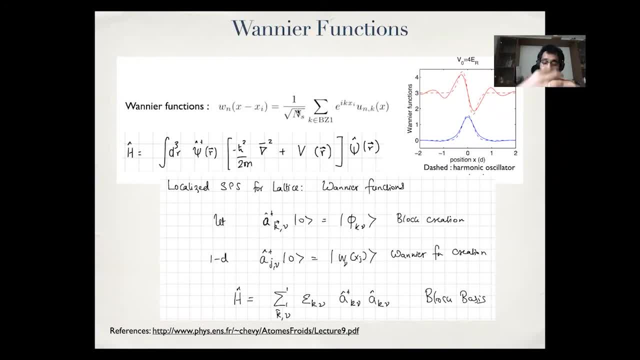 but a more sort of another, different basis that is very useful in discussing the physics of a mod-insulator. superfluid transition is the situation where I take basically a Fourier transform or a sum over many block functions. When I do that, because these block wave functions are delocalized in space. 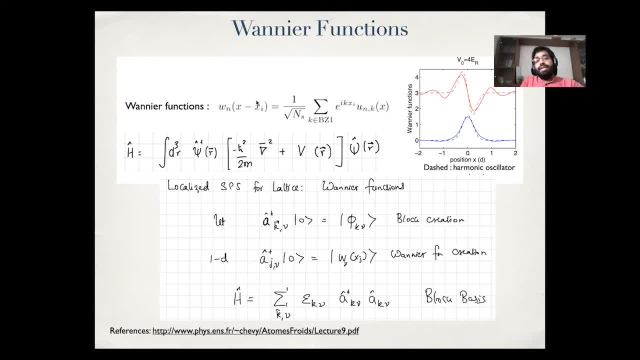 their Fourier transform gives me localized wave functions And basically these wave functions are called the Vanier functions. And these Vanier functions are, depending on the strength of your lattice. they can be very strongly, strongly localized, at the minima of my potentials. 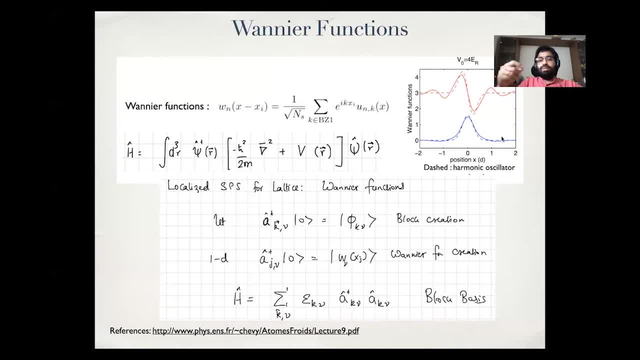 which I'm going to call as sites of my lattice right. So these are the minima of my lattice, minima of my optical lattice potential. Now, if I write down the many body, Hamiltonian or just quantum, multiple quantum, non-interacting quantum particles in a periodic potential, 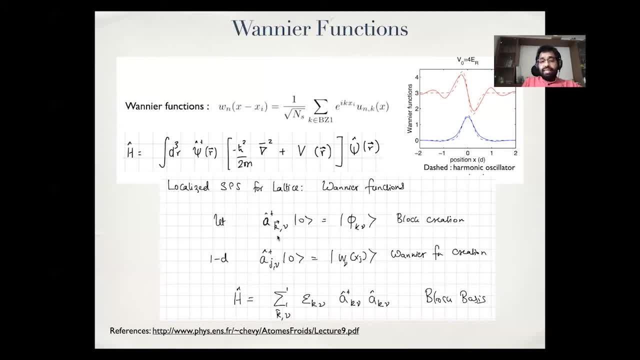 V of R, given by some periodic potential. I can essentially write it down in terms of creation annihilation operators to create or annihilate atoms into blocks right. So I can essentially write it down in terms of creation annihilation operators to create or annihilate atoms into blocks right. 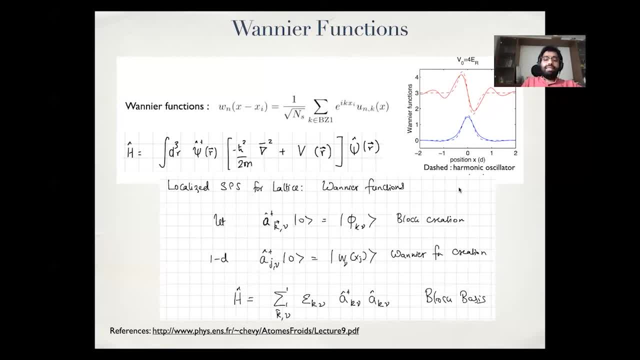 So I can essentially write it down in terms of creation, annihilation operators to create or annihilate atoms into blocks, right. Or I can basically occupy lattice side by side. So either way, I can write down this Hamiltonian in either basis right. 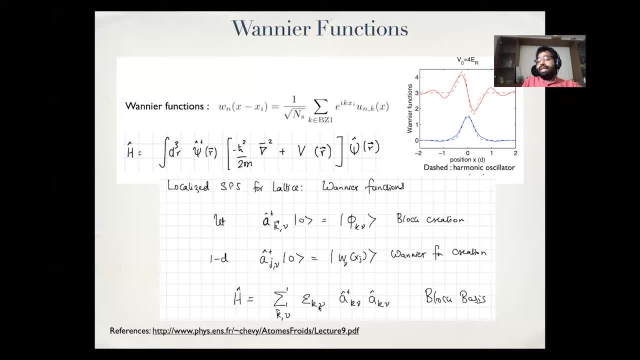 So if I write it in the block basis, of course this is completely diagonal. E K nu is basically the energy levels that I have here, And A dagger K nu. A K nu is just counting the number of atoms in such states. okay, 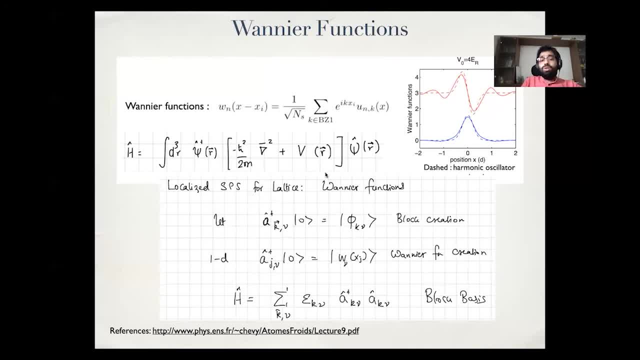 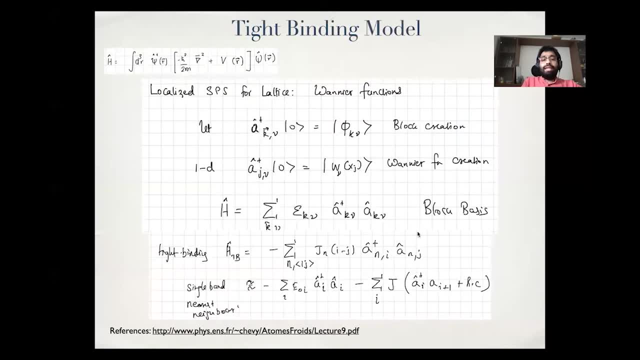 That would be Hamiltonian. But on the other hand, I can also write this Hamiltonian in the Vanier function basis, And when I do it, if I write it in the Vanier function basis, I get this very well-known version of the Hamiltonian of particles. 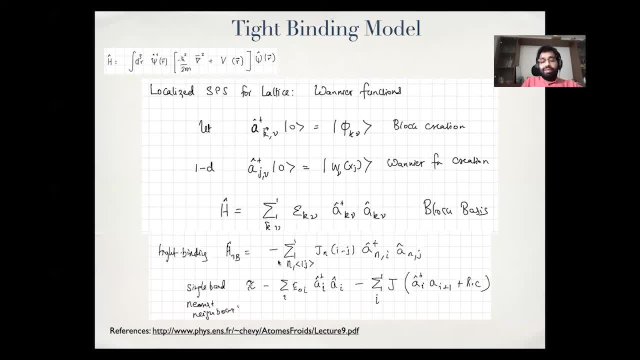 in a periodic potential called the tight binding Hamiltonian. After a little bit of simplification, this tight binding Hamiltonian really gives you the following sort of picture: It is just: each individual well, has some energy and you have a sum over I with A I dagger, A I plus one. 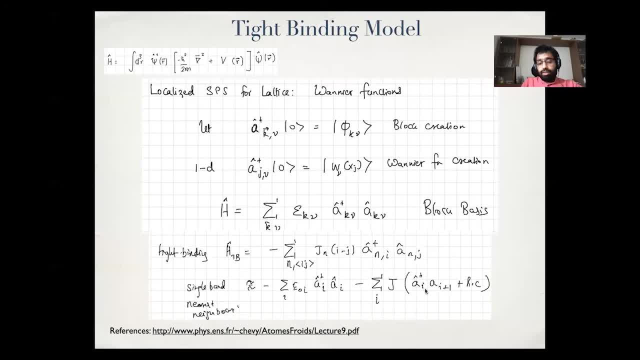 A I dagger, A I plus one, A I dagger creates an atom at the position I, the minima I-th. well, of your lattice, I plus one and I different I's are like that. So now this term precisely talks about tunneling. 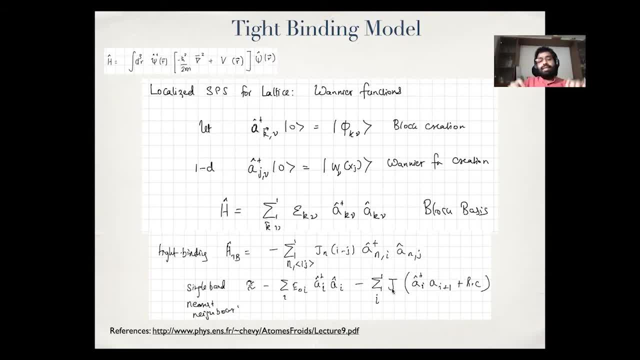 of the atoms between different sites of your optical lattice. And J is the tunneling strength. Typically, once I make my V one, two recoils I can safely cut off. in principle I can tunnel because I have the localization. I can tunnel from site one to site 10 or site 20, far away. 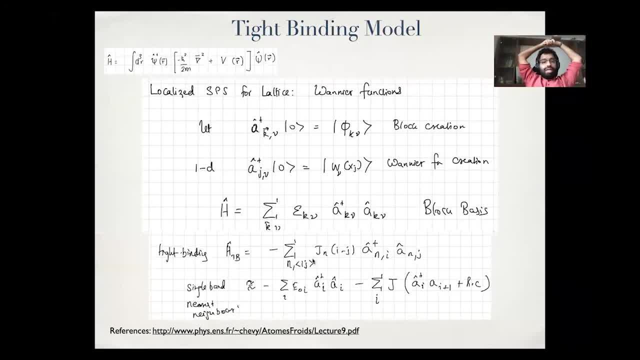 But once my potential strength is large enough, only nearest neighbor tunneling is enough, And that is why I have written it as A I dagger, A I plus one, And I can also restrict the physics to a single band, because the higher bands are at a different energy. 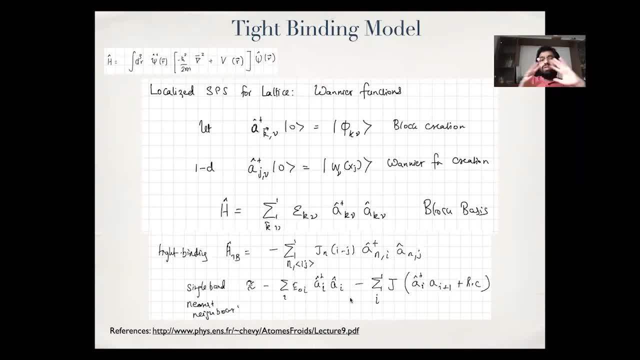 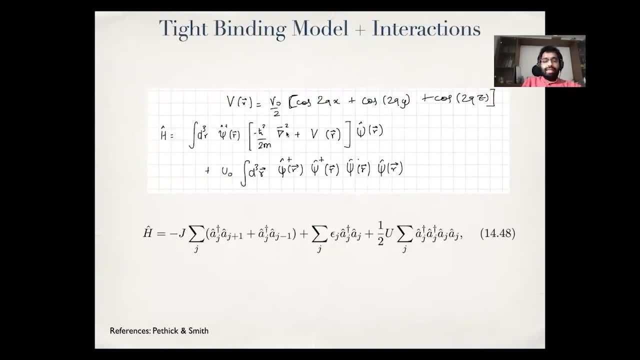 and I'm always going to be in a single band picture. So this is the physical description of, basically, atoms in an optical lattice. Now, if these atoms are bosonic atoms and they have this contact interactions, okay Of course. now I have to plug in this psi. 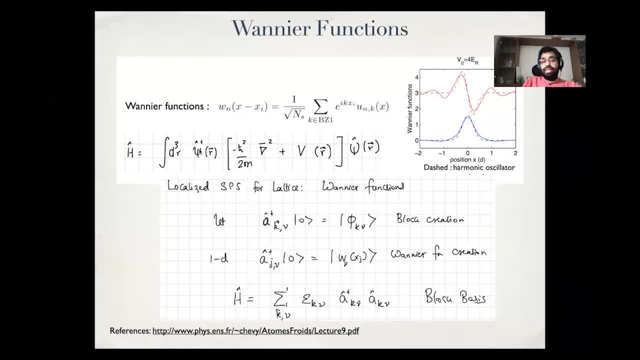 that I was writing here in terms of. originally I was writing psi in terms of just these: let's write psi, expand psi in the Vanier creation operator basis. And when I did that, I got the tight, binding model when there were no interactions in my Hamiltonian. 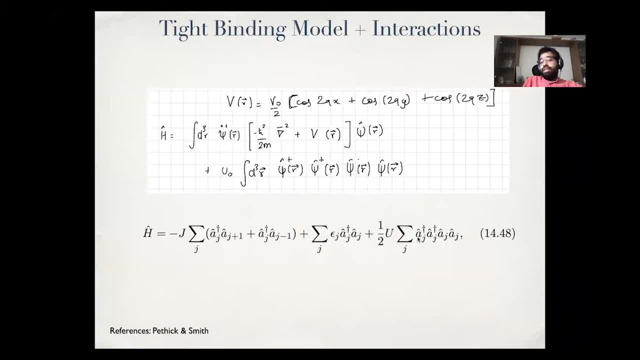 Right Now, if I have interactions like this, I also get this extract term that describes my interactions between the atoms. okay, So now this is the Hamiltonian that describes an interacting bosonic system on an optical lattice. okay, And this is called the Bose-Hubbard model. 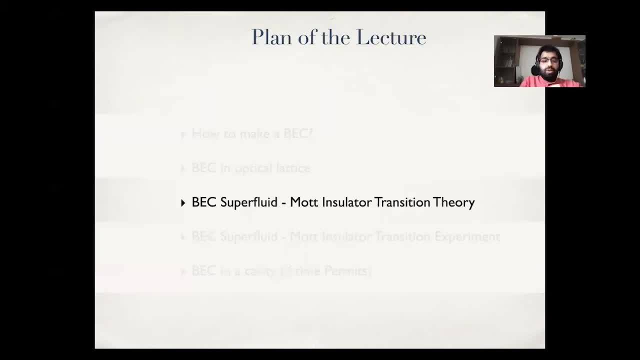 All right, okay. So now, before I go on and talk about the prop, talk about this Bose-Einstein condensation superfluid-Mott insulator transition. if there are questions you can ask me now. Okay, they're asking questions in the chat. 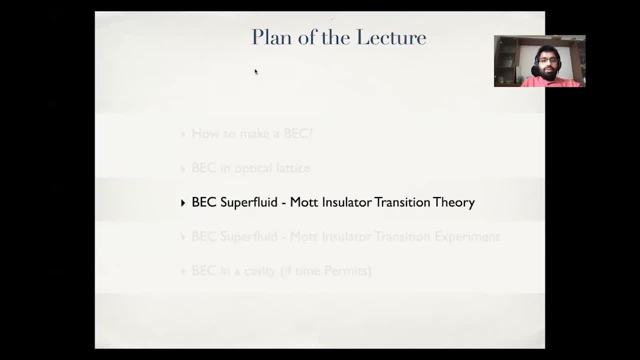 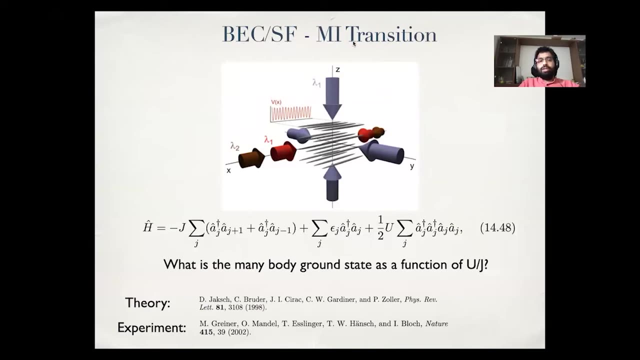 I have a problem? Huh, okay, good, So, since there are no questions, let's move on and study this: properties of this Bose-Einstein, of this Bose-Einstein, condensation. Okay, so, the main question. one asks the central question of the superfluid-Mott. 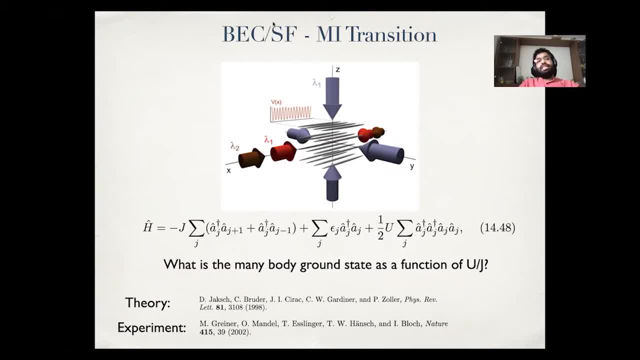 interlacer transition and or okay, So why am I writing this as BEC superfluid-Mott insulator transition? I'm just trying to not be disingenuous because I haven't really talked about superfluidity in detail in this series of lectures. 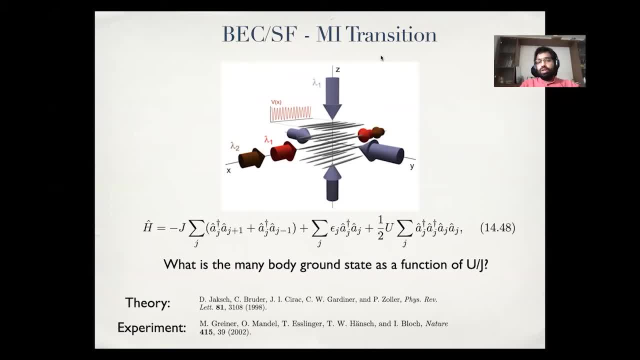 For our purposes, I'm going to interchangeably use the concept of a BEC with a superfluid. Any BEC that you make with interactions between them, between atoms, will give you a superfluid, basically okay. So with that caveat, 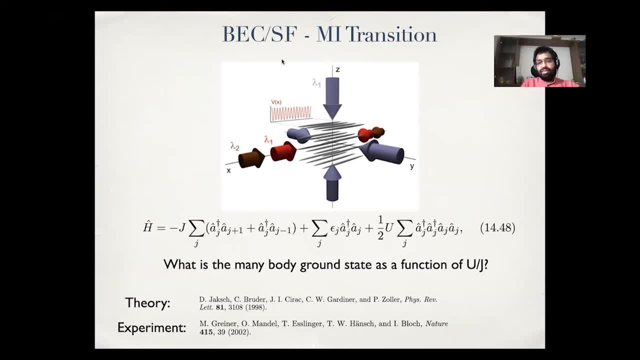 that's why I'm going to call this superfluid. But whenever I'm saying superfluid, imagine that I'm talking about a Bose-Einstein condensate. Okay, so we are interested. what is the main question in this superfluid-Mott? 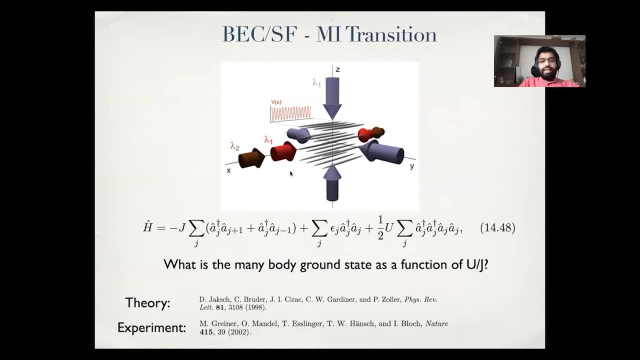 insulator transition business. The idea is to take a Bose-Einstein condensate in an optical lattice and then ask the question: what happens to the many body ground state of these atoms? as I make The interaction between the atoms stronger and stronger, 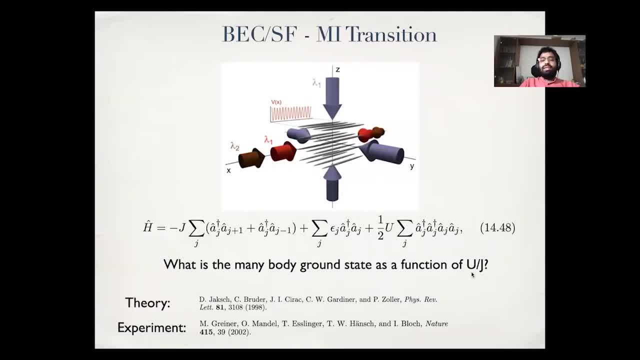 and stronger compared to the tunneling strength right. In principle. the way one does that is, you can make the tunneling strength larger and larger and larger, sorry, smaller and smaller and smaller by making the lattice deeper and deeper right. So effectively you can boost the interaction strength. 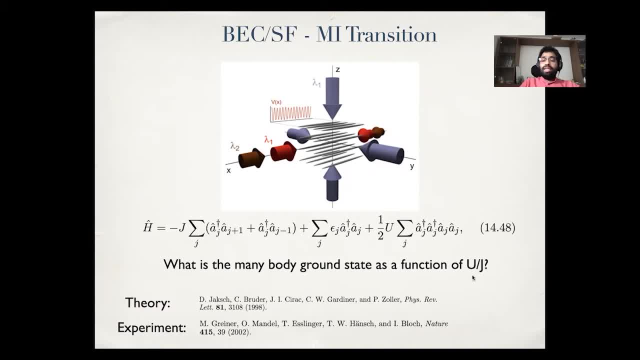 with respect to the tunneling by making that happen. And then one can ask what really happens to my many body ground state? Of course, something interesting happens. That's why we are asking this question And we will now explore the theory behind what happens. 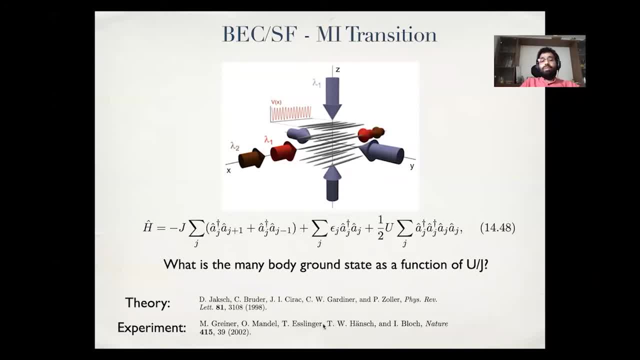 as well as this famous, as well as briefly examine this famous experiment from the group of Immanuel Block in 2002, Immanuel Block and Ted Hench in 2002.. And the theory, of course, was from Eta-Jacks and Zoller in 98.. 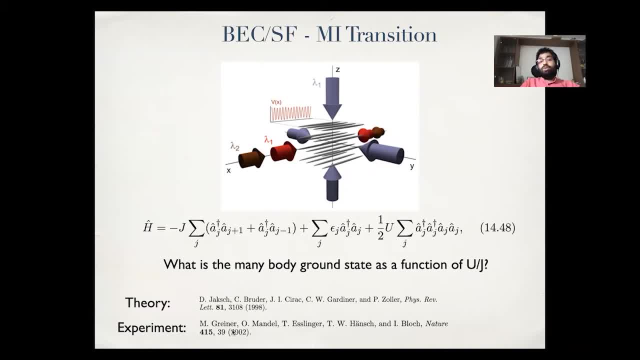 So the theory was proposed in 98, and the experiment was done in 2002, which is again one of the most heartening experiments, which is again one of the most heartening experiments, which is again one of the most heartening experiments. 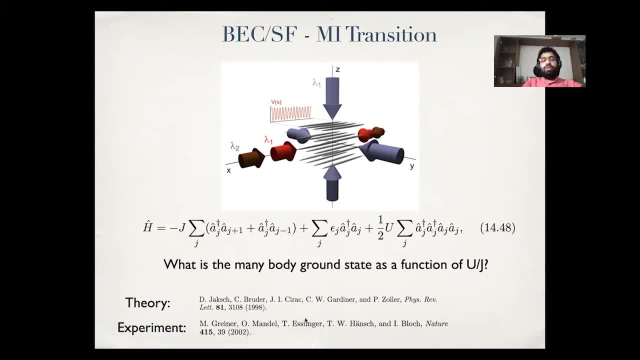 the very beginning features of this entire field of ultra-cold atoms of ionochrome condensate. So basically, this was proposed during the PhD of Eta-Jacks, I think, And then it was implemented essentially almost by the time he finished his PhD. 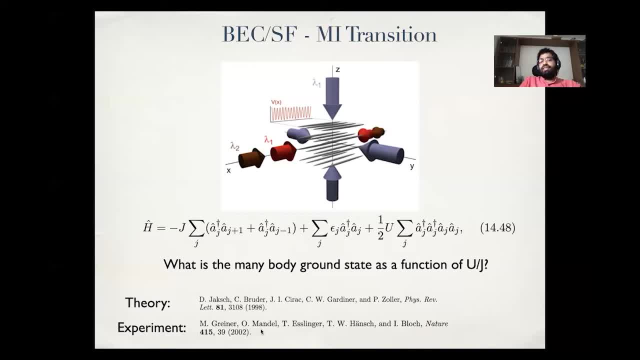 or when he was in his postdoc- which is very rare in theoretical physics that you propose an idea and then it gets implemented. But in this ultra-cold atoms, there is a hope for that, And that is really one of the most driving forces. 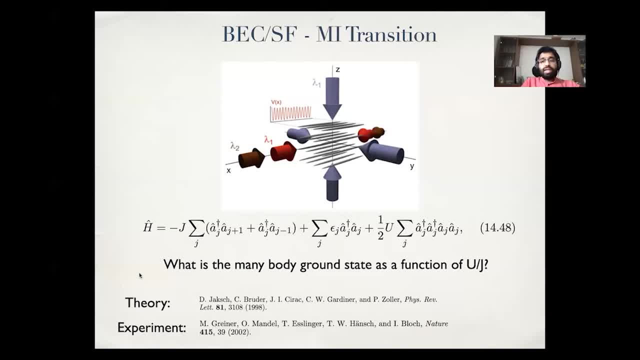 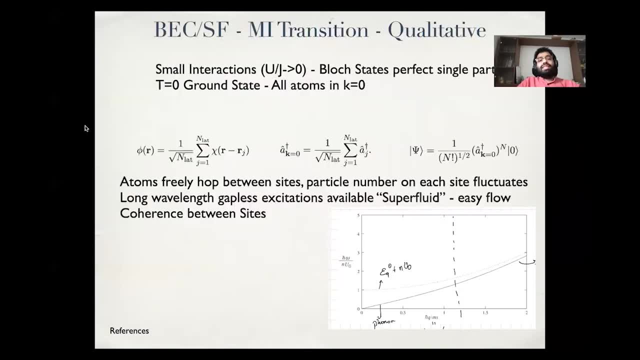 for why this is really exciting. OK, for a theorist, that is one aspect that is very interesting, right, so that your theory can be realized in an experiment. okay, so let's examine what happens. so now, if i am in this, let me qualitatively understand why i expect the- uh, the state of my system to be very different for small. 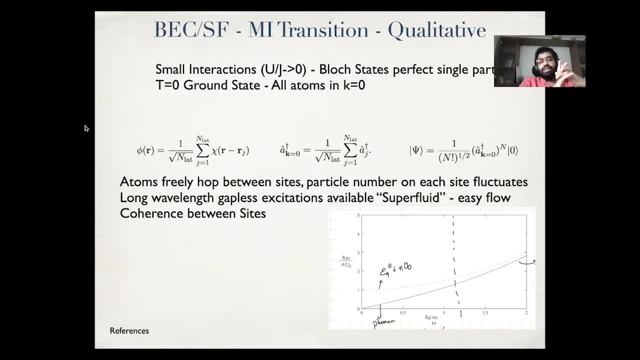 versus large interactions, or for small u over j versus large u over j. so let me look at this first, this extreme limit where essentially u is zero, so my tunneling is is very large, so i just have a lattice very nice uh with some weak uh lattice strength, so my u is practically zero compared to 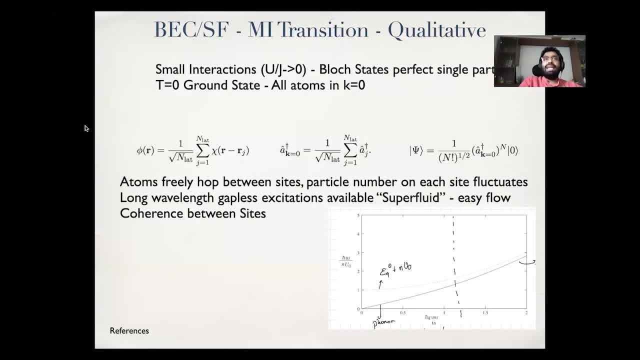 the tunneling strength. right, so the tunneling strength is larger. if my lattice depth is smaller, okay, keep that in mind in this limit. it's very simple. we just talked about this- is exactly the non-interacting limit of bosons in an optical lattice. and if 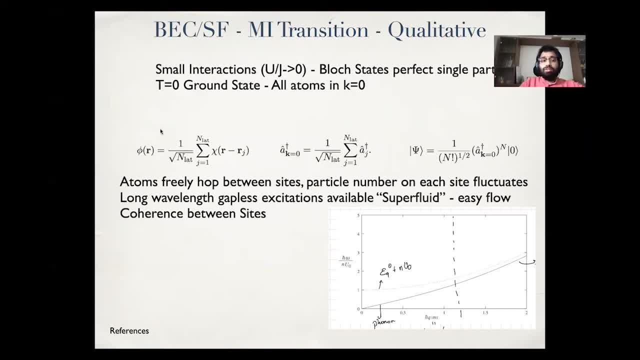 i am in this extreme limit where essentially u is zero, so my tunneling strength is larger. i make a boson stand condensate. of course all of my atoms in my boson stand condensate will occupy the same, uh, single particle state, in this case the single, the single particle state. 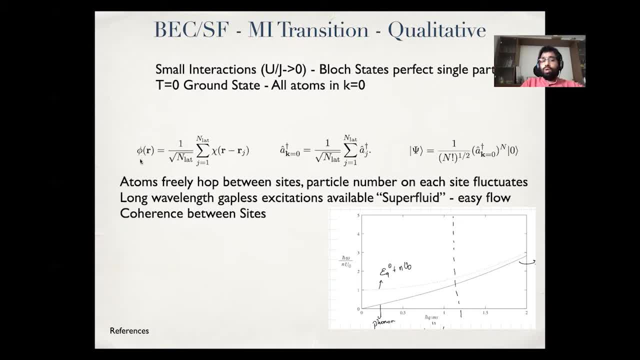 which is the ground state, is a block state of quasi-momentum zero, which is represented by phi of r, and this is given by a superposition right of different vanier functions which are the localized functions at the lattice sites of the atom of the lattice which are localized. 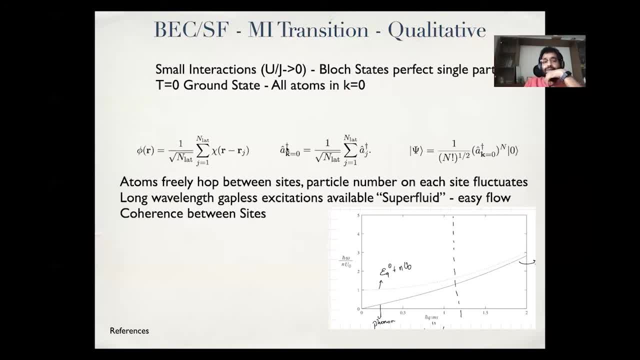 at the minima of the lattice and that is a. basically, if you write the creation operator- creation operator- corresponding to this block state, it is a superposition over different localized operators, right, and then what we are saying is: in this regime, our atoms are going to be in a boson stand, condensate, with all atoms occupying uh, a delocalized uh atomic wave on my. 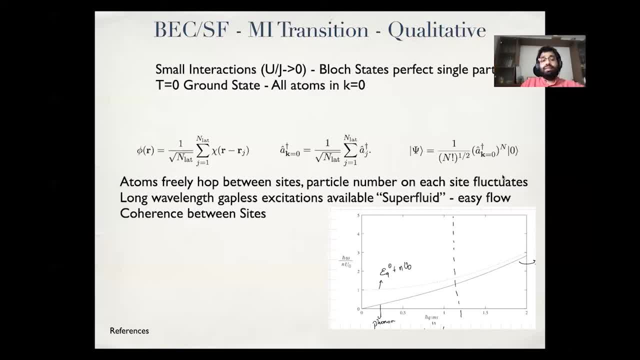 optical lattice. so this means that basically atoms are going to be in a boson stand condensate state. for me, atoms can hop freely between the. so everything is described by a BC wave function. but the BC wave function is now a block wave And hence there are no fixed particles on each site, If I 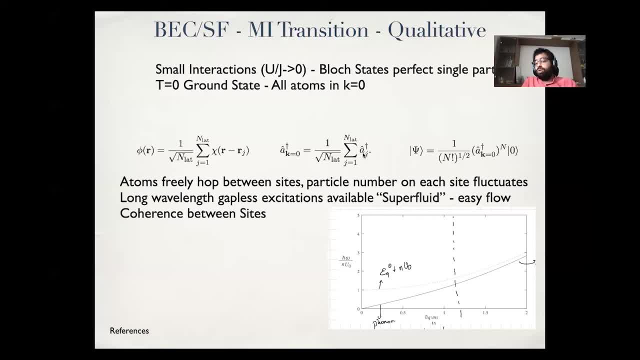 look at the fluctuations of individual particle numbers. so AJ dagger, AJ squared, that will not be, that will basically there'll be large fluctuations of that. And the second aspect, because I have essentially a Bose-Einstein condensate, the reason why one calls this: 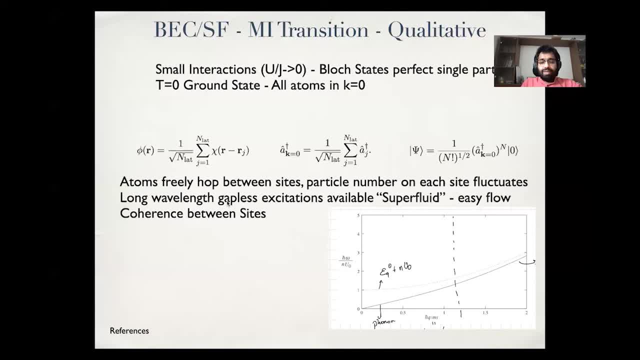 superfluid, in a very nutshell way, is to go back to what we studied yesterday, which is the excitation spectrum. This was for a uniform gas, but for a very weak lattice it is almost like a uniform gas And what we see is that when you look at the excitation of such an uniform Bose-Einstein. 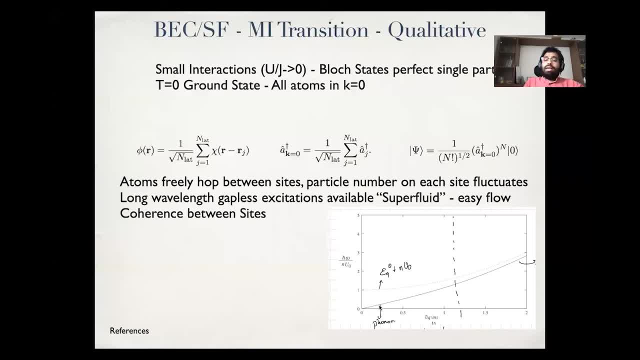 condensate the excitation spectrum. there are excitations available at very small energies and essentially very long wavelengths, which means I can excite my system and actually the system will accommodate an excitation at essentially zero energy. At the end of the day, you can think of superfluidity as basically 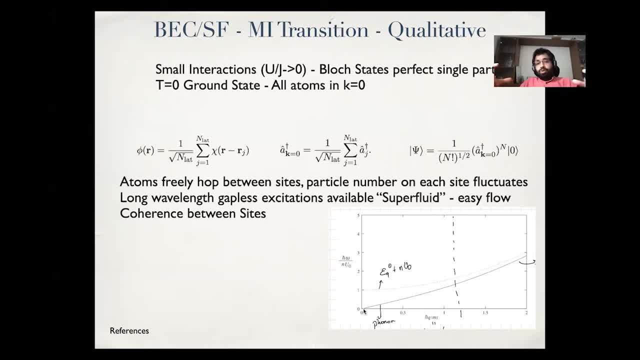 something like this, where my Bose-Einstein condensate: if I allow it to flow, it will flow without any resistance, Because I don't need to provide any energy for it to move. Even at very long wavelengths I have motion. And the other idea is that excitations are all of very long wavelength, meaning I have 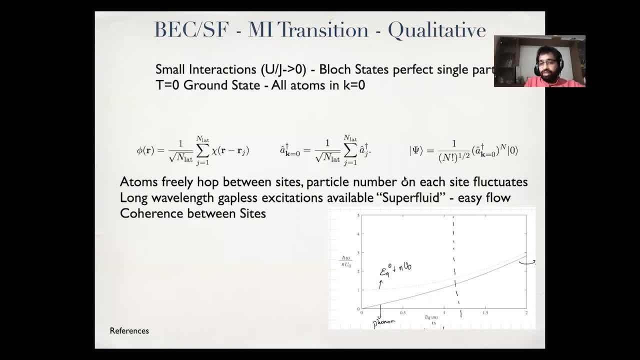 essentially coherence between different sites. That coherence between different sites one can also understand it as basically from this operator which is creating basically a superposition over many localized states. So these are all the features that tell us at very, very small distances. So if I have interaction, strength and large tunneling, I have a Bose-Einstein. 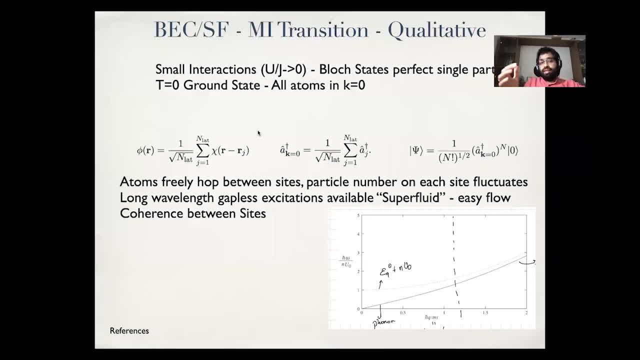 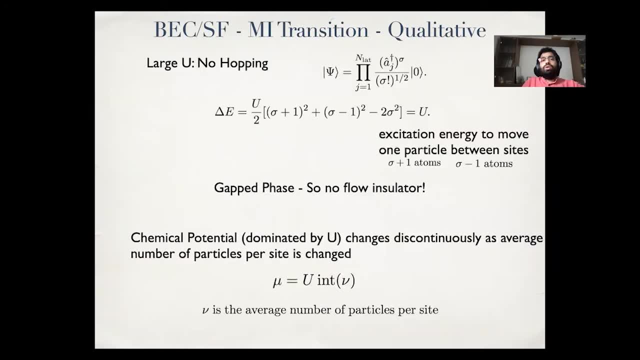 condensate or a superfluid. So if I keep these atoms in this state, they will flow without resistance. I haven't explained this in detail, but that's how it is Now what happens in this opposite limit. So let me go to this extreme limit, where I have made my lattice. 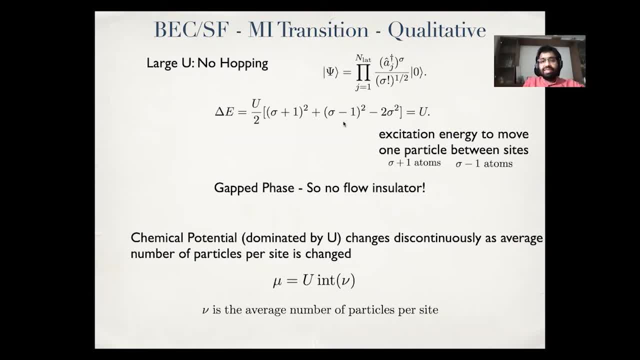 so strong that there is no hopping between different sites of my lattice, Then I know for sure that I have in some sense. I cannot have atoms delocalized between different sites, So I have to really tell how many atoms are there in each site. So the state for such a situation could roughly be like: 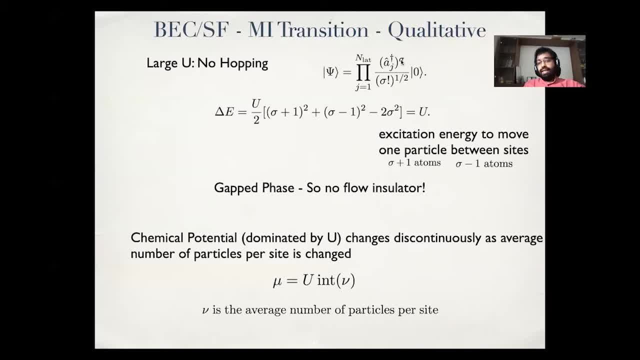 this. So in the jth site, in each site, if I have an atom number of sigma, basically my total state is basically of this form. So it is a j dagger to the sigma In each site, in each site I create. 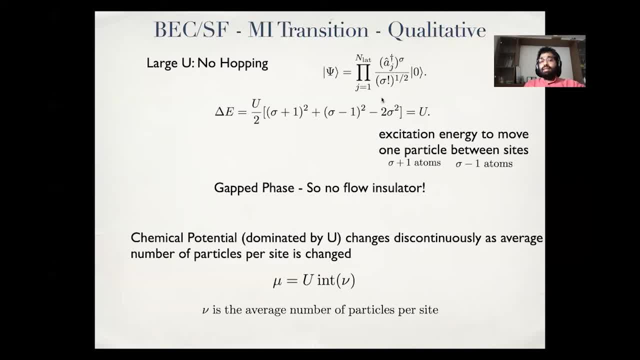 sigma atoms in the localized state. Now, this state, I want to show that this is kind of an insulating state or an insulator. How do I show that qualitatively? The idea is, let's ask, when I have sigma atoms, when I have this kind of situation where I have basically filled in each site sigma, 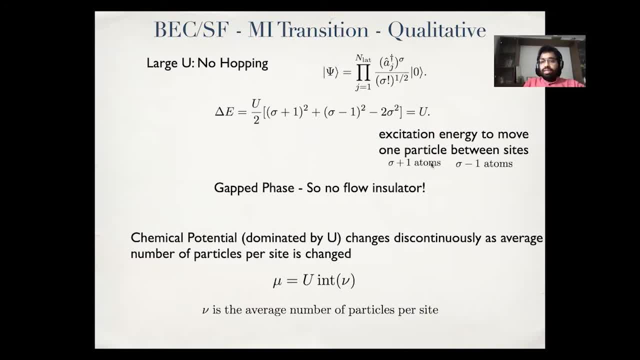 number of atoms. Now, in such a situation, if I have to make an excitation in my system, which means I want to move Basically one particle from a site with sigma plus one atoms to a site with sigma minus one atoms, right So that I can make each of them have the same number sigma of atoms, This is like an 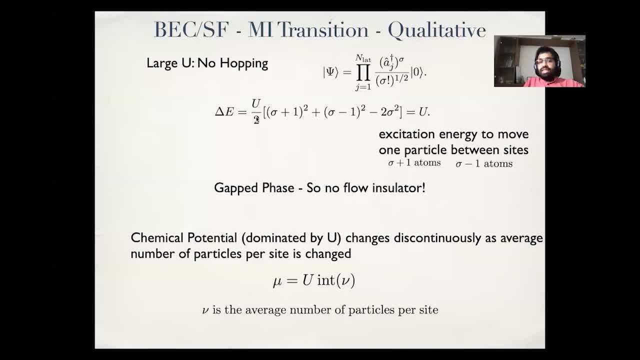 excitation in my system. Now you can calculate the energy of this excitation. There is no tunneling, It's only the interaction energy. You can calculate it. This is the situation before right, When I had sigma plus one atoms in one site, sigma minus one atoms in another site. 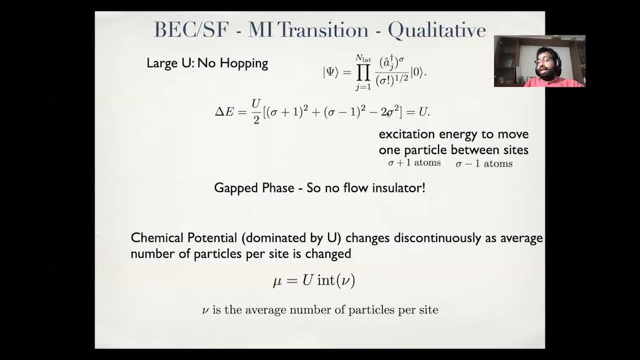 Basically did the swap And basically I have sigma in each site And then I take the difference: It is precisely U. So in this scenario, each excitation that I have to create on my many body state requires a fixed and in fact large energy U which is given by the interactions. This is repulsive And so there is no, I can't, I have to pay energy cost to put an atom. 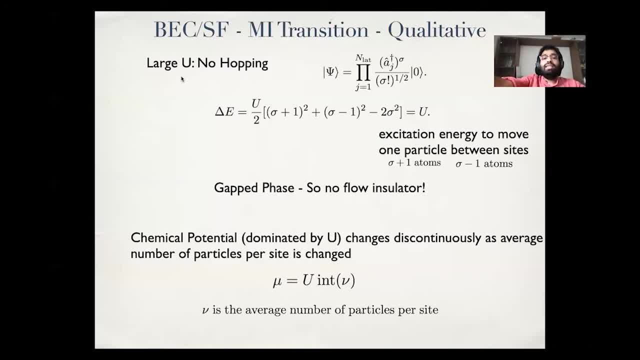 into a site that has atoms already. Okay, So, which means there is always a gap, that is, a gap in energy that is there, And if I basically make infinitesimal push to my system, it will not flow Right. So I have to give it energy that is over this U in order to get it to flow Right, And that is precisely what an insulator is. Okay, So now. 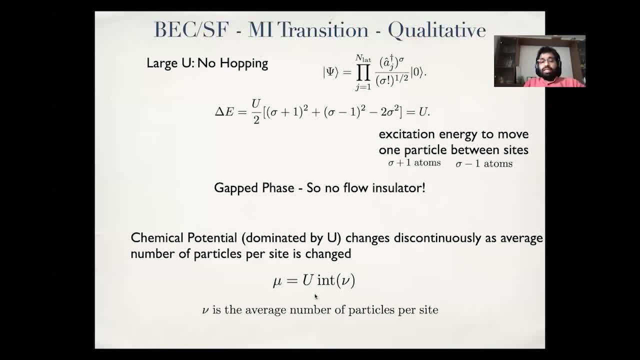 one can actually calculate what is the chemical potential in this system. I will just show this in a moment More in a more quantitative manner- And it turns out that it is basically proportional to U times the integer part of the average number of particles per site. Okay, 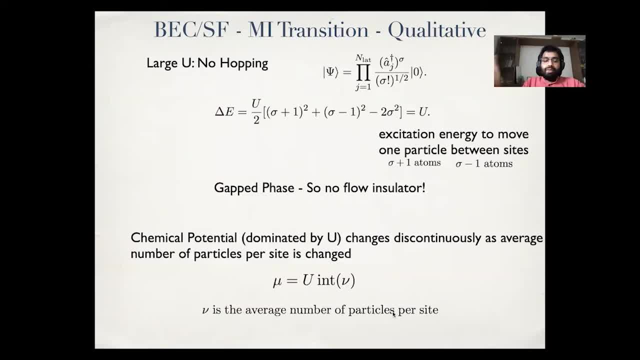 So it is basically: you calculate the total number of particles divided by the number of sites. that is the average number of particles per site. Okay, So let's so. that is the qualitative picture- tells us that extremely large U- I would expect a state like this- And at extremely small U and. 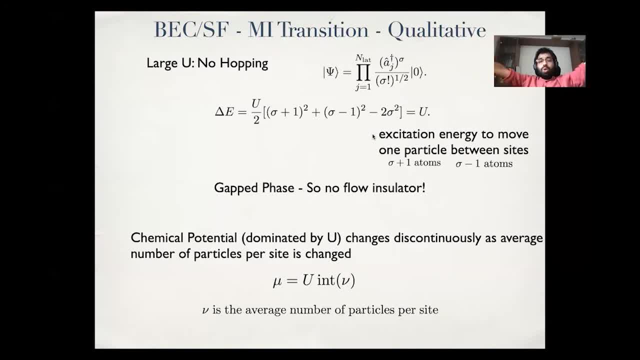 large tunneling. I would expect this superfluid, And these two quantum states are very different. quantum mechanically, This is an insulator, whereas that is a Bose-Einstein condensate with coherence And basically, as you change this J over U continuously, you will get a phase. 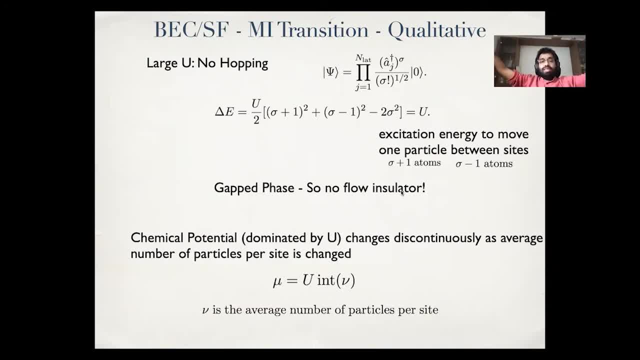 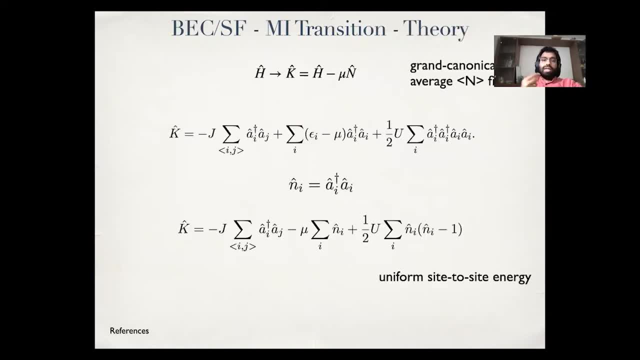 transition between these two very different, many-body states, which is this superfluid, not-insulated transition. So let's look at this in a little bit more detail. Again, I'm going to be somewhat wishy-washy here, I'm going to hand wave a bit, but that's the best one can do given the 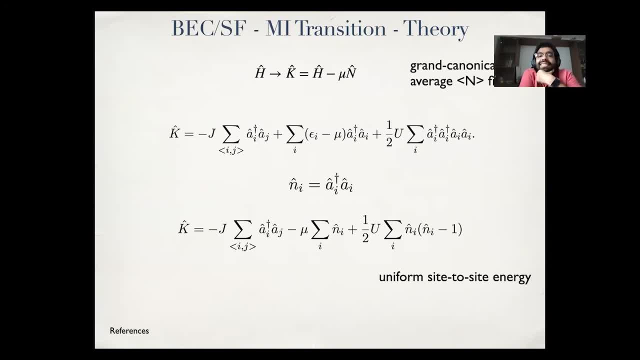 time. So now one thing we will do is, instead of analyzing the Hamiltonian and looking for the ground state, which is the point. So we want to look at the ground state of the system, as I tune this J over U, Instead of doing that with the Hamiltonian. 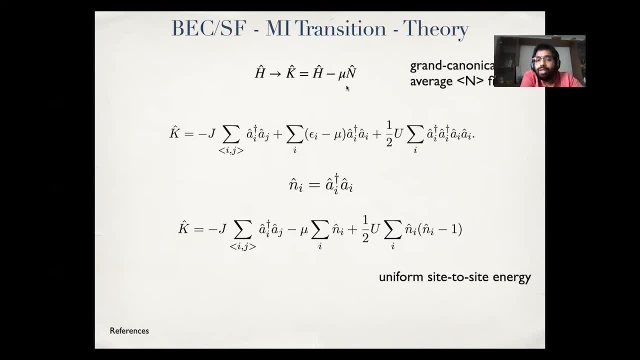 what is better here is to actually look at this grand canonical potential H minus mu n. Why is this useful? This basically says that we only have the average n fixed, And this is somewhat easier. I won't go into the technical details, but typically this is somewhat easier. 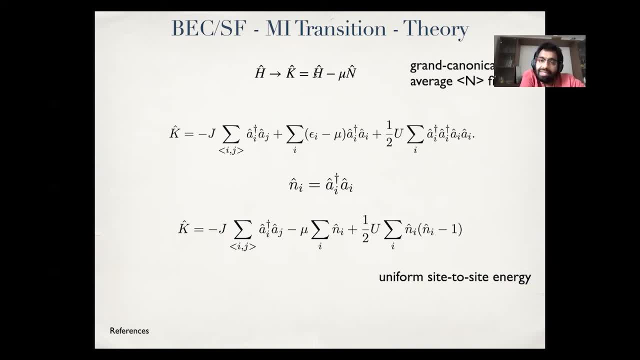 to analyze than the Hamiltonian, in which case you have to by hand always implement the constraint that I have the same number n of atoms, which is somewhat harder when you are calculating things. So, just as the thing that I remarked earlier With that, 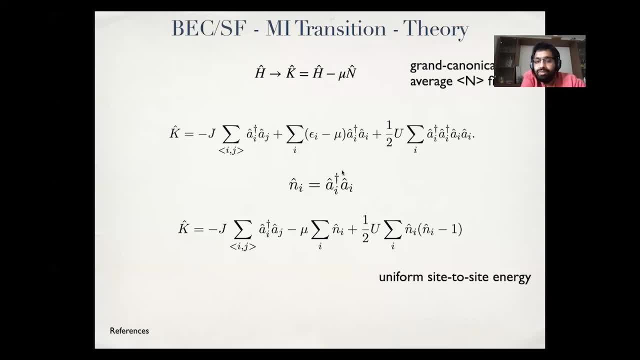 we have our, and then you can make a little bit of changes. Like, for example, when you write H minus mu n, you get something like this: And you can transform your interactions also into this simple form: ni times ni minus one. This is like density-density interaction at each site: ni is. 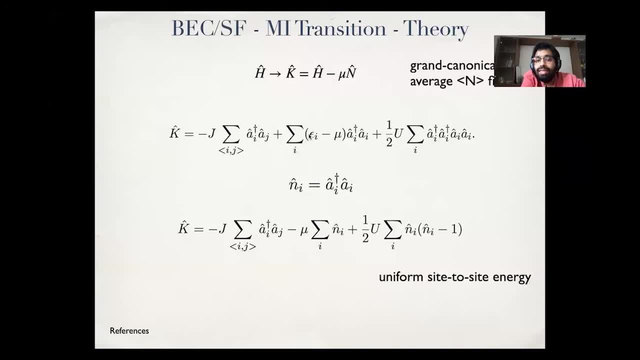 the number operator at site i. And then if you assume that basically all of my sites have the same ground state energy, which is fair enough. And then if you assume that I have a perfectly symmetric lattice, if I don't apply any external trapping potential over and on top of this optical lattice, this EI is same and it's just you can. 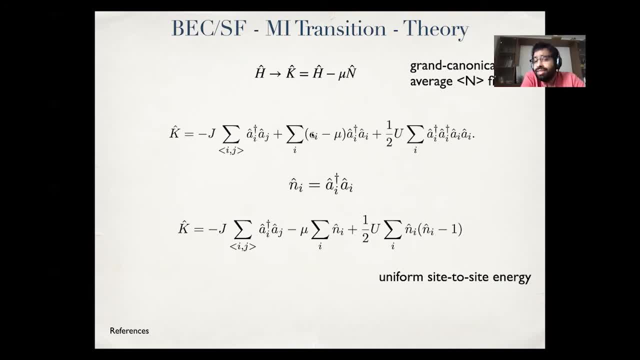 remove it. It's in constant addition And of course this is not exactly the case in experiments, but this is good enough for our understanding, our analysis. So this is our Hamiltonian, or I'm just going to call this the Hamiltonian. This is called the grand canonical potential, or grand. 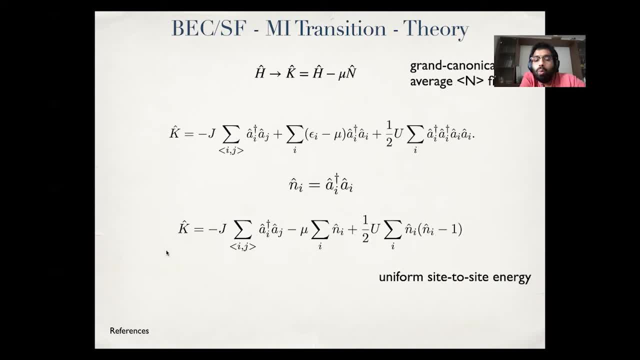 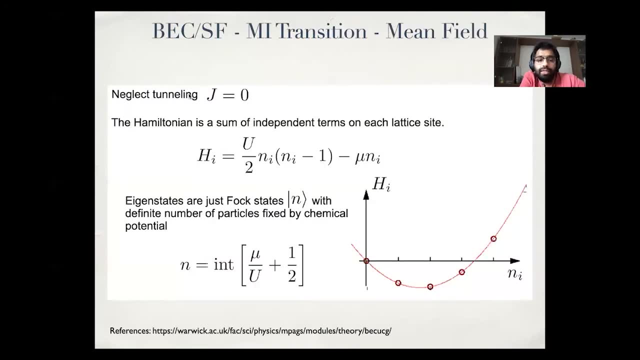 canonical Hamiltonian. And now we can analyze what happens to the ground state of this system as we tune u over j. Let us look at this extreme case: When I make j equal to zero, then this k becomes a sum of individual element, independent terms on each lattice site. And it is given precisely by this u over two ni. 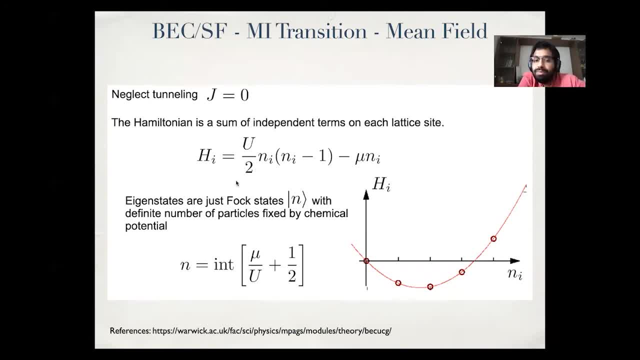 ni minus one minus mu ni. And now it becomes immediately clear that the eigenstates of this are basically Fock states with a fixed number n on each site. Then the value that your ground state takes is essentially fixed by the integer value of mu over u plus half. This n is precisely the number of particles in each. 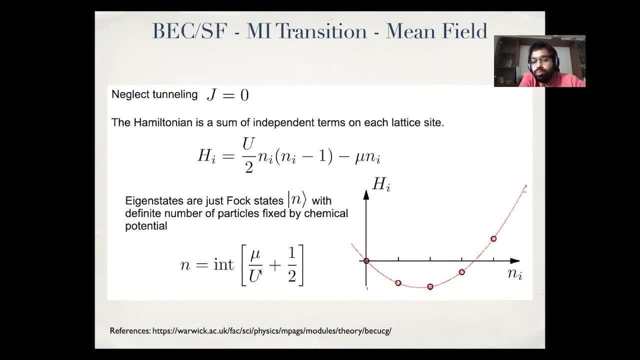 site is fixed by the value of the chemical potential to u. So that is my state in the j: equal to zero limit. This is just making the Fock state that I wrote down. I'm making a more concrete argument for it. OK, so now what we want to do is: now we have this qualitative suspicion that as I add this tunneling and the tunneling becomes larger and larger compared to u, I am going to lose this Fock state. 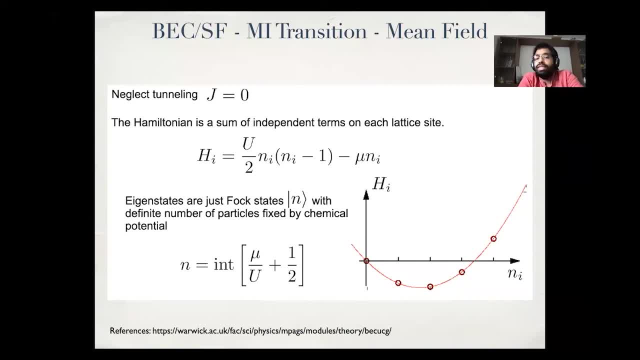 I'm going to go from this Fock state as my ground state to a superfluid state, And now all that. the only theory I'm going to discuss today is: how do you calculate the critical value at which I can go from this Fock state or? 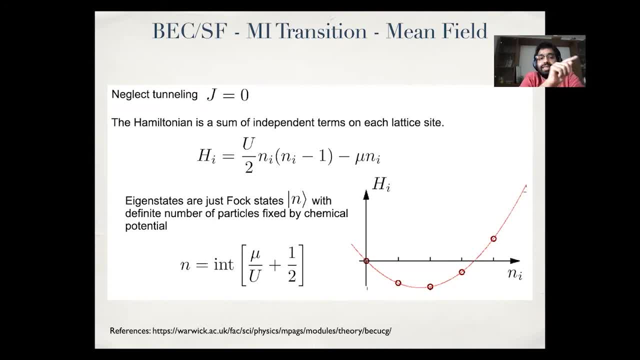 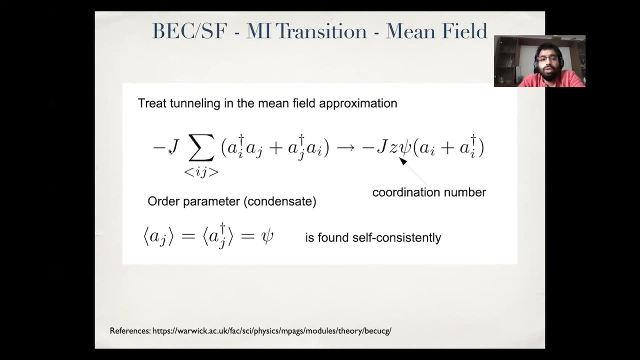 this Mott insulator state, with each site occupied with some Fock state to a superfluid. What is the critical value? How do you calculate? One method to calculate it. That's all we are going to do. So the way to do that is simple. It has two steps. The first step is the fact that I have to introduce this tunneling term. 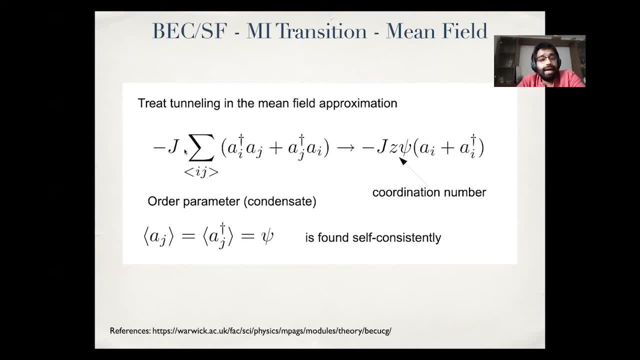 which has a i dagger a j, a j dagger a i. And I take this tunneling term and I want to introduce it as a mean field, as as as a perturbation, And I'm going to put up my energy eigenstates, which are Fock states, and calculate the new energy eigenstates under this perturbation from the tunneling. 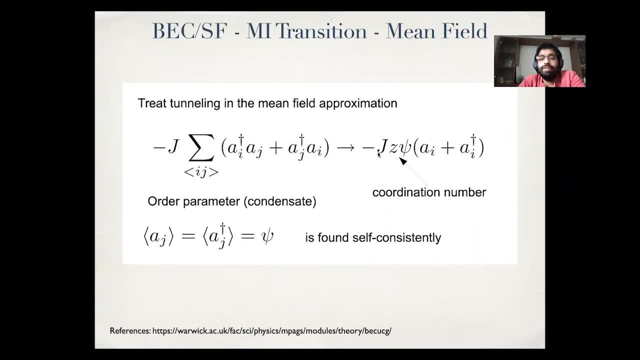 The second thing I want to do is I want to make a mean field ansatz for my perturbation, where I assume that this a, j, a, j, dagger, These have a finite amplitude. This finite amplitude is a feature Of having a superfluid state. you can see that immediately by going to what sort of state we have in the superfluid, in the superfluid. 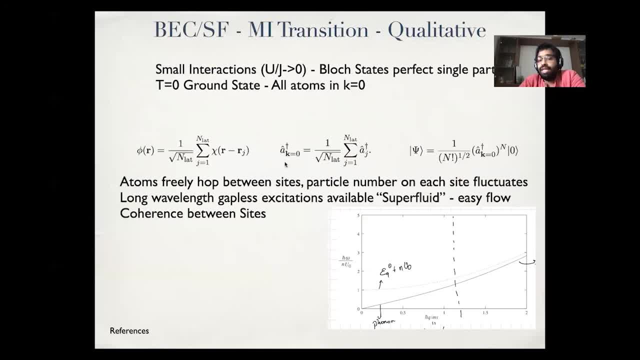 We have basically occupation of this k equal to zero state And if you look at the, the, the basically the, The condensate wave function that has amplitudes to be in different positions, different lattice sites. the amplitude on different lattice site is particular. 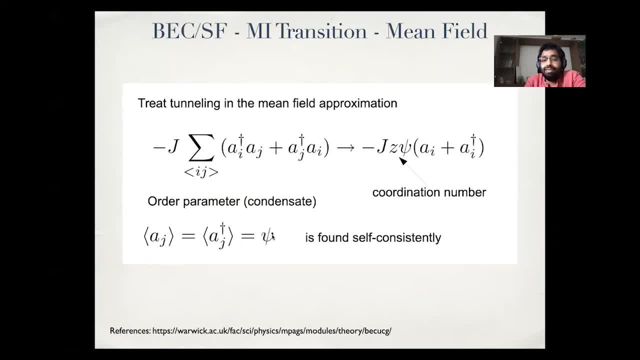 This is precisely this mean field parameter, psi, that we are taking. OK, And we are taking in the simplest sort of approximation, that it is the same mean field across different sites. OK, And now the idea is, once you do that, this tunneling term becomes very simple. 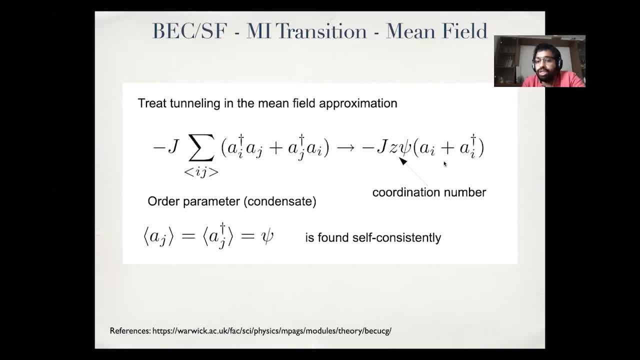 It becomes like an individual perturbation to each of the site. Each site has this Hamiltonian in terms of a i dagger, a i, And it has basically a perturbation given by this j z psi: a i plus a i dagger. And now we will find the value of this order parameter self consistently. 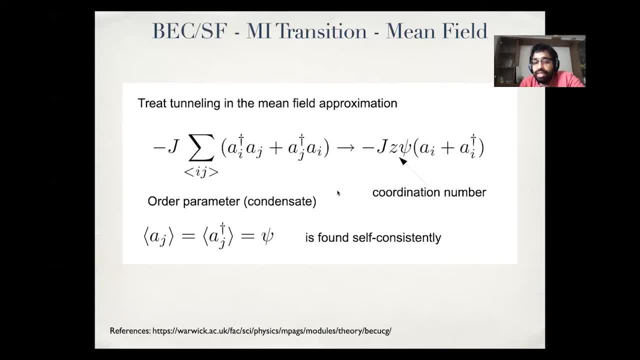 And, of course, a mod insulator is a scenario where this self consistent value for psi should be zero. Right, Because in that case I can completely ignore my tunneling. That is the fundamental idea. OK, So now let's just write down the expression for this perturbation theory. 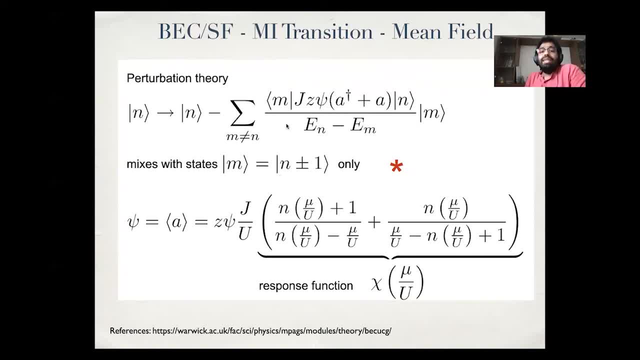 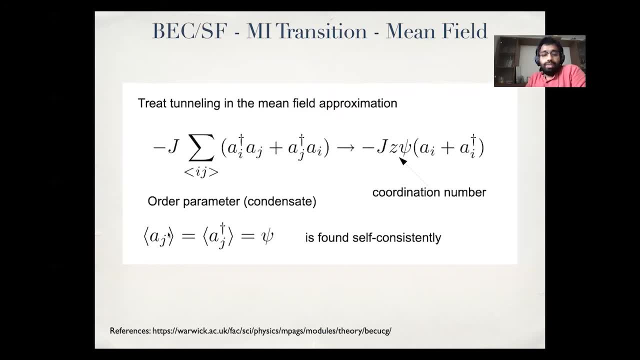 Very simple: first order perturbation theory for the state. And once I write down the perturb state, I can calculate the value of this A, i, which is my tunneling parameter, which is same in for all j, And I can calculate it. when I calculate that, very nicely. 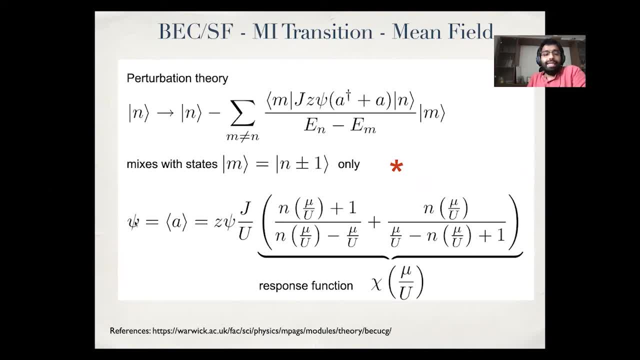 It brings me to this right hand side. So I get a self consistent equation that gives me psi equal to z, psi times this response function Chi, which depends just on the chemical potential and the interaction strength, And now I have my answer. So now the idea is that if I write this equation down, it has two solution. 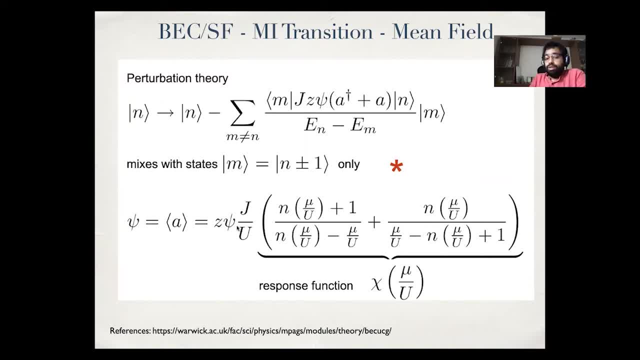 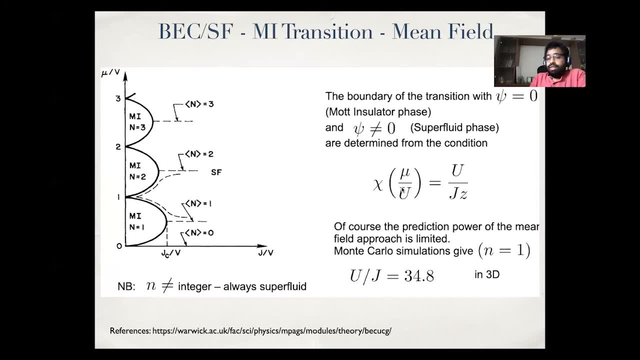 Either psi equals zero And this solution- psi equal to zero- is valid as long as this characteristic equation of this, chi equal to u or j z- has no solution. OK, As soon as this has a solution, there is a chance for psi not to be zero, which means I am going to go from a mod insulator to a superfluid. 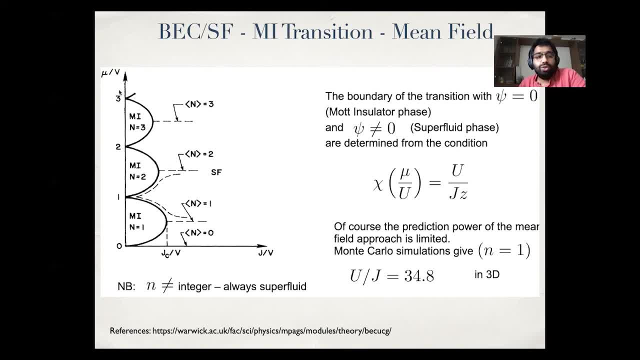 So I can basically state different values of mu and different values of j And different values of average n or, sorry, different values of n of the number of particles per site, And calculate at what point do I basically get a solution to this equation? 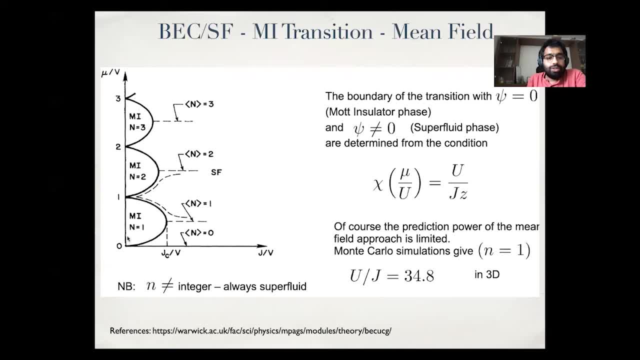 So, for example, here, I start here and I keep calculating, calculating. There is no solution, no solution, Boom, I find a solution. Then I have crossed from this mod insulator to a superfluid, And when I do that, I basically get this phase diagram with these lobes representing mod insulator states. 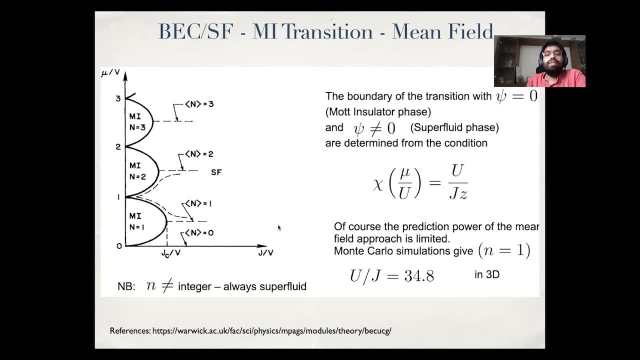 And outside the lobes having a superfluid, And from this you can predict at each value When do you get a. basically, for when do you get a transition from a mod insulator to a superfluid? For this zero case, the critical point is given by u over j. 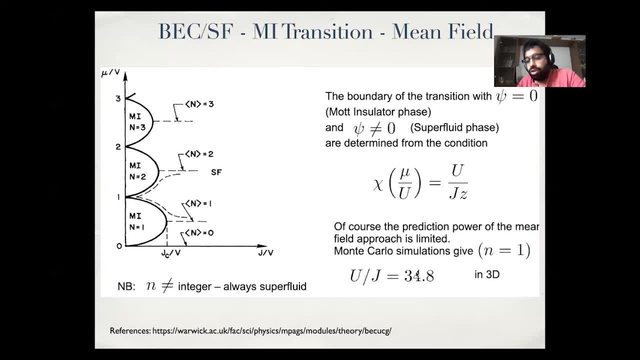 By the mean field theory, you get an answer which is not so close to this. But you can do a numerical simulations simulation and you can find the value, the exact value, But the mean field comes close, but it's not super close. 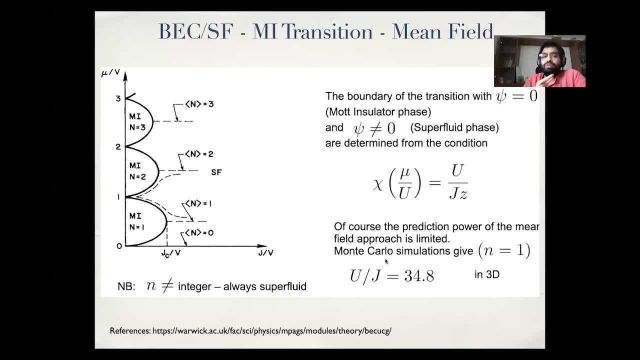 But this? this is just the basic sort of theoretical description of how you would go about talking about this BC, superfluid transition. But of course there are more and more sophisticated methods, including better numerical methods. Even theoretical methods are there which unfortunately, due to the lack of time, I cannot talk about. 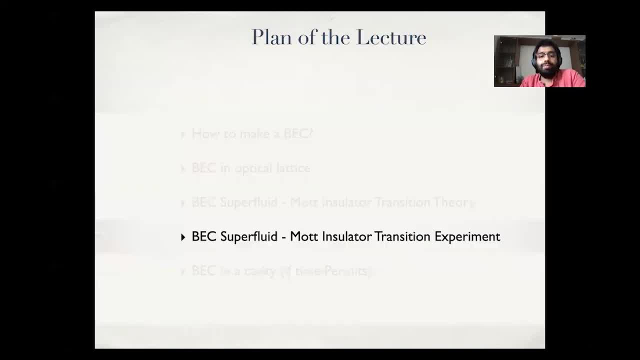 But that's just to give a rough idea of what happens in this transition. Now let me finish this part by looking at the experimental observation of this superfluid mod insulator transition, which is one of the landmark achievements in ultracold atoms. 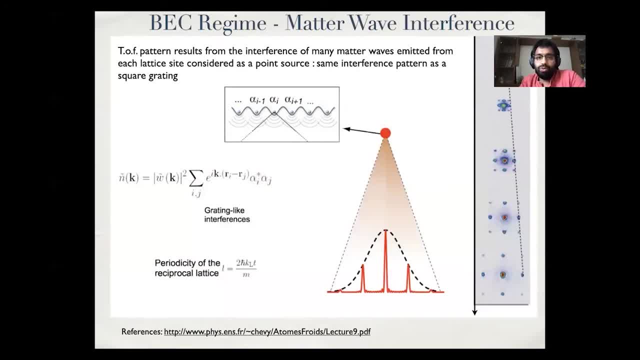 So again, I'm going to be very- it's just a very overview of it. So the idea is, as with all of these ultracold atomic experiments, how do you do this experiment? You load your atoms into this optical trap. What does that mean? 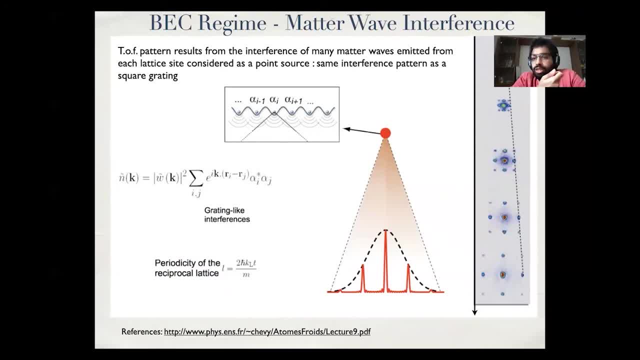 You take your magnetic trap and then you switch on this periodic potential. As you switch it on, you switch it on to certain lattice depth. So when you switch it on to a certain lattice depth and you allow the atoms to go to their ground state, 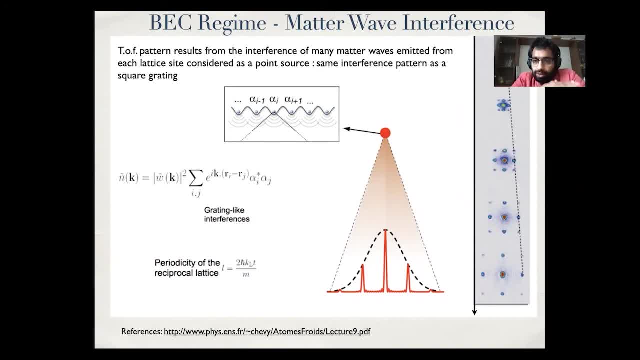 and then, once their atoms have gone and gone to the ground state, in this many body set up in this applied potential, applied optical lattice potential, you turn off the optical lattice and you let the atoms expand and you look at the density distribution. Now, for various reasons, 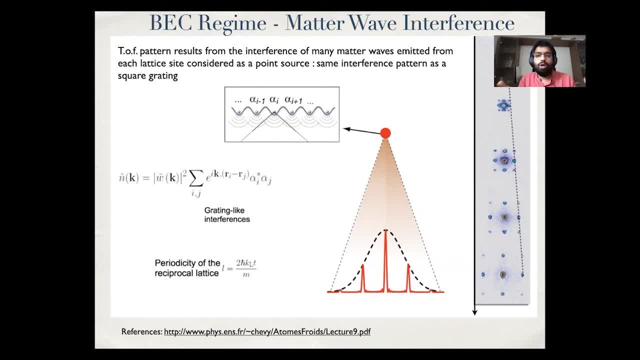 very small lattice depths if you're ramped up to, let's say, small lattice depths, in which case you expect a BEC or a superfluid. What happens is that when you look at the density distribution after time of flight, it has very clear peaks at k values given by pi over d. 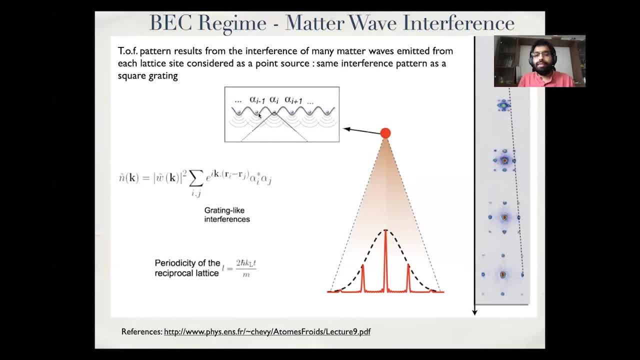 Or in other words, in this case the different atoms in the different wells are acting as though they are coherent sources of waves, and their interference between them comes out very nicely in the density distribution. The other way of looking at this is to also imagine that if I am in the block wave, 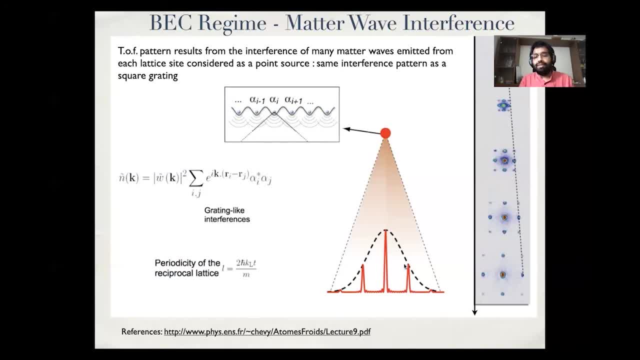 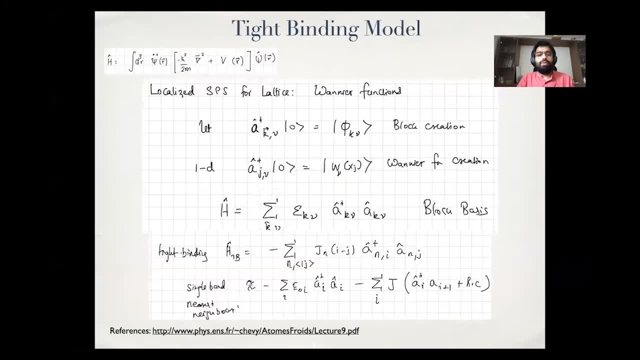 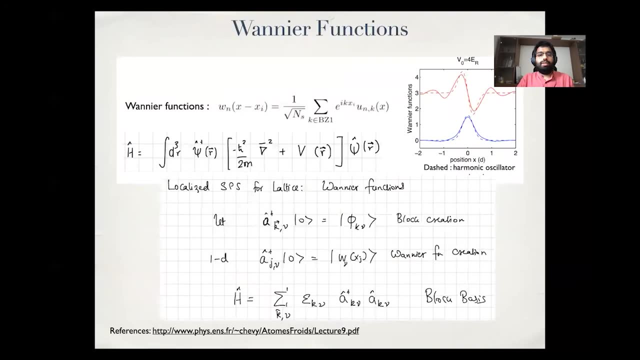 I have essentially a block wave which has peaks at different k. So if I expand my block wave solution that I wrote down here, Let me go here. Yeah, So if I take this UK nu and if I actually expand it in a Fourier series, 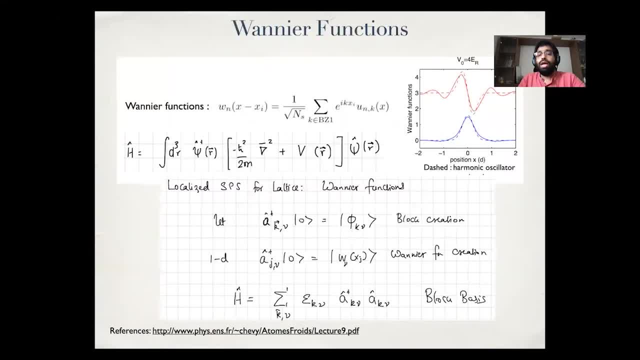 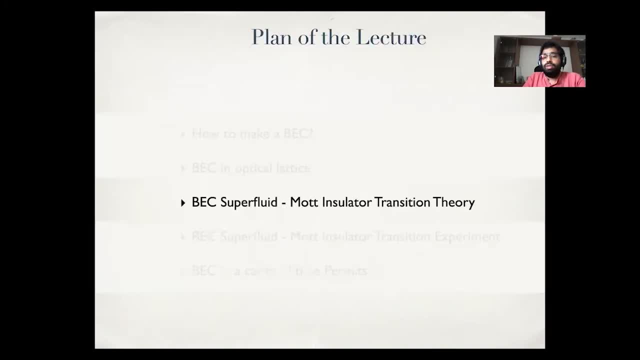 I will have amplitudes at different k values And my density distribution in my lattice is precisely going to have peaks at those k values, Right? So if I had a block wave function, if my BC boson sine condensate is in a block wave function, 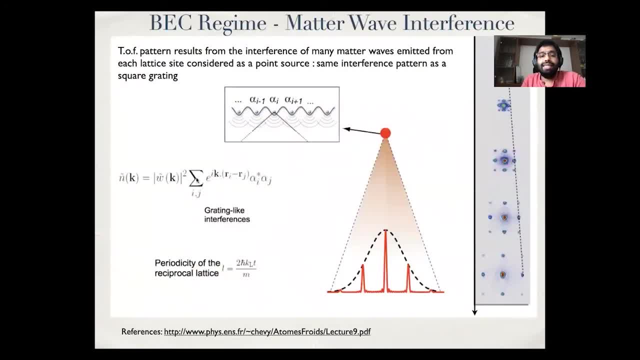 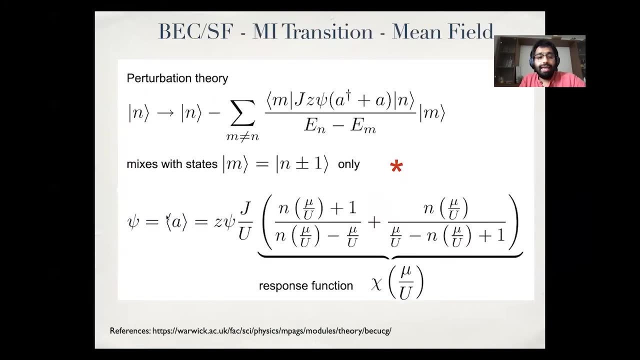 I better expect this interference pattern. And this interference pattern also arises from this idea that this individual Ai's averages are actually finite and they are given by this psi that we wrote down. So this A has to be finite in order for this interference pattern to happen. 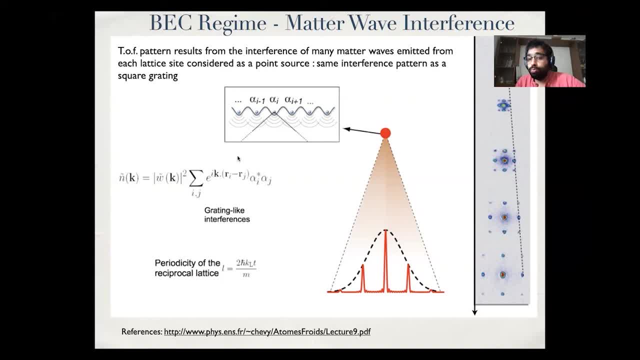 So this is basically the Fourier transform of the BEC wave function in all of the atoms in the ground state of ground, in the k equal to zero block state, for instance, And of course this is basically Ai dagger Aj's average. So you need correlations between different coherence or correlation between different sites to exist. 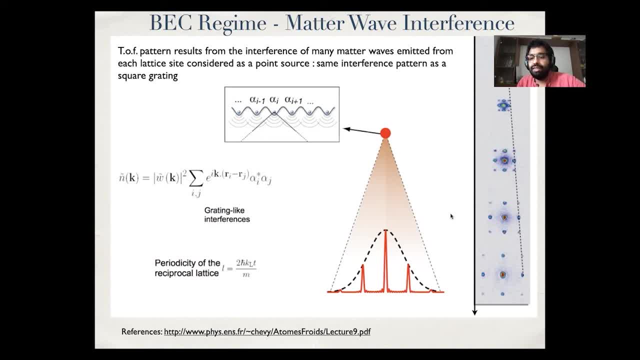 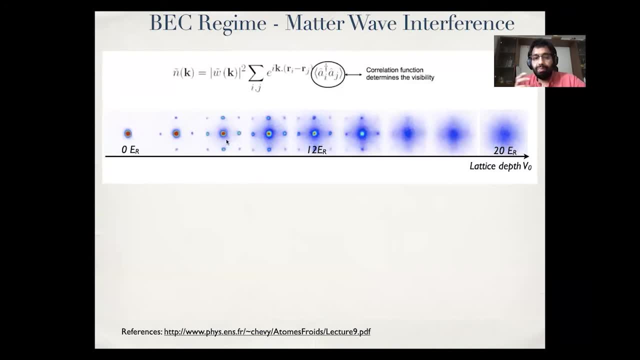 If that is not there, you do not get this interference pattern. So what happens is, as you keep increasing the lattice depth to which you ramped, you see, after a point this interference pattern completely goes away When your lattice depth is very large. 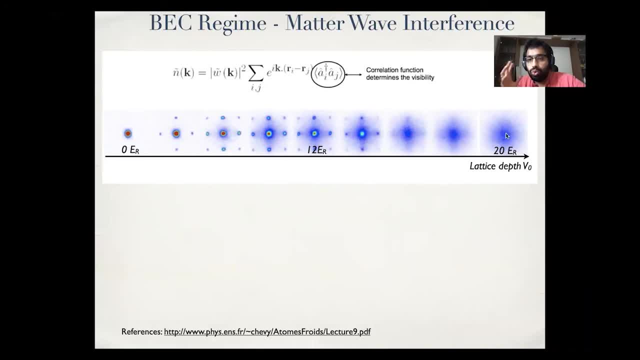 you have reached this lattice depth, You have reached this limit where your U over J is very large, Your J has become extremely small and the interactions have won as the highest time scale And at this point you have an insulating state, And this is the evidence of the insulating state is in this time of light absorption image. 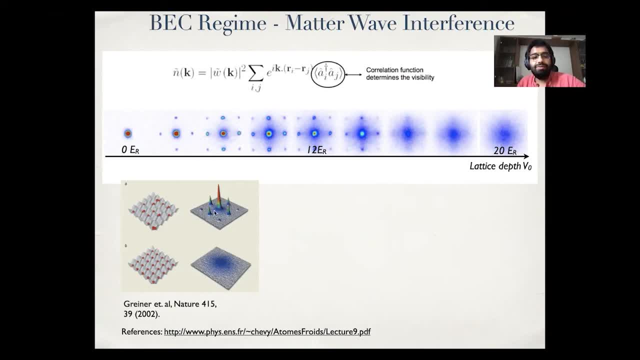 For the superfluid you get a very nice peak structure like here, And for the Mott insulator you get this completely diffused state where there is no peaks. That was in 2002.. Things have become even more cooler now. 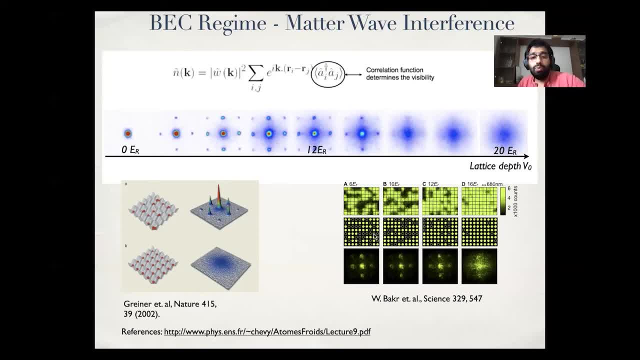 This is a recent experiment around 2010, where you can actually make one of these Mott insulators and not study the momentum distribution, but use what's called a quantum gas microscope, which is a very high resolution imaging system of an optical lattice. 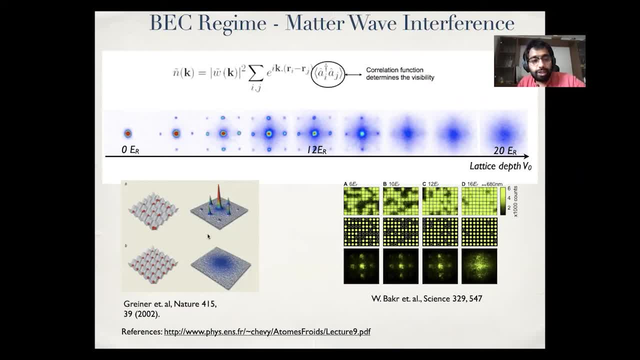 And literally look at the fact that you really have a single atom at each site. Each dot here Is basically one lattice site of my optical, of my optical lattice at lower lattice, lower lattice sites. When I take a picture of my optical lattice I get some distribution. 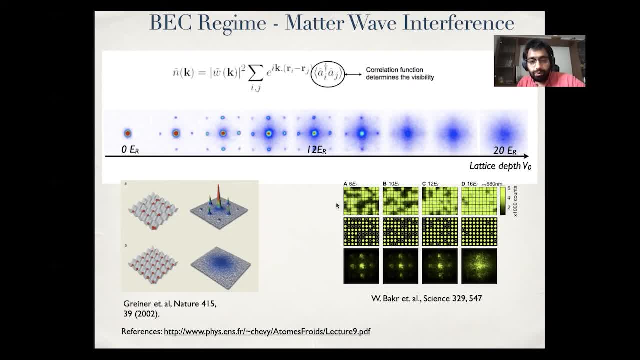 And if I keep taking pictures at one time after another time, I will see the atoms moving around a lot. On the other hand, once I get to this extremely large lattice depth, I get this Mott insulator where at different times, if I keep taking pictures. 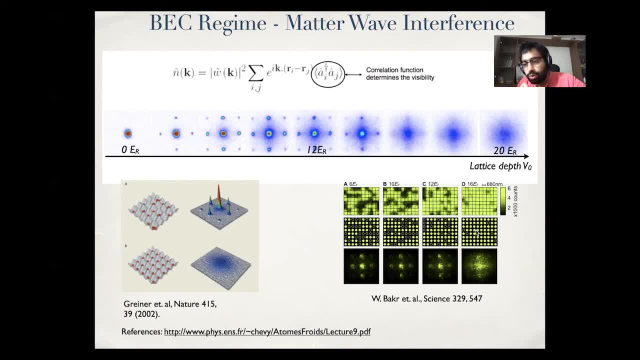 there is perfect unit filling and I can really count these atoms and I can really image the atoms in a Mott insulator. So this is literally one of the coolest pictures that you can find of a many body system, where I can take a many body system and take a snapshot of its individual components. 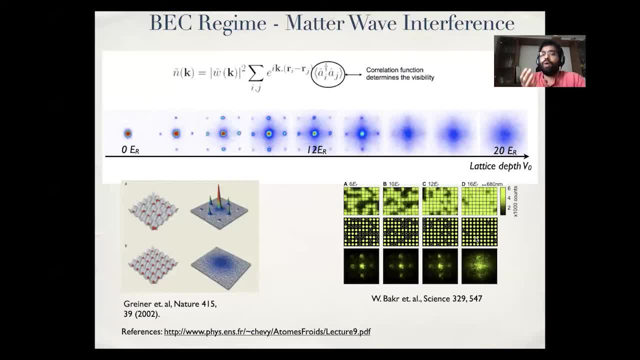 which can completely change the sort of questions you can ask of this many body states. You don't have to ask average questions anymore. You can ask very beautiful questions. And this is again. Again, it is by the same person: Marcus Greiner. 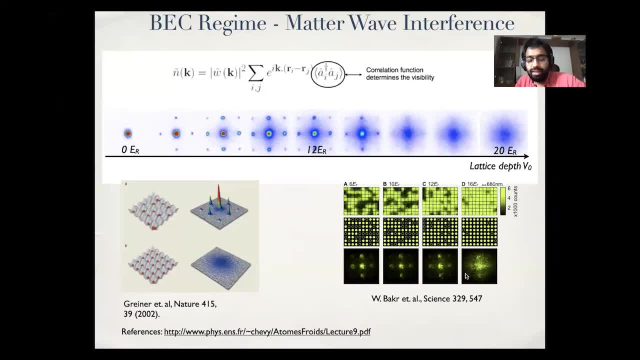 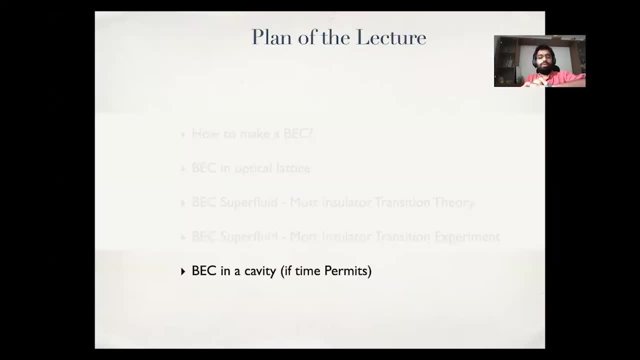 He was a student here and this is from his group now in, I forget, MIT or somewhere else. So that's that's where we are with this Mott insulator, superfluid transition. So now the time is, I have about 20 minutes. I'll stop here and take some questions. 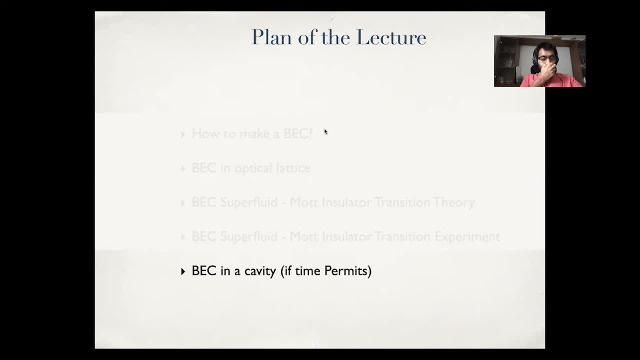 It would be nice If you can also unmute and ask the question. Let me see while I'm looking at the chart. Does anyone want to unmute? Okay, So if not, let me just read the questions. So one question in Mott insulators. 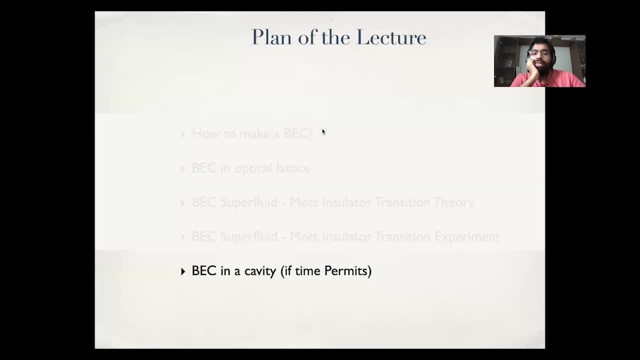 I have come across something like spin liquids, where the spin of the electron flows, leaving behind its charge. How does it make sense? Okay, So this is somewhat of a more exotic phenomena. This is called spin charge separation. I'm not an expert on this. 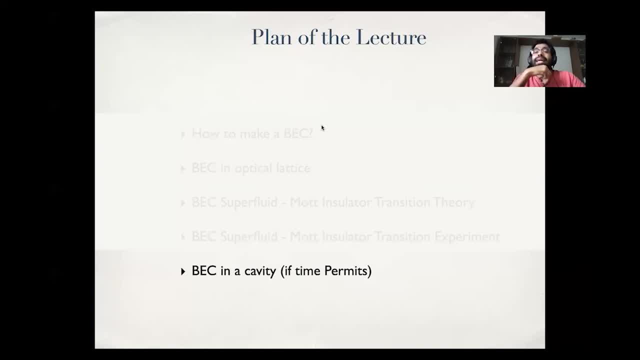 Let me just say what I know of it. in some electronic systems- strongly correlated electronic systems- in order to describe certain counterintuitive bulk properties, For example, I'll have like a situation where my magnetic probe will tell me I have, let's say, 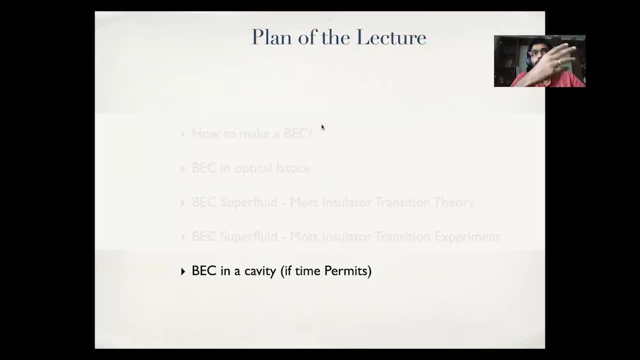 a particular kind of ordering, in which case I do not expect, you know, thermal transport to be significant due to the spins. But on the other hand, when I do a transport measurement I will see transport. Then one is somewhat flummoxed and asks: exactly how can this happen? 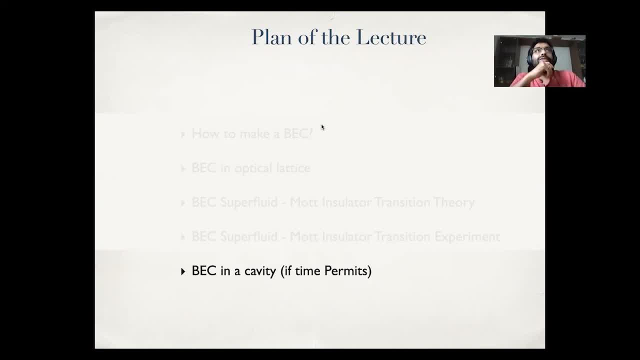 That I have a many body state of my degrees of freedom, where it looks like the degrees of freedom are frozen, But certain aspect of the degree of degrees of freedom seems to be still doing some conduction. Okay, So then, if the frozen aspect of the degree of freedom is, it's a spin. 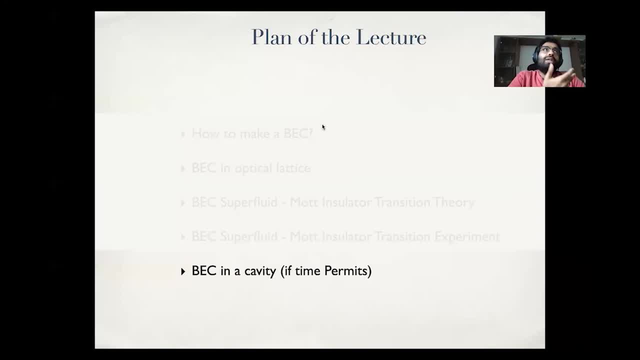 whereas the transport is done, it's charge. then one can imagine that the actual degrees of freedom, the emergent degrees of freedom of my many body interacting system, is not the original system with electrons with attached spins, But these are some strange quasi particles where I can actually uncouple the spin and be charged and they can flow independent of each other. 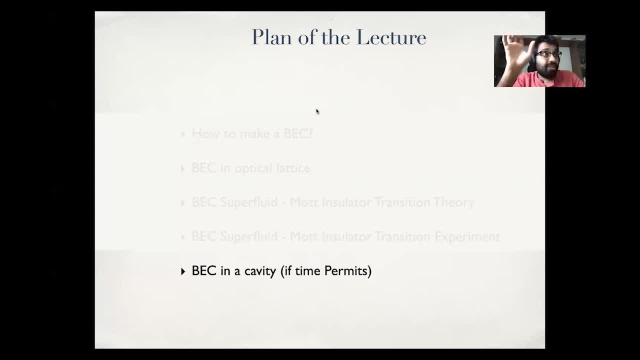 So this is rather exotic And this is sort of a popular science level explanation, And I am, I have also not done computations of such things, So I can't say much more than this popular science picture. This can happen in certain strongly correlated systems. 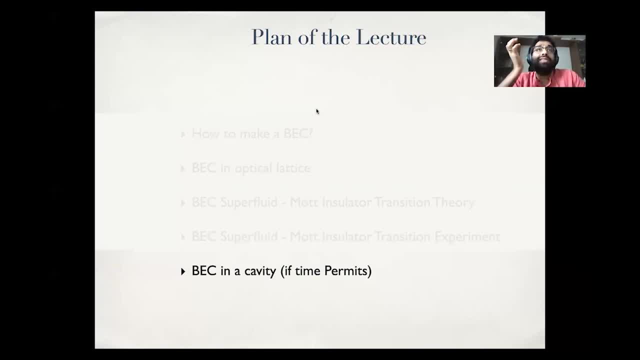 But to my knowledge in an ultra cold atomic system this has not been shown yet. Spin charge separation effectively has not been shown. In fact, magnetism with ultra cold systems is a slightly hard topic in itself. Okay, Aditya is asking. 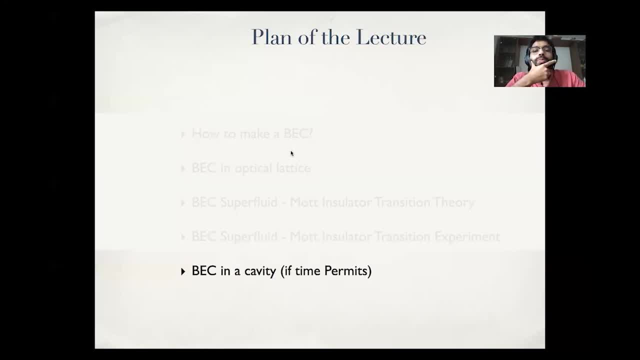 can you once again give the explanation of the superfluid distribution, The definition that you described as a BEC that flows? would that still be considered a Bose-Einstein condensate? Okay, I so. so let let me say what I'm saying. 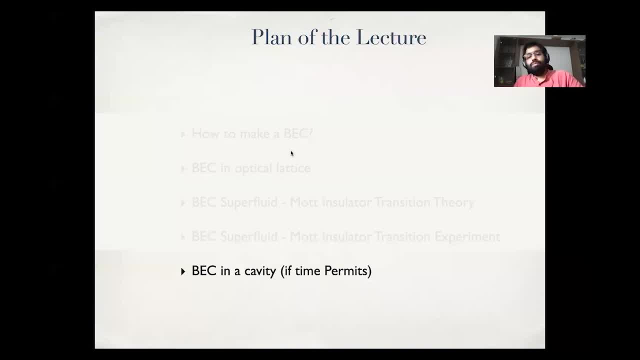 So what I'm saying is that? let me correct. maybe the way I said caused confusion more than clearing up confusion. Now, what I was saying is that super fluidity can be understood as one property of a interacting Bose-Einstein condensate. 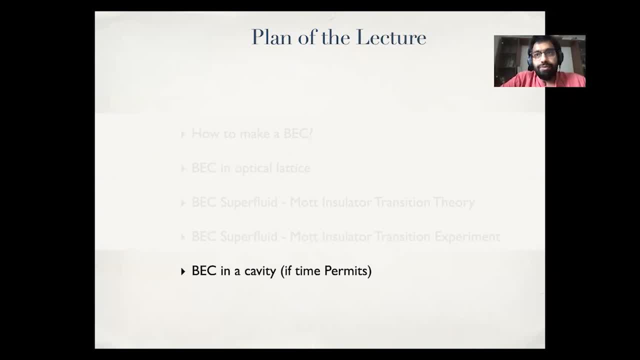 And the idea is that, basically, if you, if you somehow managed to put a Bose-Einstein condensate in an in one of these capillaries, now the capillary will also, of course, have to be made by some light induced potential. 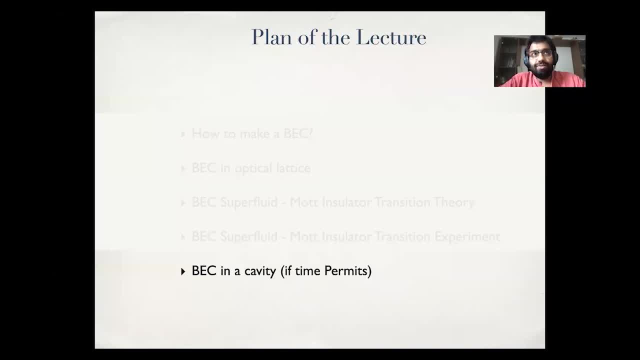 Then you will get frictionless flow at the velocity that is precisely given by the gradient of the face of the BEC wave function. This is one way of understanding super fluidity and the connection to Bose-Einstein condensation. The second way of understanding it is from the excitation spectrum. 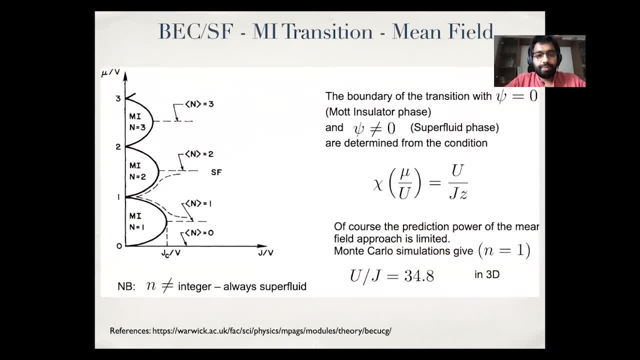 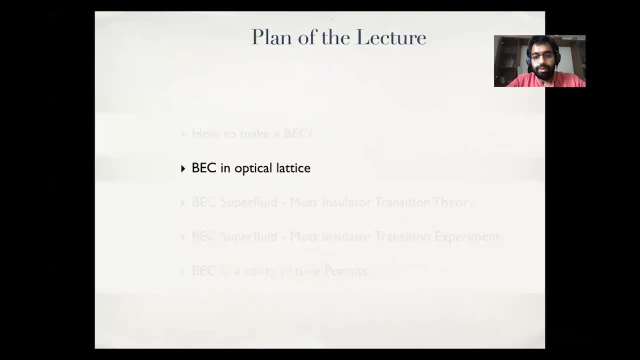 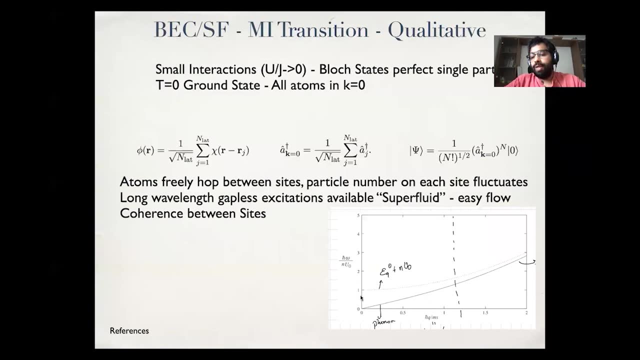 The basic point I was trying to make is the following: If we go to the excitation spectrum, where was it So? this is the excitation spectrum of a Bose-Einstein condensate We found by solving this Bogle-Libov equations. 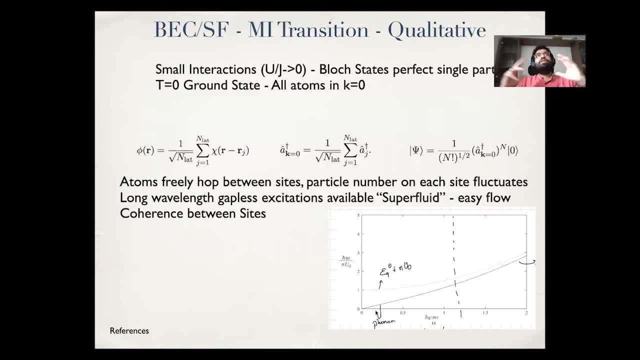 right. So now the idea is: if you think of like, like, how, super fluidity, let's say, from the helium base, how, how do people understand it conceptually, Conceptually, what is happening is somehow my atoms of my helium fluid at very low. 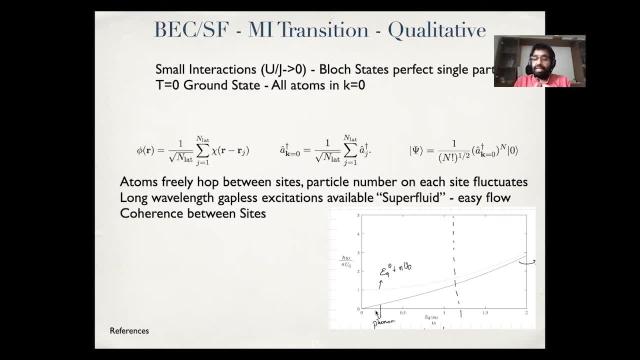 temperatures. when I put it in a real capillary, they are able to flow without friction because somehow they go into a very interesting quantum state involving many of the atoms, a collective state that somehow can screen the impurities that are present on the capillary wall. 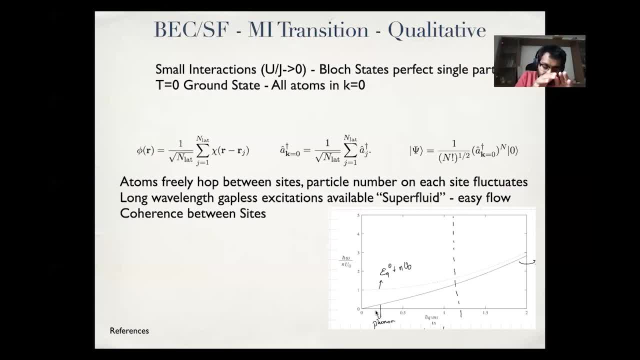 The capillary wall will cause some friction, but I'm able to screen this friction because it is not individual atoms that are actually moving. If individual atoms are moving, they would scatter off the wall and basically give me friction. That is the microscopic picture of friction. 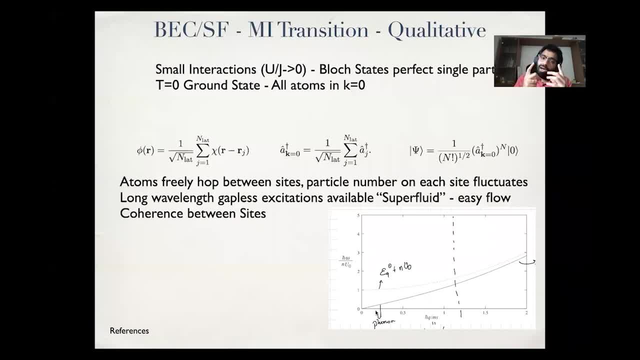 That would come, but that is not happening. But somehow these atoms are collectively becoming into some very strange quantum state, which we know, at least, as partly coming from having a Bose Einstein condensate now, which allows me to flow without resistance. Okay. 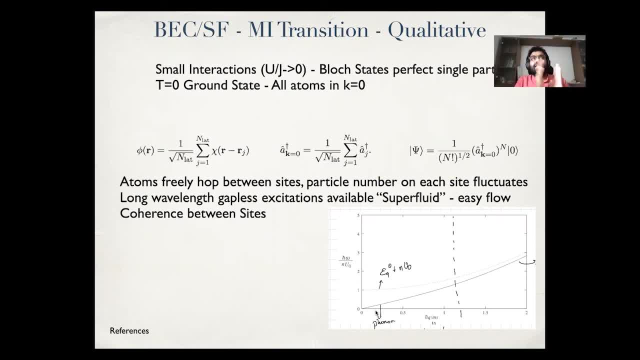 So this picture of super fluidity tells us that if you want a super fluid, you, when you, when you excite your system, your system should be able to respond collectively. Okay, And if you remember yesterday, when we looked at this phonon excitation, 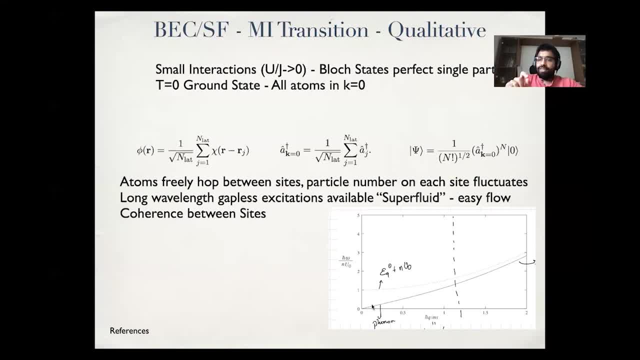 it precisely was an excitation of that nature, because in this long wavelength I'm actually involving a large part of my cloud, which means many of my atoms are participating, Or, in other words, these are collective modes, right, And of course, 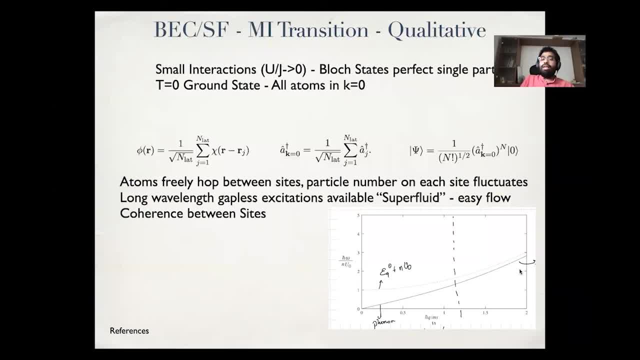 once I look at very small wavelength or very large wave number, of course I pick up my. my spectrum actually becomes EQ zero plus NU naught, which is a gap spectrum, right? So I need an minimum energy that is like single particle excitations. 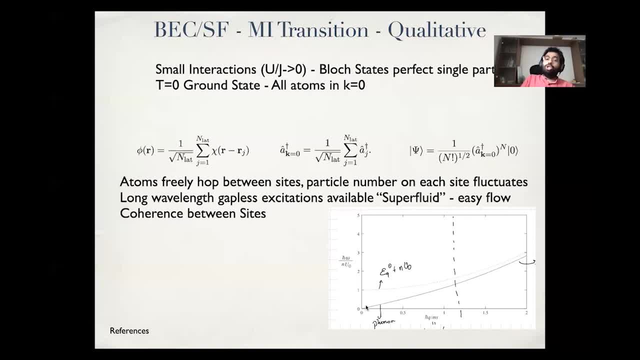 So the possibility that I can have such long wavelength excitations as the low energy behavior with with this dispersion that is going as K, that feature of my Bose Einstein condensate is again in line with the idea that the flow properties of my Bose Einstein condensate will be. 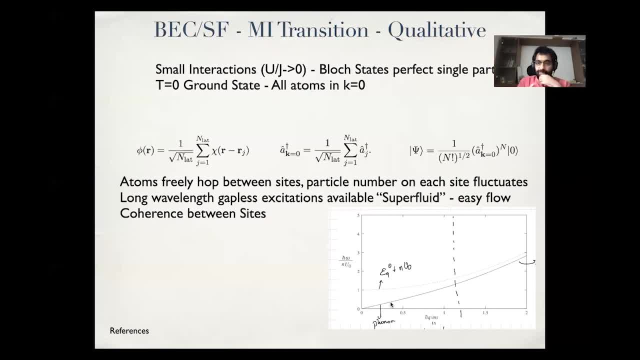 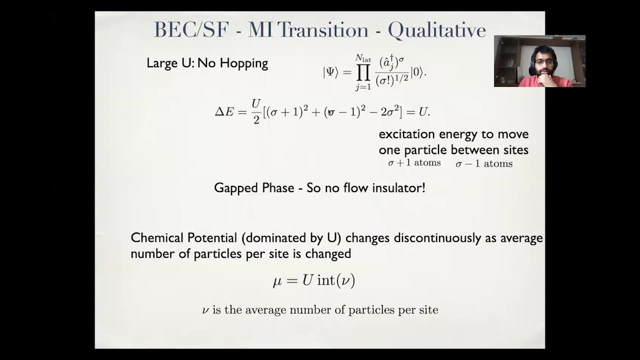 superfluid. I don't know if I answered your question, but I hope let's see You want to say something. Whoever asked the question? Okay, All right, So what is the time? We are almost Okay, Let me. 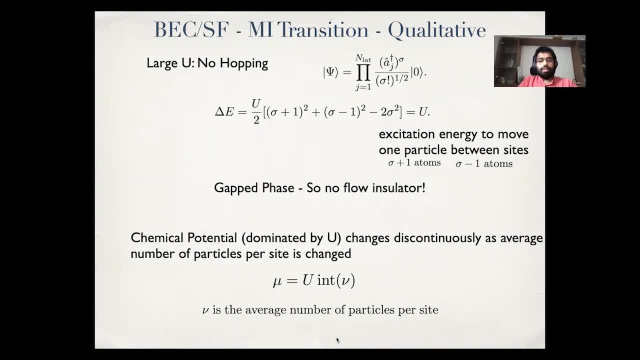 I can't see the time on my screen. You've got my watch? Oh, there is only 10 minutes. So then, let me, let me not go into this cavity. QED and Bose Einstein condensate part, because I think that is a. 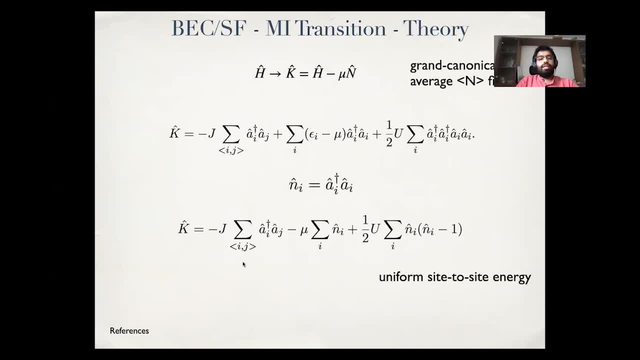 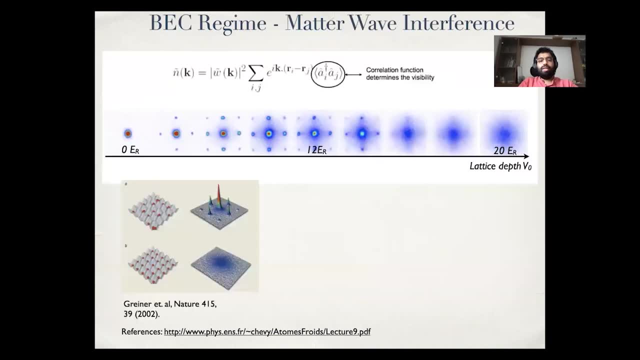 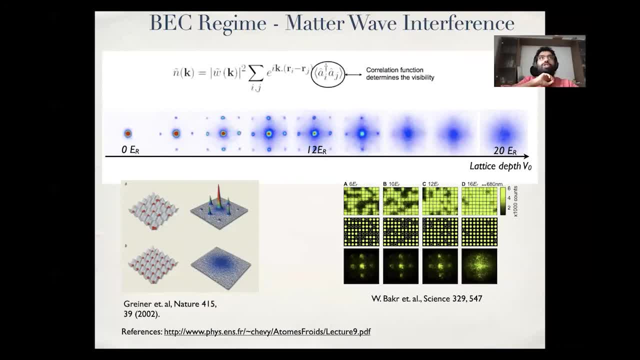 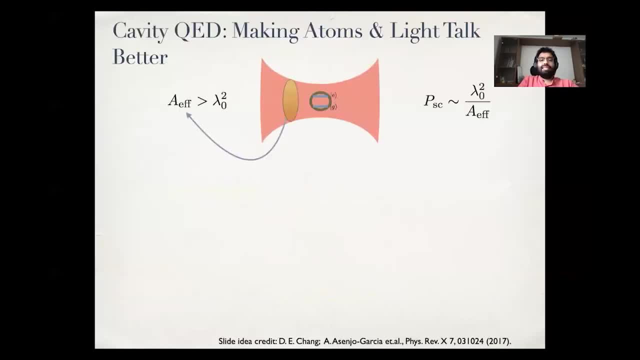 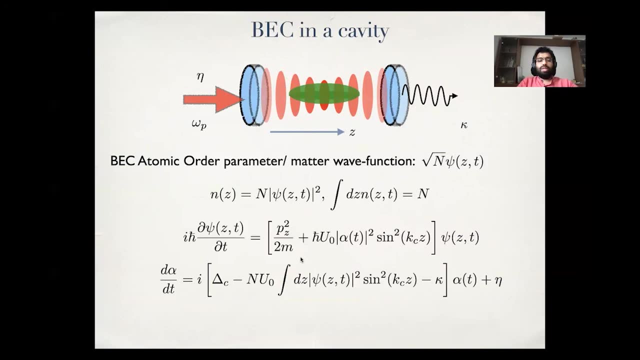 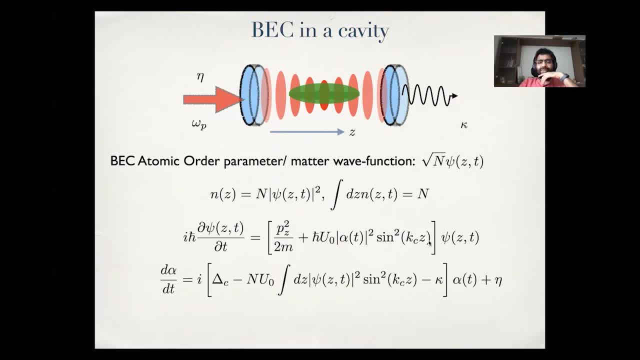 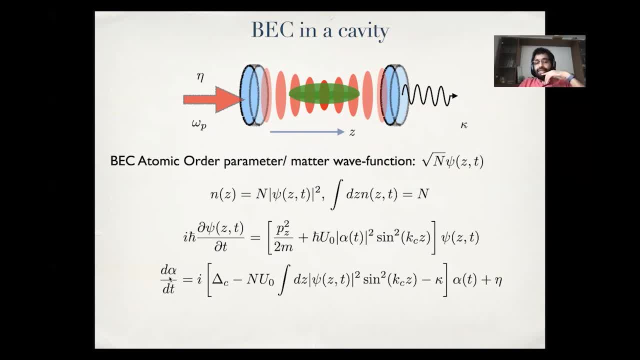 is not a given static number but really that actually also evolves with time. and it evolves with time base because my atomic degree of freedom, so my boson stand- condensate wave function, that can actually be a function of time. i can have some dynamics here. if i move my cloud that changes my 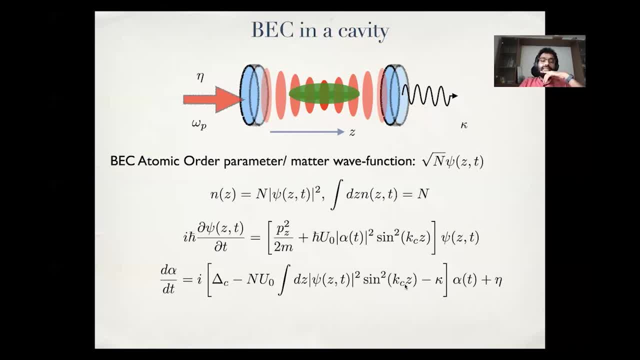 alpha and i can get some dynamics. so this means that the light induced potential that is inside a cavity is somewhat more exotic than the regular optical lattice because it allows for the atoms not just to move in some fixed potential but the atoms can back act on the potential. 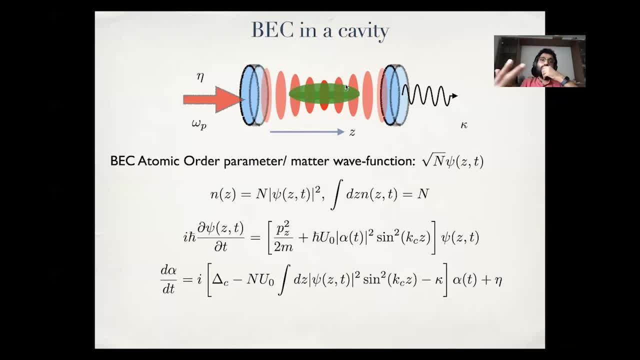 actually, and this is beautiful because this does two things. one is it leads to rich many body phenomenon and condensed matter phenomenon, because this is somewhat closer to what happens with electrons in a solid, for example, the. the most famous example of this is superconductivity, which you cannot have. 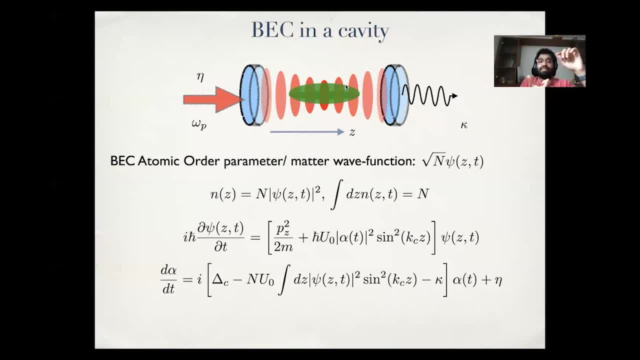 unless there can be electron phonon interactions. phonons are the lattice, so there is an. the electrons actually back act on the phonons of your metallic lattice to get a superconductivity state. so this possibility of the degrees of freedom, like our atoms, to influence the potential. 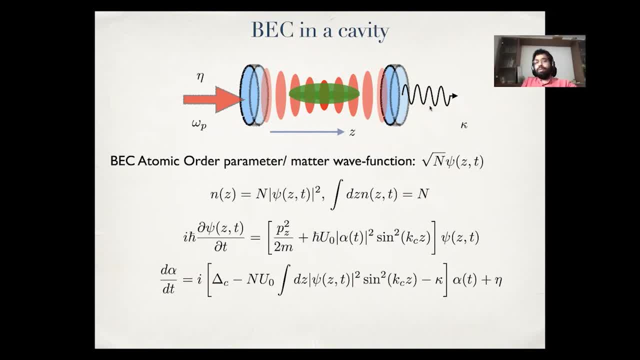 in which they are moving will lead to interesting physics that way. the second beautiful thing that can happen is because the light inside the cavity eventually leaves the cavity. i can actually use that as a beautiful non-destructive probe of the atomic dynamics and this way i can actually see. quantum phase transitions in real time, which has been done, or i can also感覺 that in the middle. yeah, i feel like i can. fundamentally, Pf Sensandra was actually able n't to change, but just because you can actually change it and, if you want, certainly can do this thinking now. 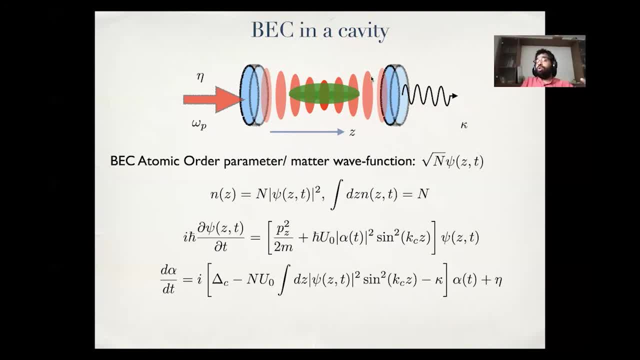 in real time, which has been done, or I can also use this as a sensor. For example, if I can use the atoms to sense a force, I can read out the force from the light of the cavity. So these two features that you get truly interesting, coupled dynamics between light and atoms, as well as you. 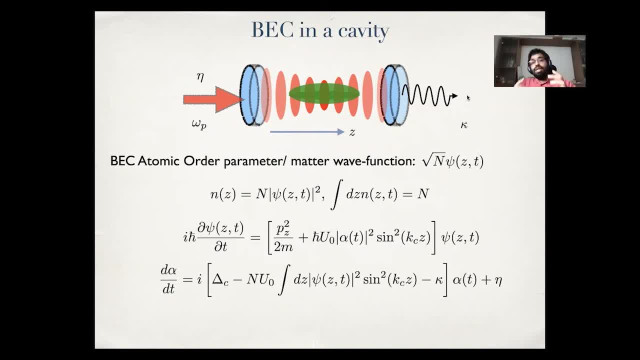 can use light as a probe to study the atoms. these two things make the study of Bose-Einstein condensates in a cavity. a very interesting field with many interesting open questions and many interesting follow-up questions, some of which I'm among others I'm looking at, like many people. 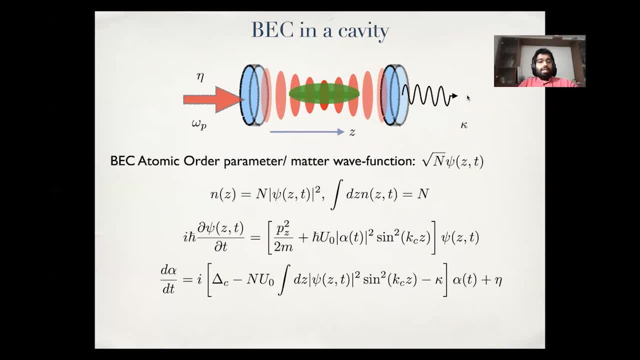 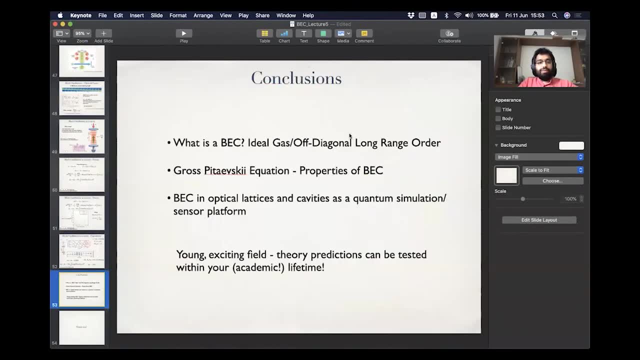 I'm looking at that as part of my research. okay, So let me quickly go to the conclusion slide and conclude. and we can have- there are more questions, we can have discussion. So we've managed over the last five days to understand, or at least partly understand. 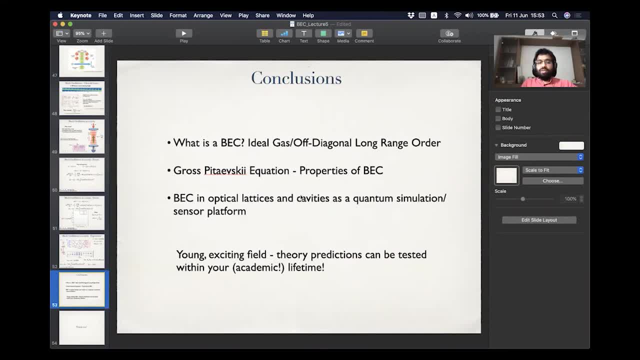 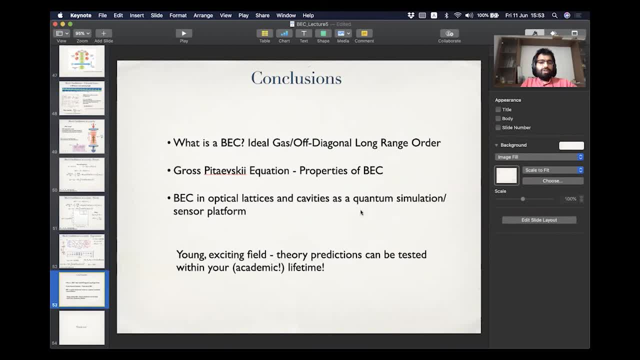 simulation and sensor problem. This last part I did not really talk in detail about, Just I hope I was at least able to convince you that this is a young and exciting field. in some sense It's only like about 20 years old and the theory predictions can be tested within your